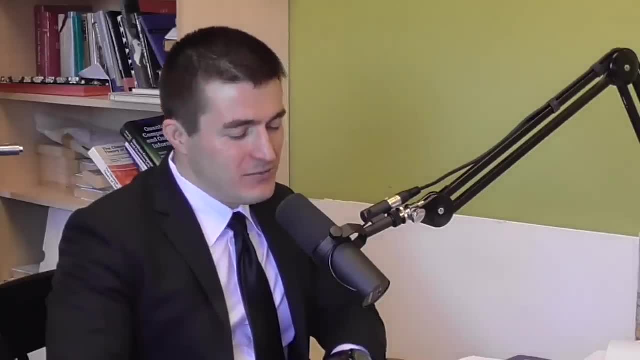 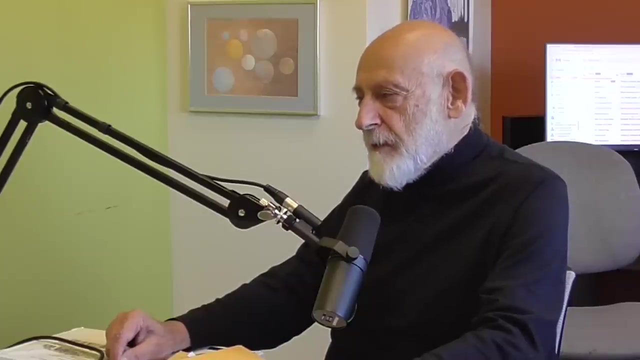 or black holes, or string theory, using intuition as a first step or a step throughout, using visualization? Yeah, very much so, very much so. I tend not to think about the equations, I tend not to think about the symbols. I tend to try to visualize the phenomena themselves. 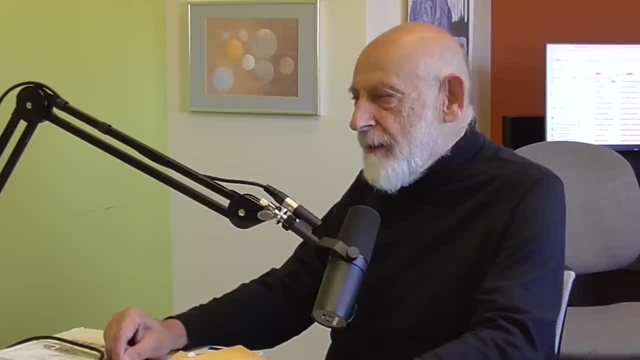 And then, when I get an insight that I think is valid, I might try to convert it to mathematics, But I'm not a natural mathematician. I'm good enough at it. I'm good enough at it, but I'm not a great mathematician. 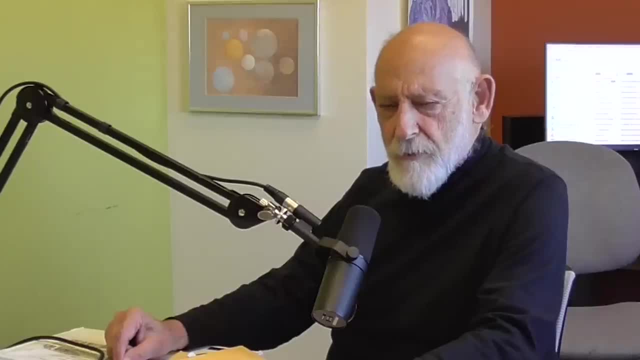 So for me, the way of thinking about physics is first intuitive, first visualization, scribble a few equations maybe, but then try to convert it to mathematics. The experience is that other people are better at converting it to mathematics than I am. 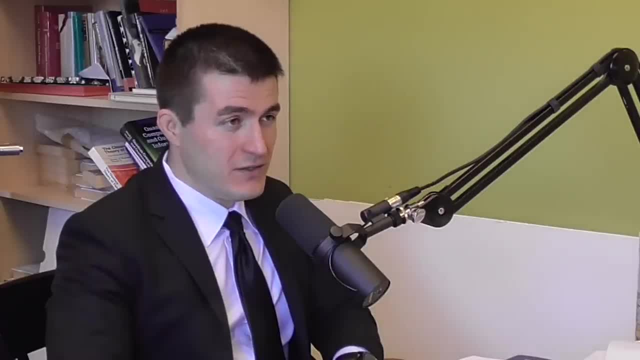 And yet you've worked with very counterintuitive ideas. No, that's true, that's true. So how do you visualize something counterintuitive? How do you dare? By rewiring your brain in new ways? Yeah, quantum mechanics is not intuitive. 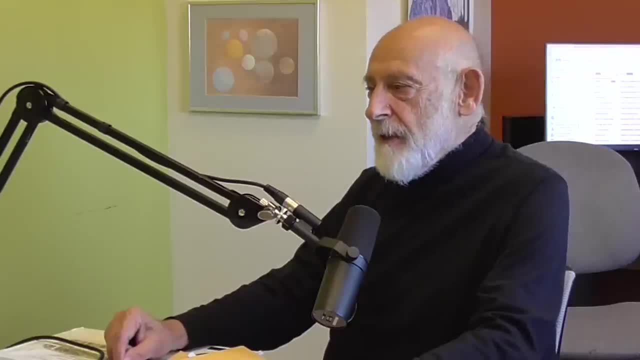 Very little of modern physics is intuitive, Intuitive. well, what does intuitive mean? It means the ability to think about it with basic classical physics, the physics that we evolved with throwing stones, splashing water, whatever it happens to be. 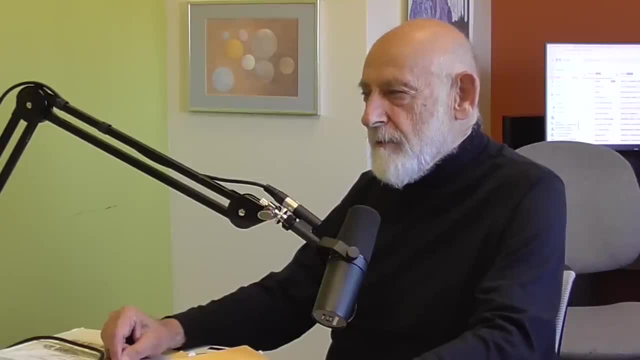 Quantum physics, general relativity, quantum field theory are deeply unintuitive in that way. But you know, after time and getting familiar with these things, you develop new intuitions. I always said you rewire. And it's to the point where me and many of my friends 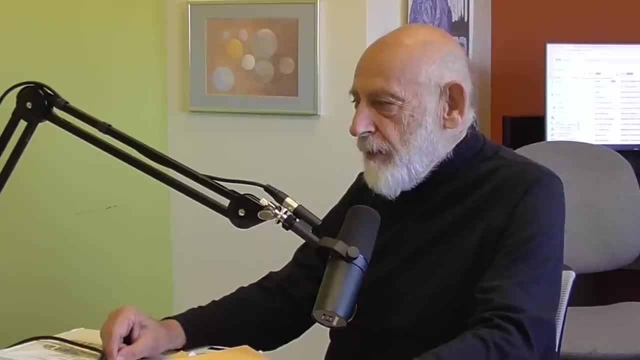 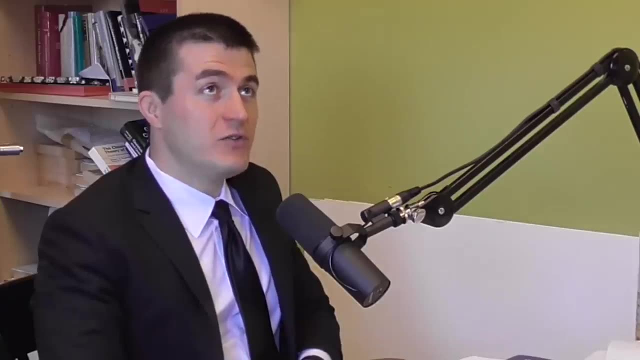 I and many of my friends can think more easily quantum mechanically than we can classically. We've gotten so used to it. I mean, yes, our neural wiring in our brain is such that we understand rocks and stones and water and so on. 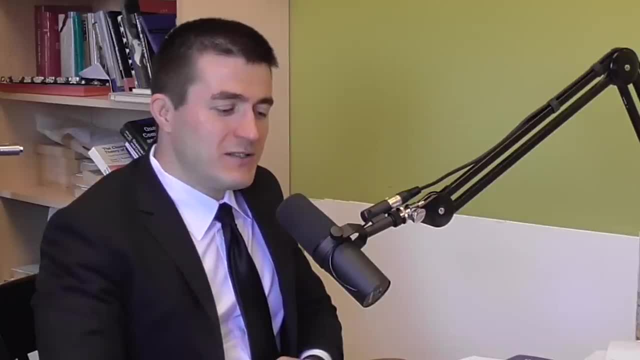 We sort of evolved for that, Evolved for it. Yeah, Do you think it's possible to create a wiring of neuron-like state devices that more naturally understand quantum mechanics, understand wave function, understand these weird things? Well, I'm not sure. 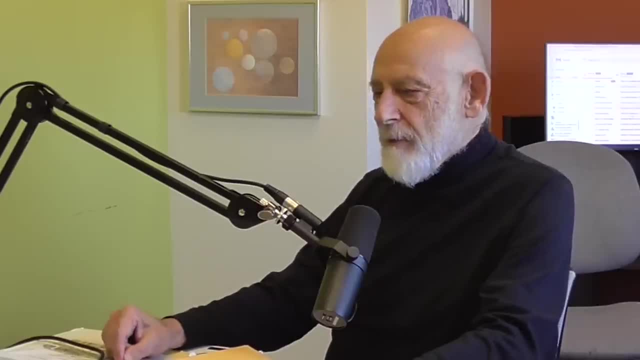 I think many of us have evolved the ability to think quantum mechanically to some extent, But that doesn't mean you can think like an electron. That doesn't mean. another example: Forget for a minute quantum mechanics, Just visualizing four-dimensional space, or five-dimensional space, or six-dimensional space. 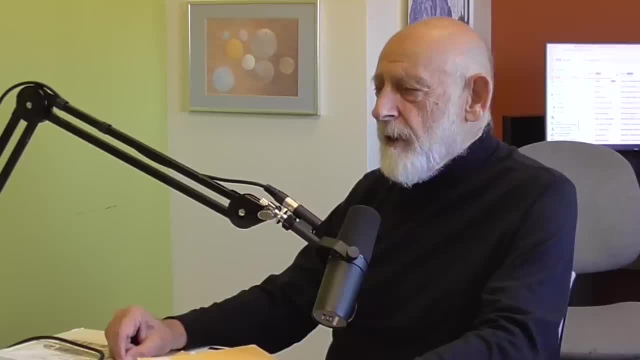 I think we're fundamentally wired to visualize three dimensions. I can't even visualize two dimensions or one dimension without thinking about it as embedded in three dimensions. Right, If I want to visualize a line, I think of the line as being a line in three dimensions. 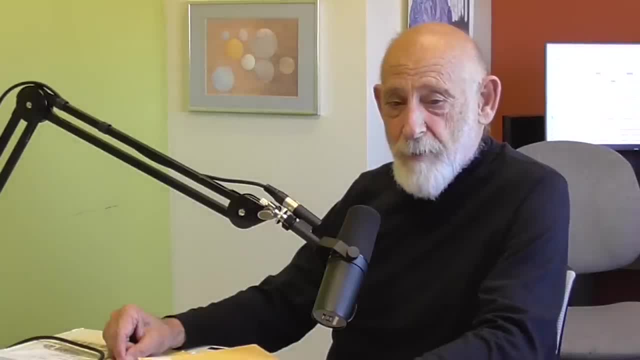 Right? Or I think of it as a line in three dimensions, Right? Or I think of the line as being a line on a piece of paper, with a piece of paper being in three dimensions. I never seem to be able to- in some abstract and pure way. 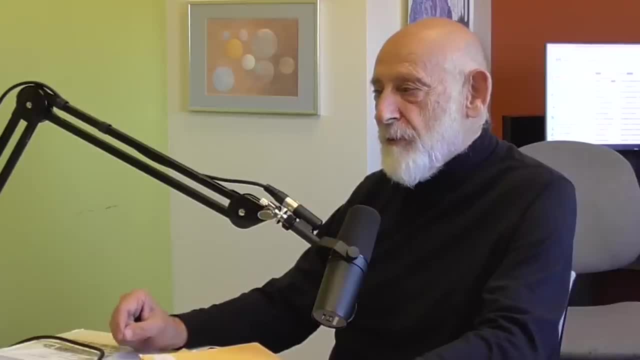 visualize in my head the one dimension, the two dimension, the four dimension, the five dimensions, and I don't think that's ever going to happen. The reason is, I think our neural wiring is just set up for that. On the other hand, we do learn ways to think about five, six, seven dimensions. 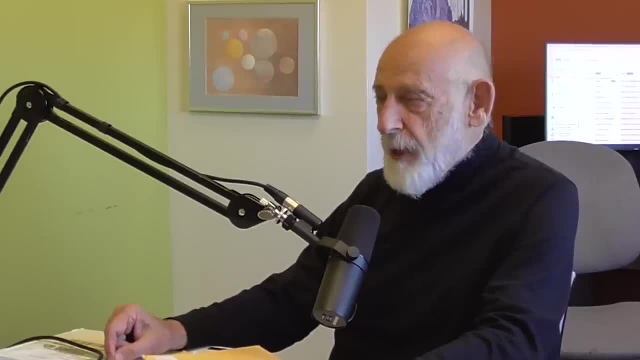 Right, We learn ways, we learn mathematical ways and we learn ways to visualize them, but they're different. And so, yeah, I think we do rewire ourselves, Whether we can ever completely rewire ourselves to be completely comfortable with these concepts. 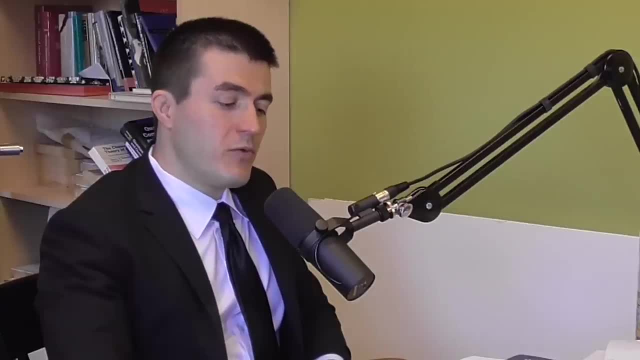 I doubt So that it's completely natural To where it's completely natural. So I'm sure there's somewhat, you could argue, creatures that live in a two-dimensional space? Yeah, Yeah, maybe there are. And while it's romanticizing the notion, of course, 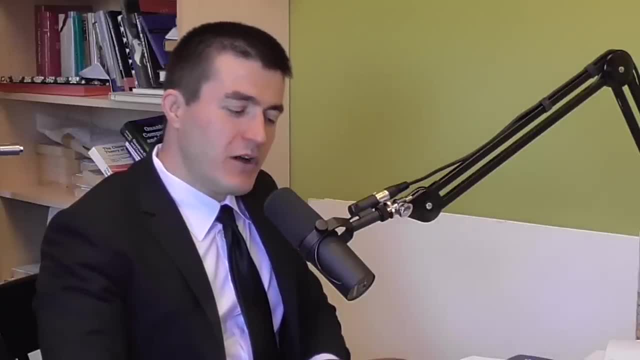 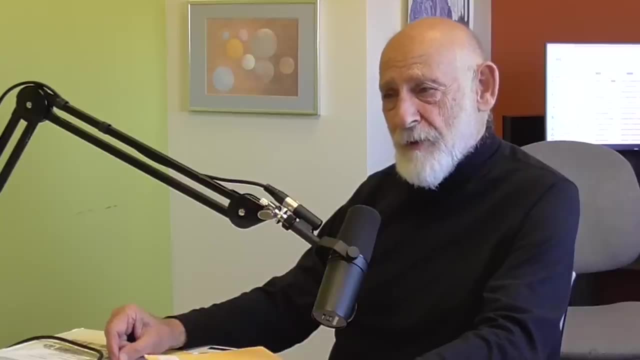 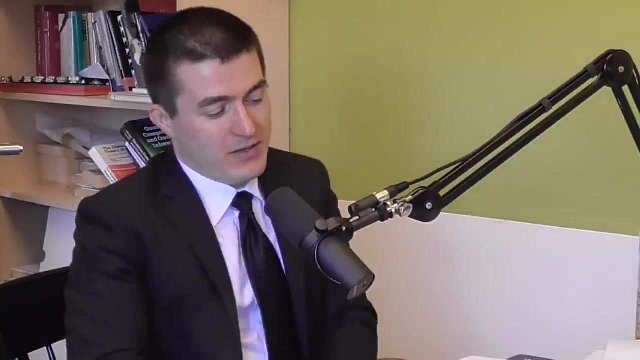 we're all living, as far as we know, in three-dimensional space. but how do those creatures imagine 3D space? Well, probably the way we imagine 4D: by using some mathematics and some equations and some tricks. Okay, so jumping back to Feynman just for a second, he had a little bit of an ego. 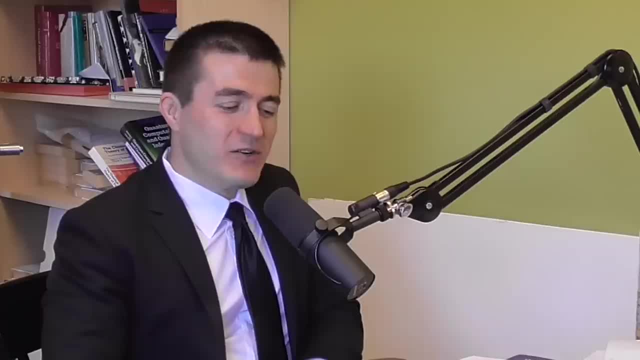 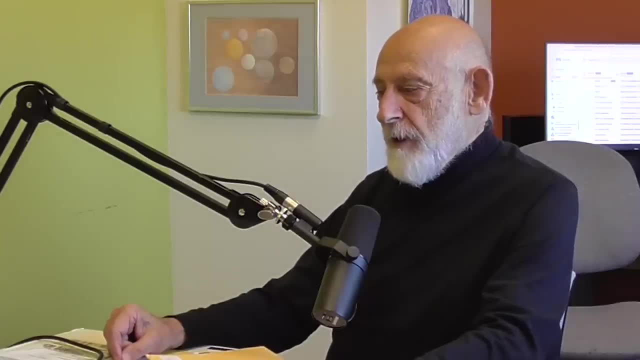 Yes. Well, do you think ego is powerful or dangerous in science? I think both, Both, Both. I think you have to have both arrogance and humility. You have to have the arrogance to say: I can do this. Nature is difficult. 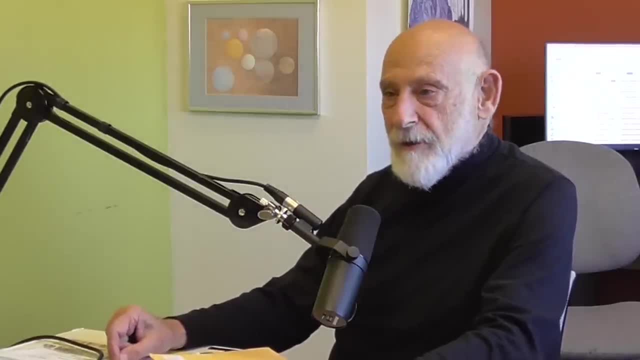 Nature is very, very hard. I'm smart enough. I can do it. I can win the battle with nature. On the other hand, I think you also have to have the humility to know that you're very likely to be wrong on any given occasion. 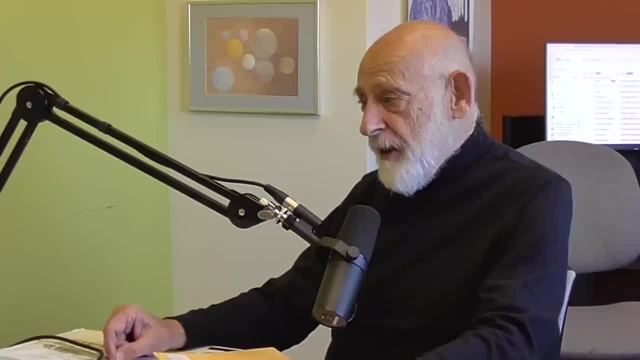 Everything you're thinking could suddenly change. Young people can come along and say things you won't understand, and you'll be lost and flabbergasted. So I think it's a combination of both. You better recognize that you're very limited and you better be able to say to yourself: 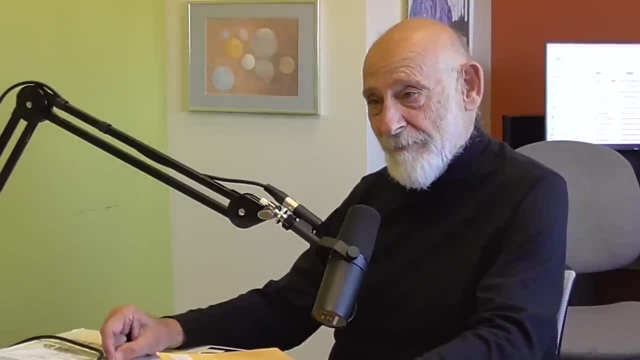 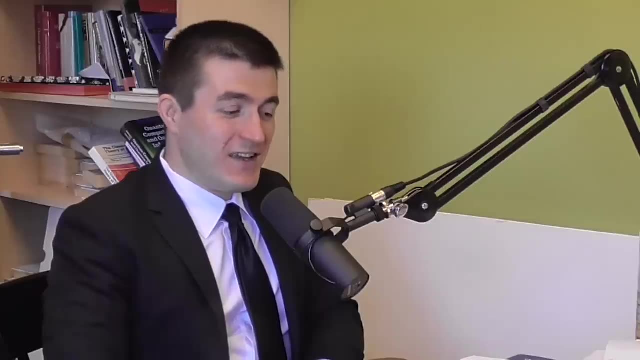 I'm not so limited that I can't win this battle with nature. It takes a special kind of person who can manage both of those. I would say, And I would say there's echoes of that in your own work- A little bit of ego, a little bit of outside of the box, humble thinking. 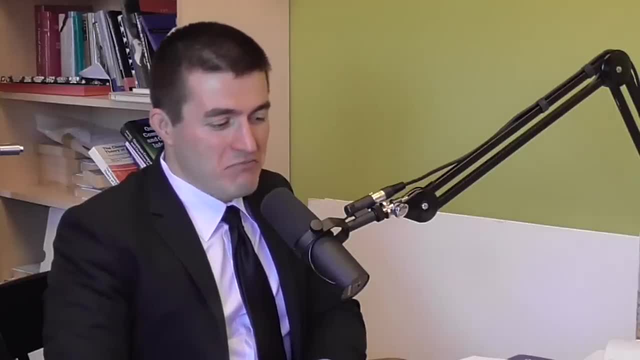 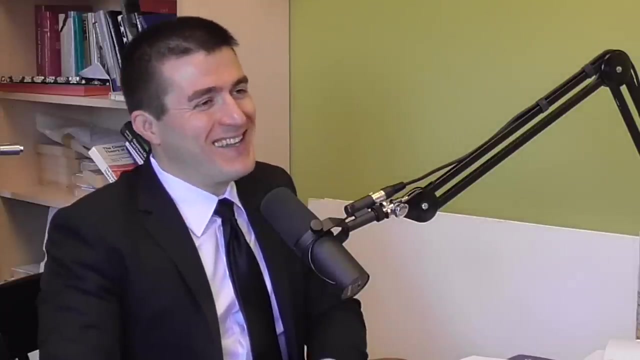 I hope so. So was there a time where you felt you looked at yourself and asked: am I completely wrong about this? Oh yeah, About the whole thing. Yeah, Yeah, About specific things. The whole thing. Wait, which whole? thing? 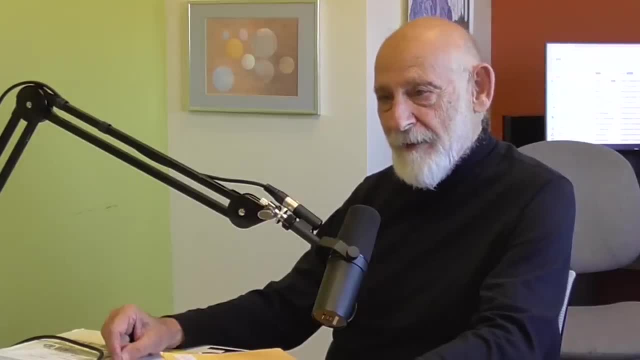 Me and me and my ability to do this thing. Oh, those kinds of doubts First of all. did you have those kinds of doubts? No, I had different kinds of doubts. I came from a very working class background and I was uncomfortable in academia. for 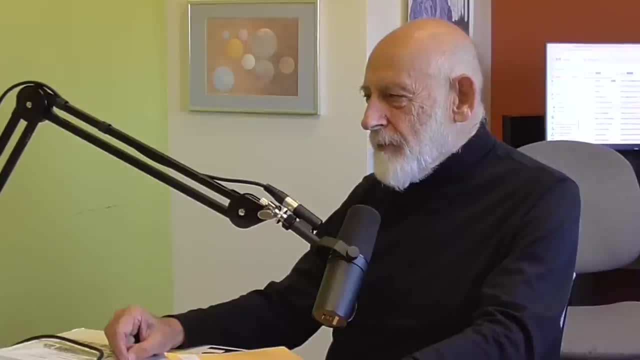 oh, for a long time. But they weren't doubts about my ability. they were just the discomfort in being in an environment that my family hadn't participated in I knew nothing about as a young person. I didn't learn that there was such a thing called physics until I was almost 20 years old. 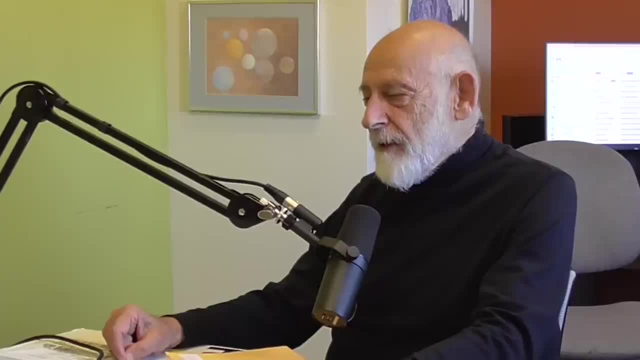 Yeah. So I did have certain kinds of doubts, but not about my ability. I don't think I was too worried about whether I would succeed or not. I never felt this insecurity: am I ever going to get a job? No, That had never occurred to me that I wouldn't. 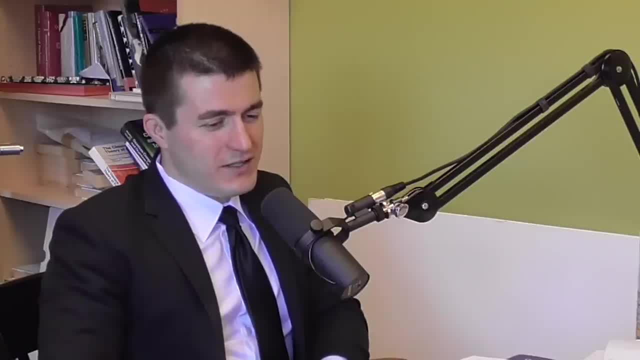 Maybe you could speak a little bit to this sense of what is academia, because I too feel a bit uncomfortable in it. There's something I can't put quite into words. what you have that's not doesn't. if we call it music, you play a different kind of music than a lot of academia. 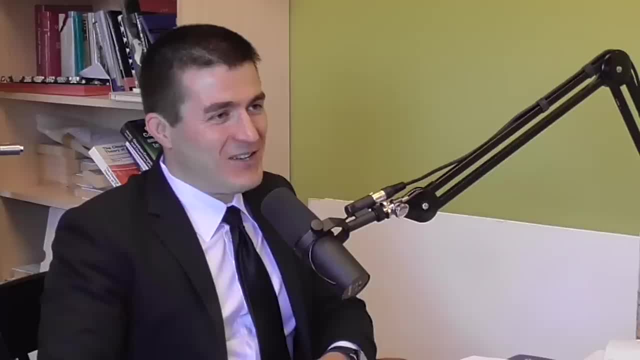 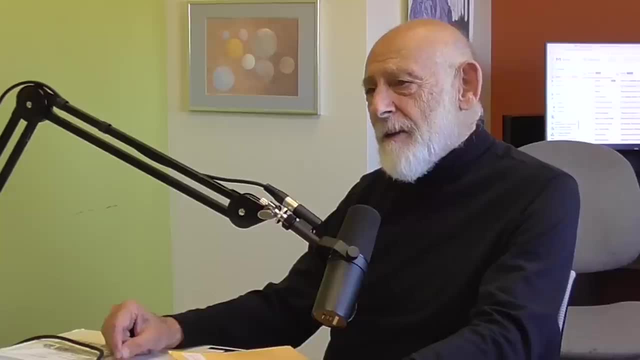 How have you joined this orchestra? How do you think about it? I don't know that I thought about it as much as I just felt it. Thinking is one thing, feeling is another thing. I felt like an outsider until a certain age, when I suddenly found myself the ultimate insider. 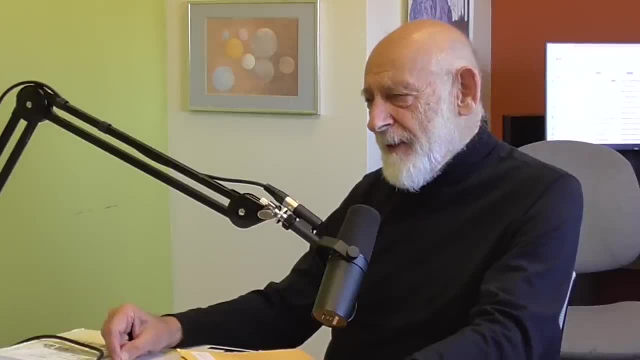 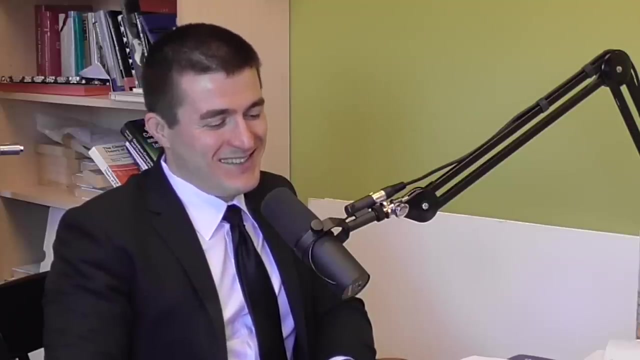 in academic physics. That was a sharp transition and I wasn't a young man, I was probably 50 years old. Yeah, You were never quite. it was a phase transition. you were never quite in the middle, Pretty much. Yeah, that's right, I wasn't. 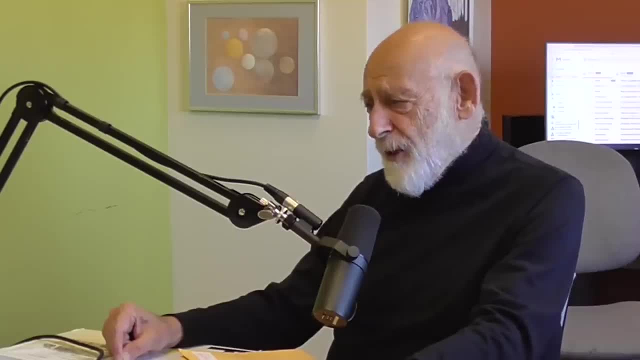 I always felt a little bit of an outsider In the beginning, a lot an outsider. My way of thinking was different, my approach to mathematics was different, but also my social background that I came from was different. You know, these days half the young people I meet 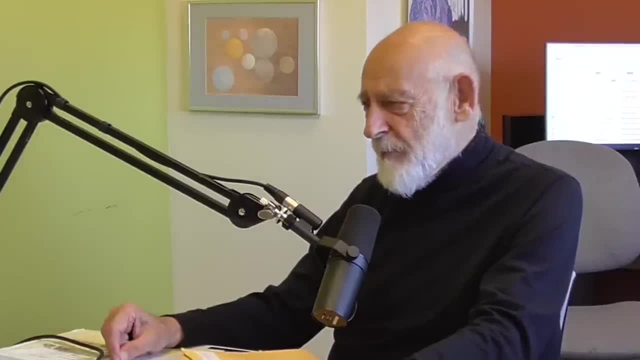 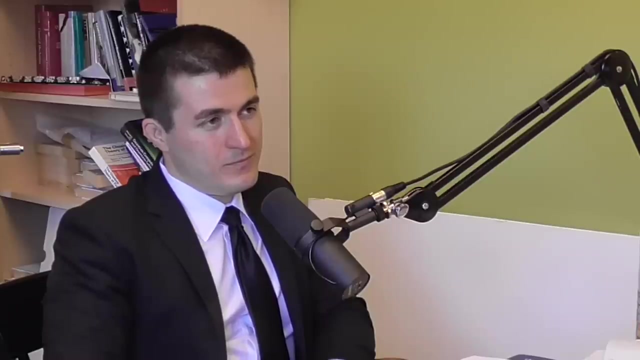 they're parents or professors, Right? That was not my case. So yeah, But then all of a sudden, at some point, I found myself at very much the center of- maybe not the only one at the center, but certainly one of the people in the center. 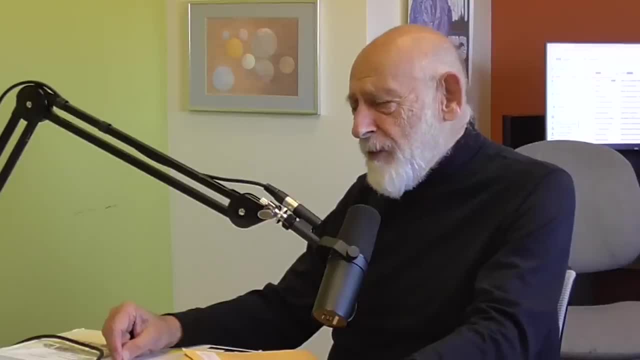 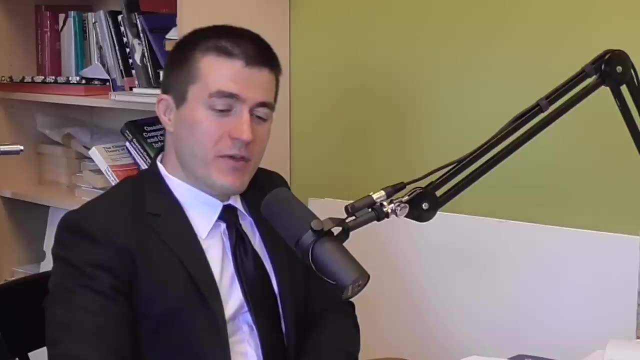 of a certain kind of physics And all that went away. I mean, it went away in a flash. So maybe a little bit. I know you've worked with Feynman, but in general, how do you develop ideas? Do you work through ideas alone? 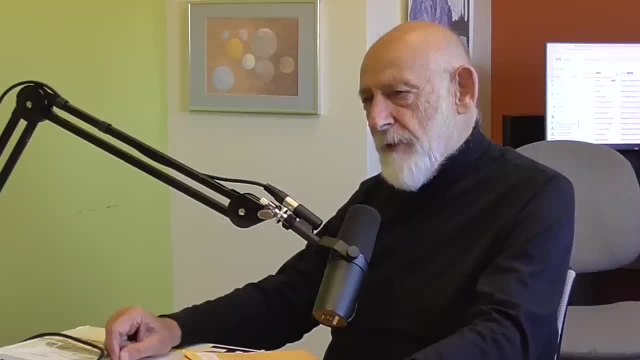 Do you brainstorm with others? Oh, both, Both, Very definitely both The younger time. I spent more time with myself Now because I'm at Stanford, because I have a lot of ex-students and people who are interested in the same thing. I am. 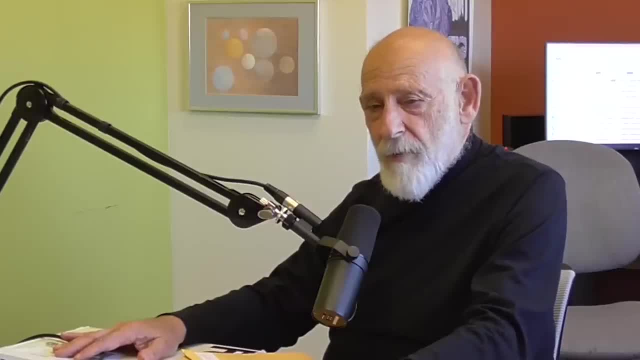 I spend a good deal of time almost on a daily basis interacting, brainstorming, as you said. It's a very important part. I spend less time, probably completely self-focused with a piece of paper and just sitting there staring at it. 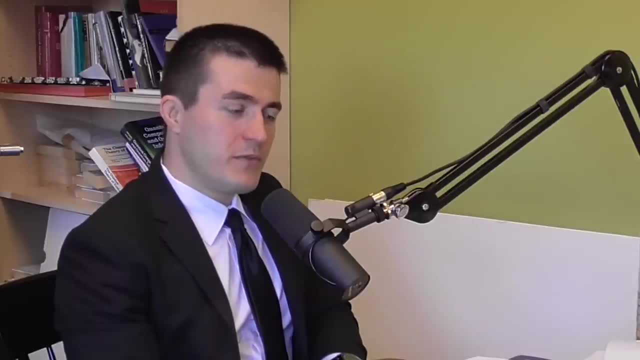 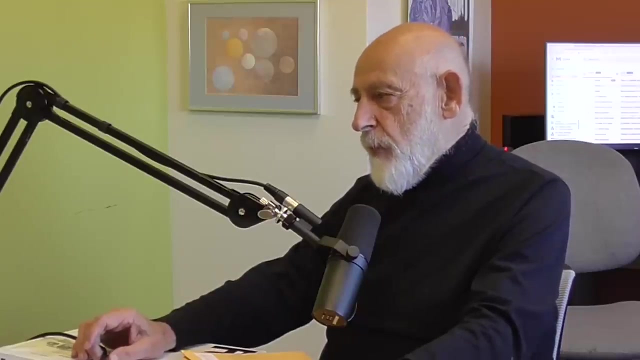 What are your hopes for quantum computers? So machines that are based on that have some elements of leveraged quantum mechanical ideas. Yeah, It's not just leveraging quantum mechanical ideas. You can simulate quantum systems on a classical computer. Simulate them means solve the Schrodinger equation for them or solve the equations. 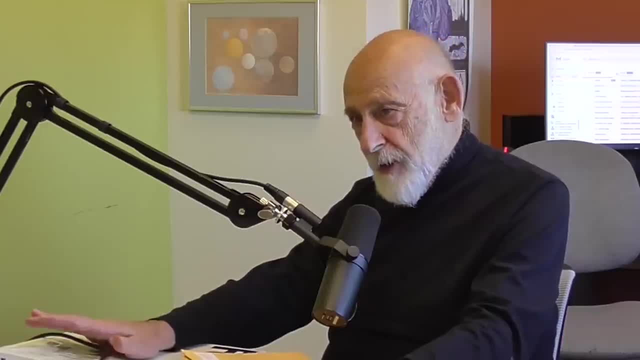 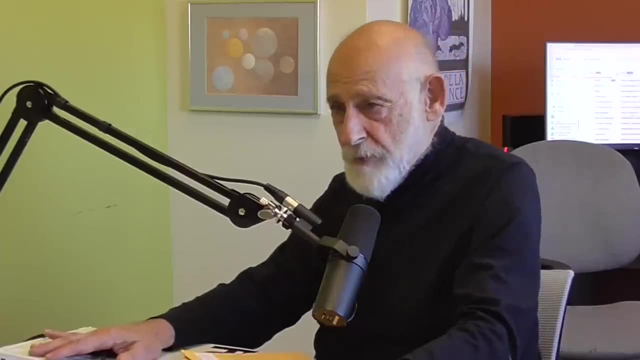 of quantum mechanics on a computer, on a classical computer. But the classical computer is not doing, is not a quantum mechanical system itself? Oh, of course it is. Everything's made of quantum mechanics, but it's not functioning. It's not functioning as a quantum system. It's just solving equations. The quantum computer is truly a quantum system which is actually doing the things that you're programming it to do. You want to program a quantum field theory. If you do it in classical physics, that program is not actually functioning in the computer. 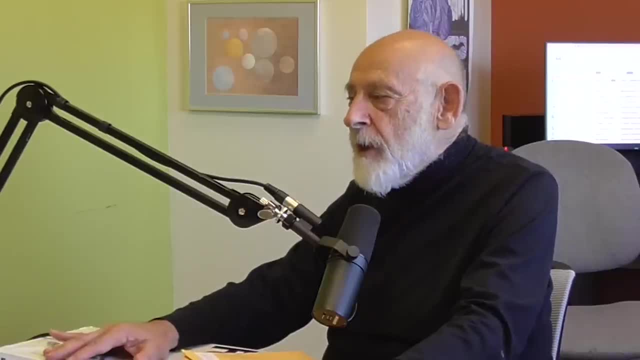 as a quantum field theory. It's just solving some equations Physically. it's not doing the things that the quantum system would do. The quantum computer is really a quantum mechanical system which is actually carrying out the quantum operations. You can measure it at the end. 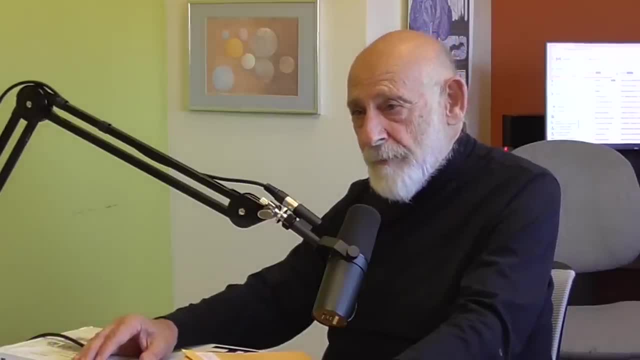 It intrinsically satisfies the uncertainty principle. It is limited, in the same way that quantum systems are limited by uncertainty and so forth, And it really is a quantum system. That means that what you're doing when you program something for a quantum system is you're actually building. 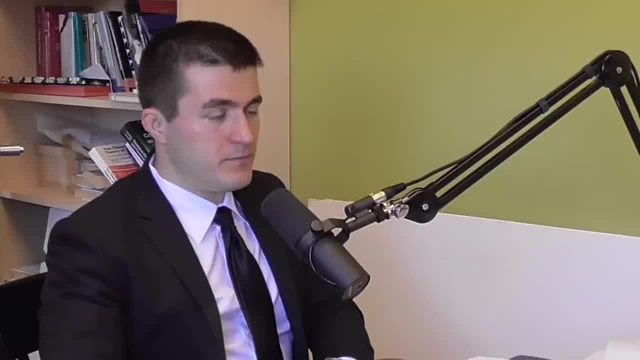 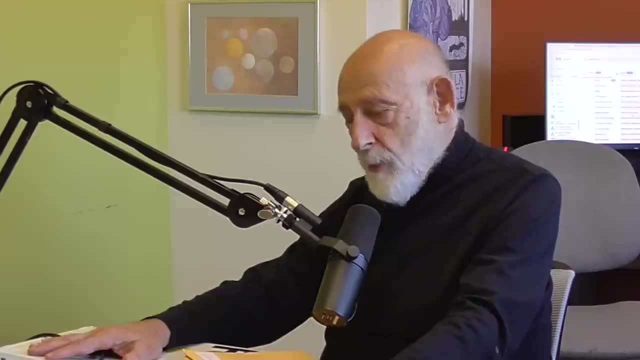 a real version of the system. The limits of a classical computer. Classical computers are enormously limited. when it comes to quantum systems, They're enormously limited because- you've probably heard this before- but in order to store the amount of information that's in a quantum state of. 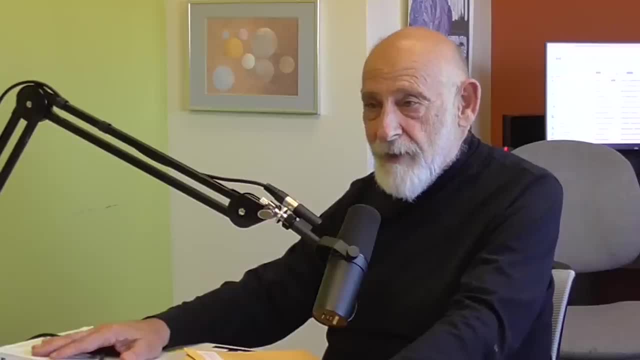 400 spins. That's not very many. I can put 400 pennies in my pocket To be able to simulate the quantum state of 400 elementary quantum systems, qubits we call them. to do that would take more information than can possibly be stored in the entire. 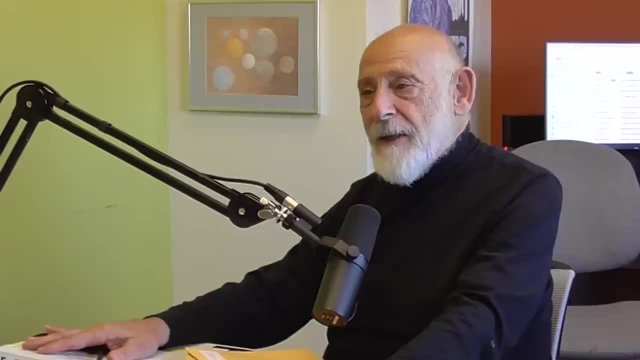 universe if it were packed so tightly that you couldn't pack any more than what you need. Well, commentum quanta in 400 qubits. On the other hand, if your quantum computer is composed of 400 qubits, it can do everything. 400 qubits can do What kind of space, if you just intuitively think. 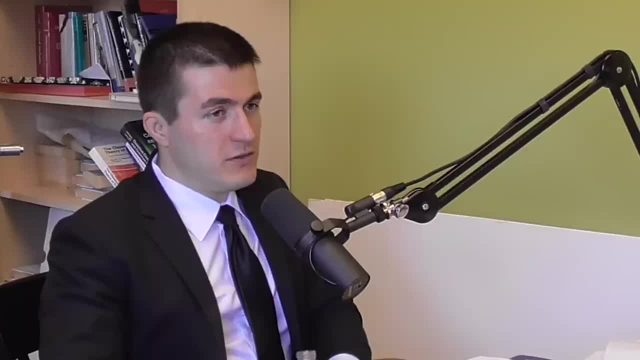 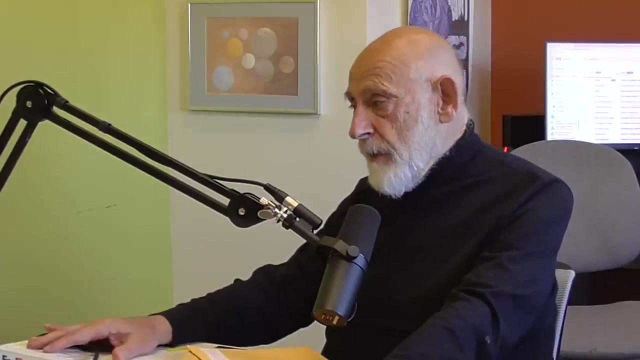 about the space of algorithms that that unlocks for us. So there's a whole complexity theory around classical computers measuring the running time of things, NP, so on. What kind of algorithms, just intuitively, do you think it unlocks for us? Okay, so we know that there are a handful. 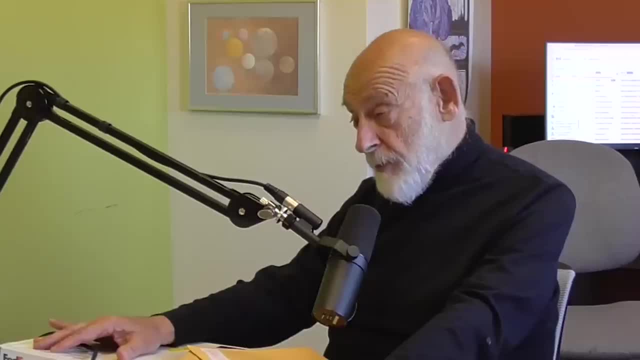 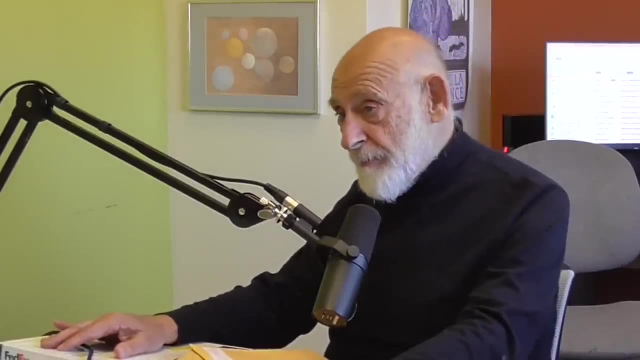 of algorithms that can seriously beat classical computers and which can have exponentially more power. This is a mathematical statement. Nobody's exhibited this in the laboratory. It's a mathematical statement. We know that's true. but it also seems more and more that the 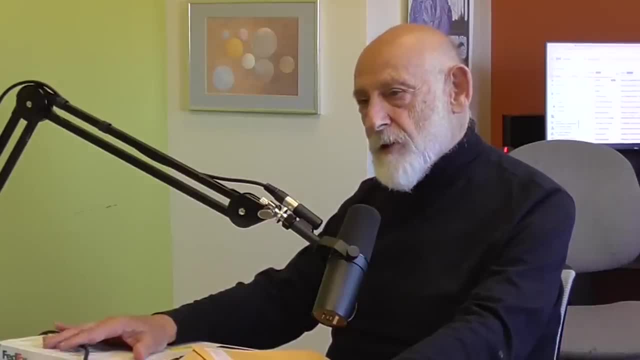 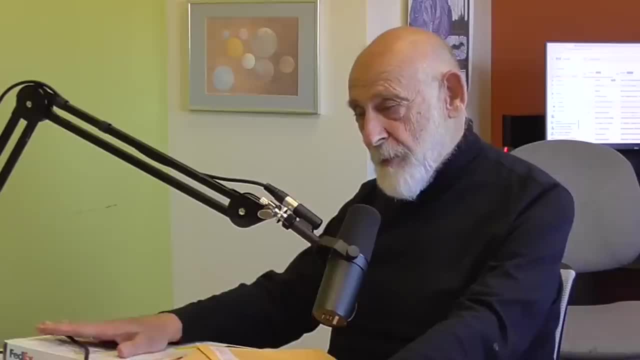 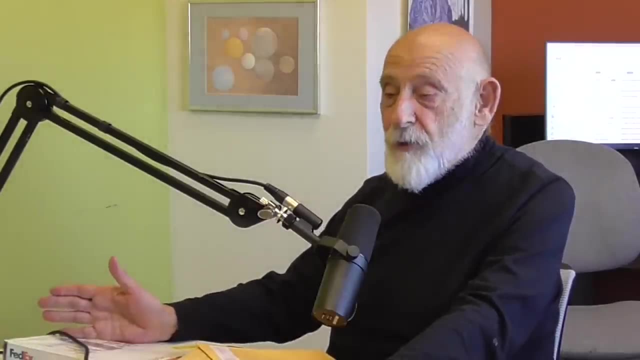 quantum system. You make measurements on it, quantum measurements on it. The advantage is you can run it much slower. You could say, why bother, Why not just use the real system? Why not just do experiments on the real system? Well, real systems are kind of limited, You can't. 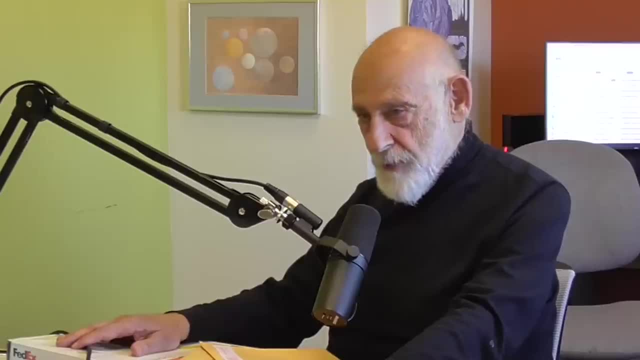 change them. You can't manipulate them, You can't slow them down so that you can poke into them. You can't modify them in arbitrary kinds of ways to see what would happen if I change the system a little bit. So I think that quantum computers 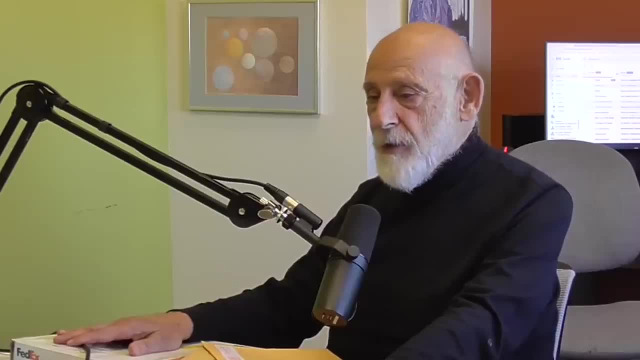 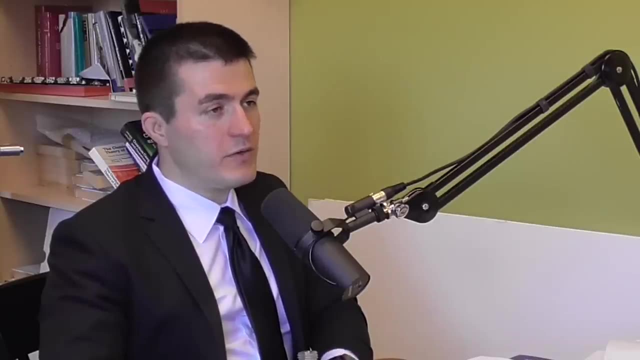 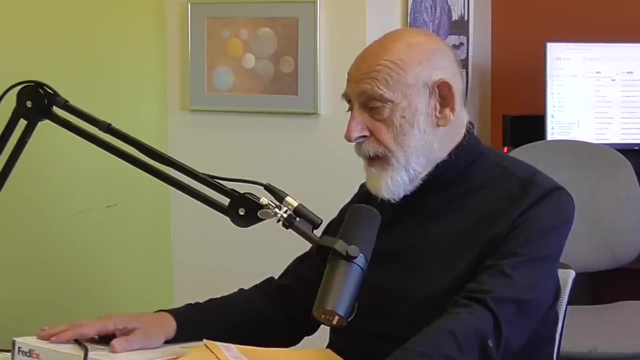 will be extremely valuable in understanding quantum systems At the lowest level, the fundamental laws. They're actually satisfying the same laws as the systems that they're simulating. That's right, Okay. So on the one hand, you have things like factoring. Factoring is the great. the thing of quantum computers factoring large numbers. That doesn't seem that much to do with quantum mechanics. It seems to be almost a fluke that a quantum computer can solve the factoring problem in a short time, And those problems seem to be extremely special. 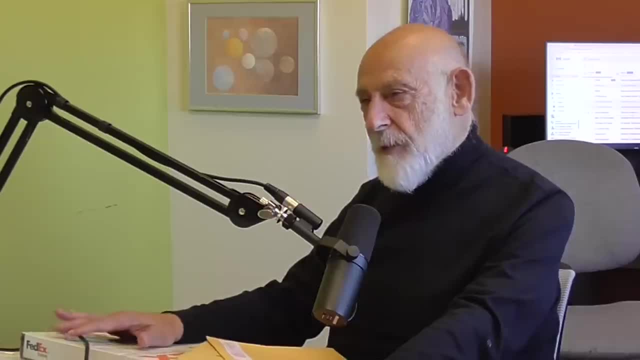 rare and it's not clear to me that there's going to be a lot of them. On the other hand, there are a lot of quantum systems. There's chemistry, there's solid state physics, there's material science, there's quantum gravity, there's all kinds of quantum field theory. 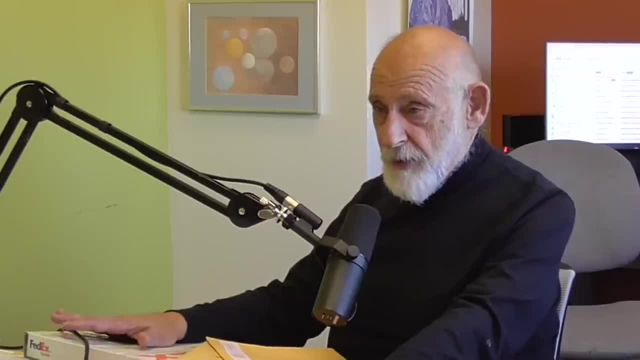 And some of these are actually turning out to be applied sciences as well as very fundamental sciences. So we probably will run out of the ability to solve equations for these things. Solve equations by the standard methods of pencil and paper. Solve the equations by the method of. 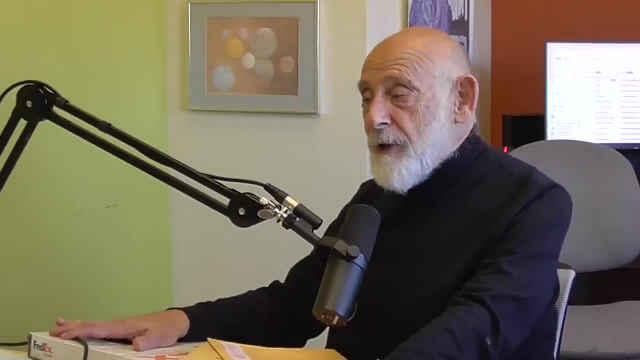 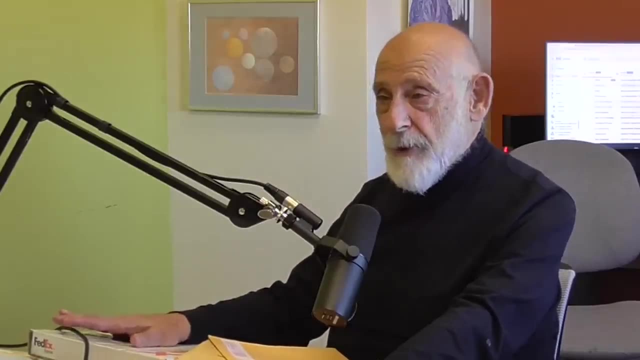 classical computing, And so what we'll do is we'll build versions of these systems, run them and run them under controlled circumstances, where we can change them, manipulate them, make measurements on them and find out all the things we want to know. 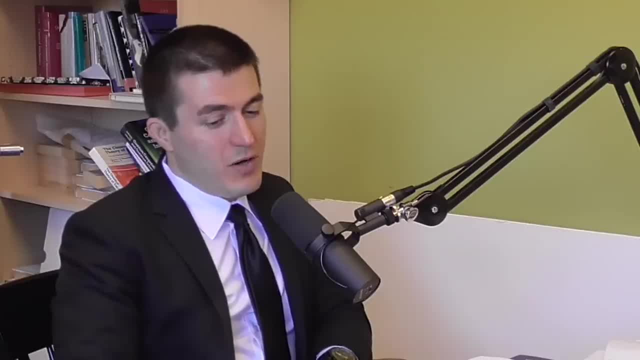 So, in finding out the things we want to know about very small systems, right? Is there something we can also find out about the macro level, about something about the function, And forgive me- of our brain biological systems? the stuff that's about one meter in size versus much, much smaller? 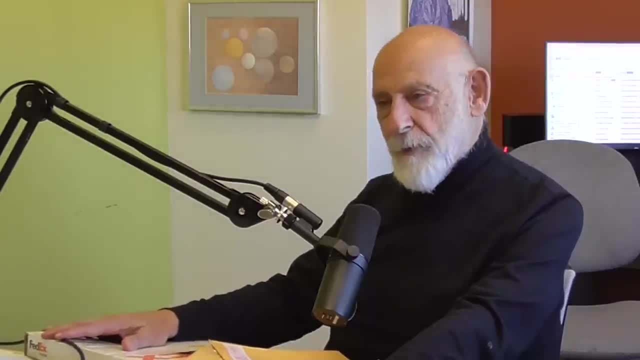 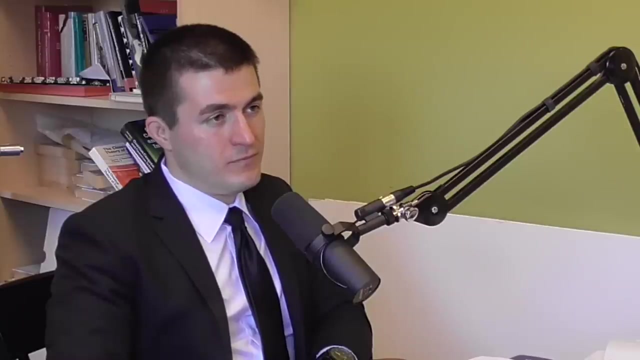 Well, what all the excitement is about among the people that I interact with is understanding black holes. Black holes are big things. They are many, many degrees of freedom. There is another kind of quantum system that is big. It's a large quantum computer. 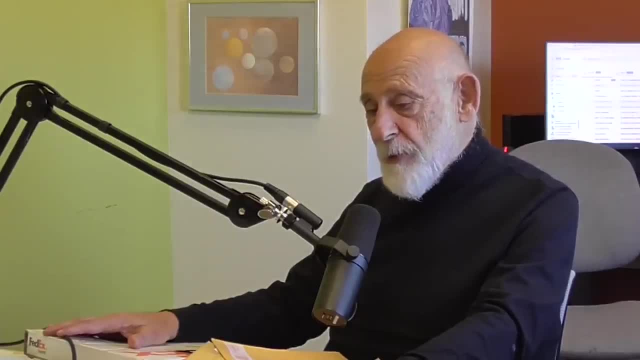 And one of the things we've learned is that the physics of large quantum computers is in some ways similar to the physics of large quantum black holes, And we're using that relationship. Now, you didn't ask about quantum computers or systems. 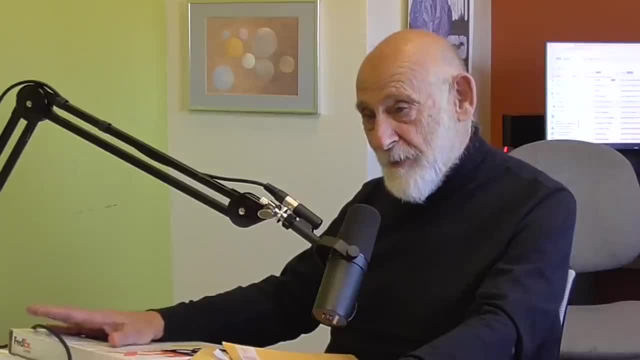 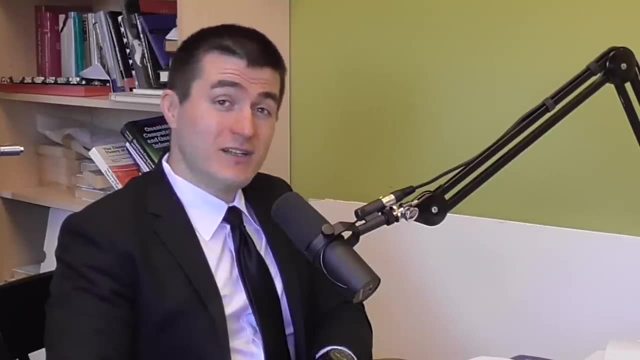 You didn't ask about black holes. You asked about brains, Yeah, about stuff that's in the middle of the two. It's different. So black holes- there's something fundamental about black holes that feels to be very different than brains. Yes, 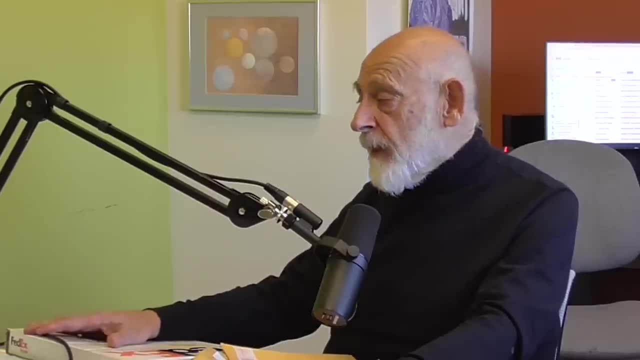 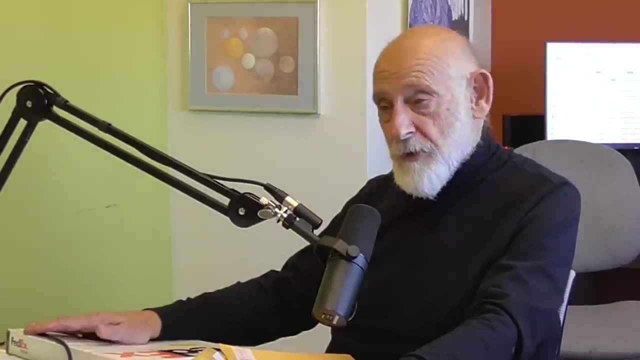 And they also function in a very, In a very quantum mechanical way, Right, Okay, It is first of all unclear to me. but of course it's unclear to me. I'm not a neuroscientist. I don't even have very many friends who are neuroscientists. 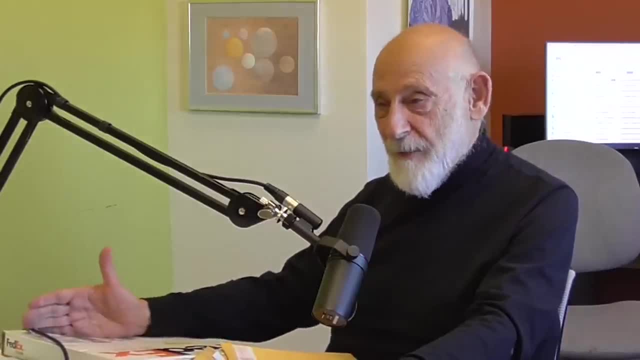 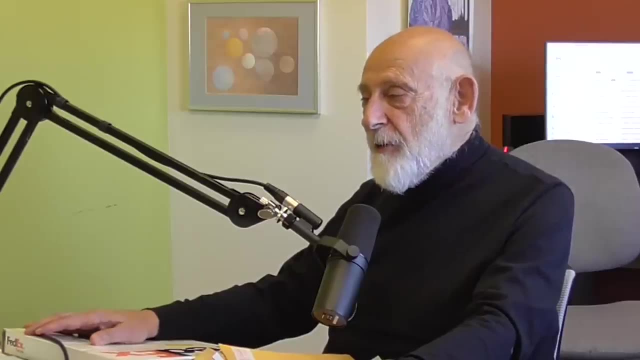 I would like to have more friends who are neuroscientists. I just don't run into them very often. Among the few neuroscientists I've ever talked about about this, they are pretty convinced that the brain functions in a very quantum mechanical way. 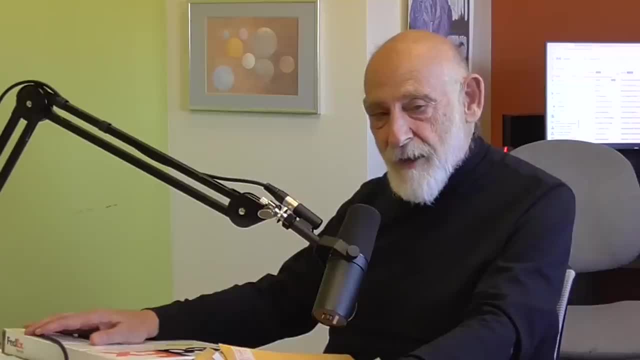 Functions classically, That it is not intrinsically a quantum mechanical system or it doesn't make use of the special features, entanglement, coherence, superposition. Are they right? I don't know. I sort of hope they're wrong, just because I like the romantic idea that 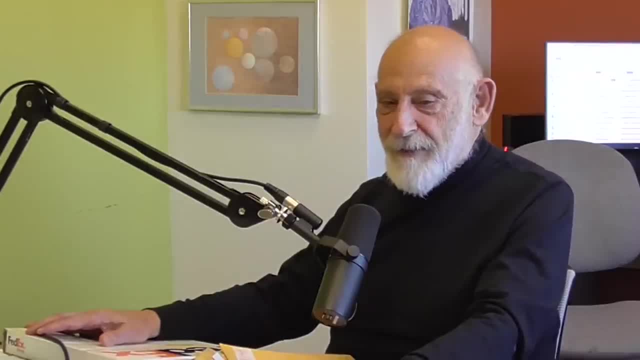 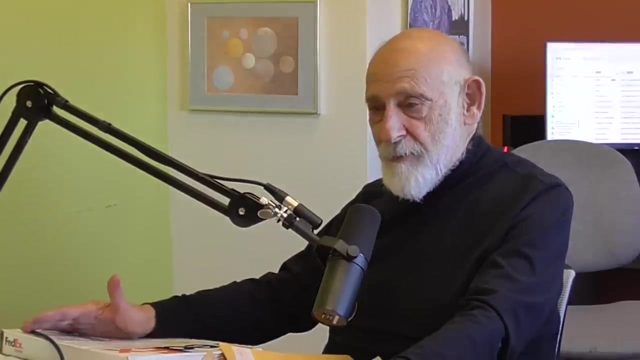 the brain is a quantum system. Yeah, But I think probably not The other thing. big systems can be composed of lots of little systems. Okay, Materials, The materials that we work with, and so forth, can be large systems, a large piece of material, but they're made out of quantum systems. Now, one of the things that's 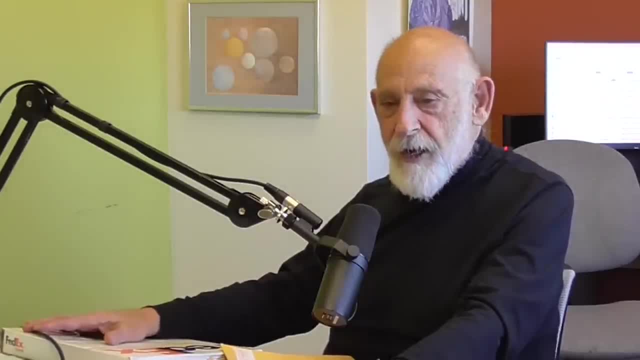 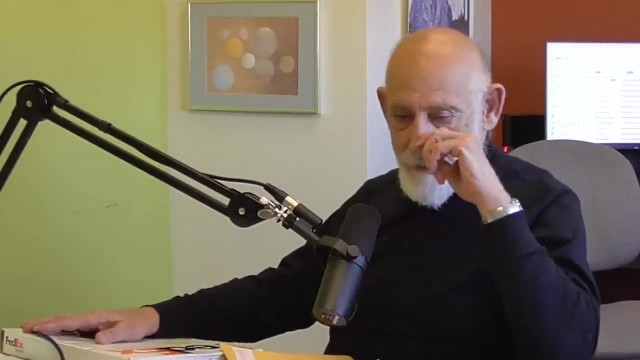 been happening over the last good number of years is: we're discovering materials and quantum systems which function much more quantum mechanically than we imagine. Topological insulators, this kind of thing, that kind of thing, Those are macroscopic systems, but they're just superconductors. Superconductors have 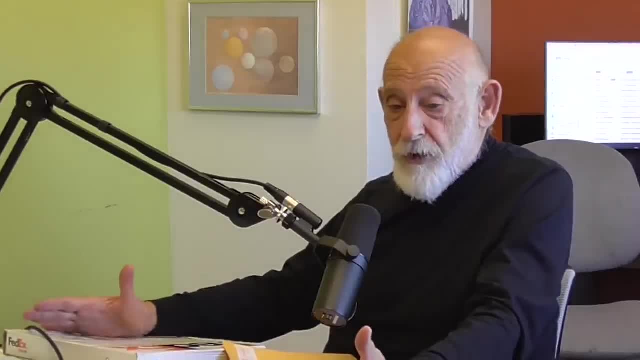 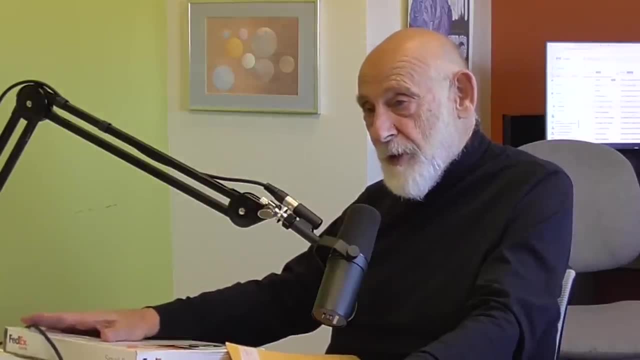 a lot of quantum mechanics in them. You can have a large chunk of superconductor, so it's a big piece of material. On the other hand, it's functioning and its properties depend very, very strongly on quantum mechanics, And to analyze them you need the tools of. 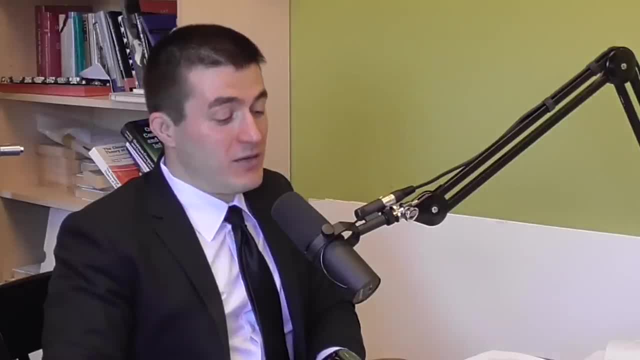 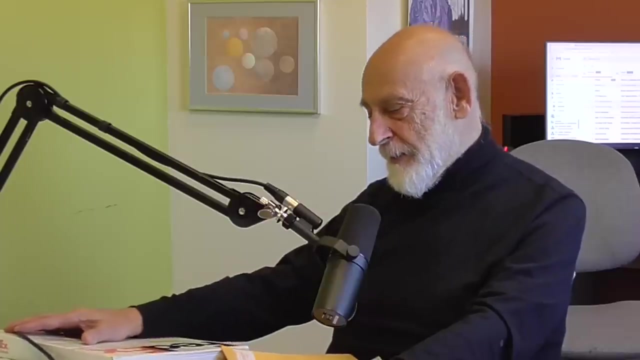 quantum mechanics, If we can go on to black holes and looking at the universe. The universe is an information processing system. It's a computer. It's a giant computer. It's a giant computer. What's the power of thinking of the universe as an information processing system? Perhaps? 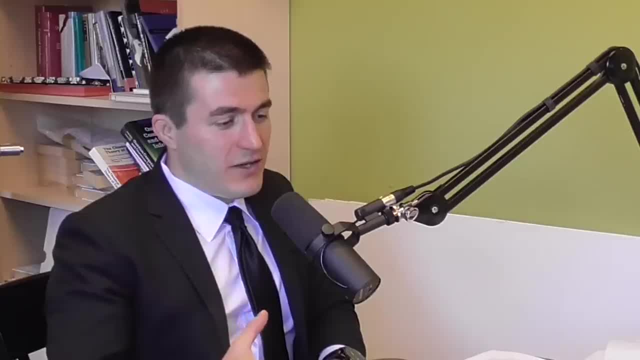 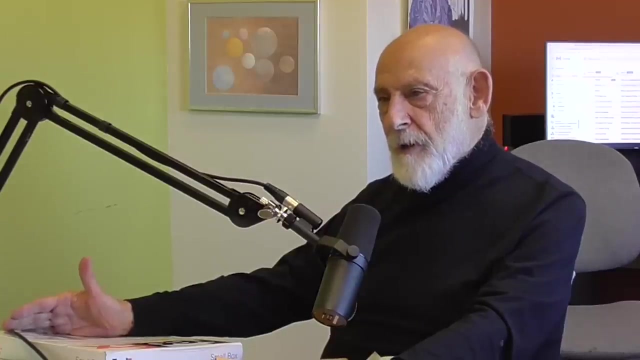 its use- besides the mathematical use of discussing black holes and your famous debates and ideas around that- to human beings or life in general, as information processing systems. All systems are information processing systems. You poke them, they change a little bit, they evolve. All systems are information. 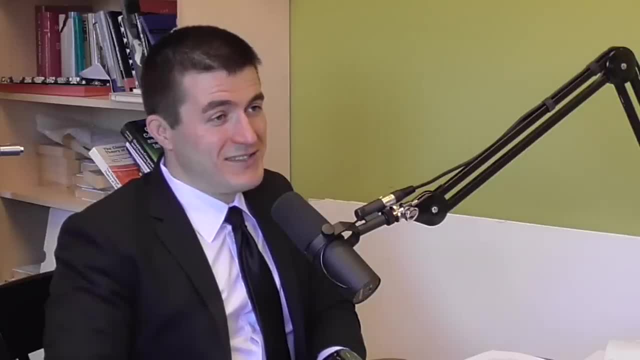 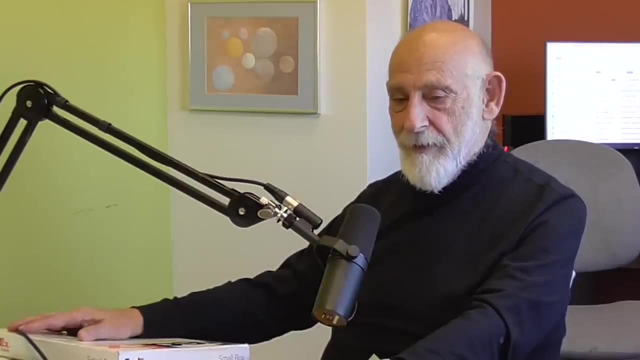 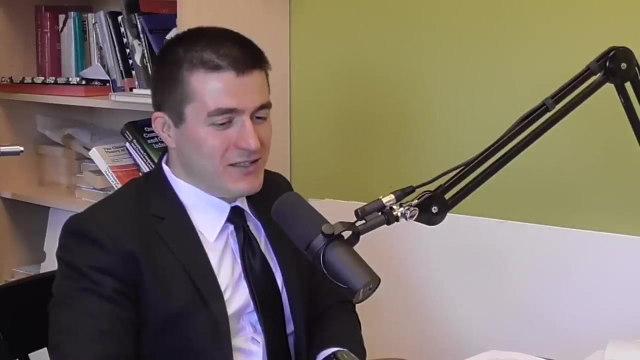 processing systems. So there's no extra magic to us humans. It certainly feels consciousness and intelligence feels like magic. It sure does. Where does it emerge from? If we look at information processing, what are the emerging phenomena that come from viewing the world as an information processing system? 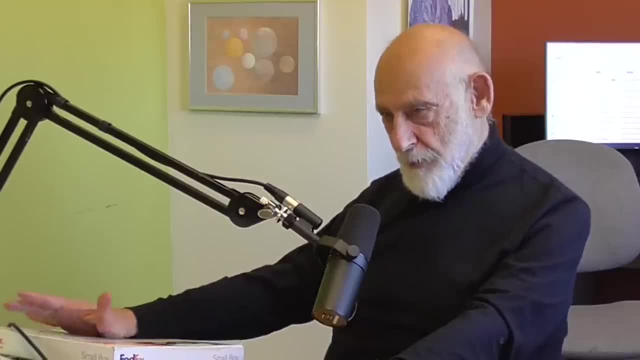 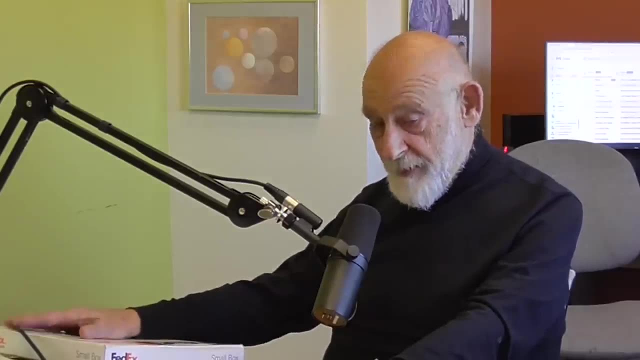 Here is what I think My thoughts on that are worth much in this. If you ask me about physics, my thoughts may be worth something. If you ask me about this, I'm not sure my thoughts are worth anything. But as I said, 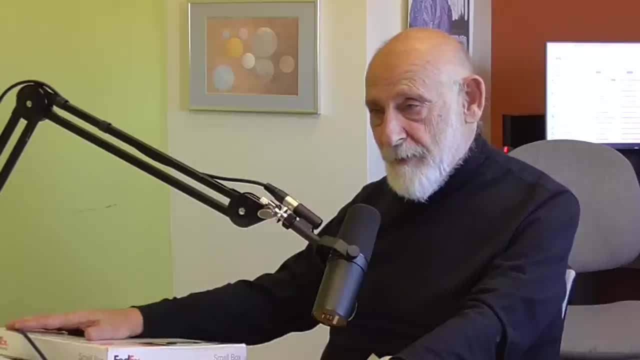 earlier. I think when we do introspection, when we imagine doing introspection and try to figure out what it is, when we do and we're thinking I think we get it wrong. I'm pretty sure we get it wrong. Everything I've heard about the way the brain functions is so counterintuitive. 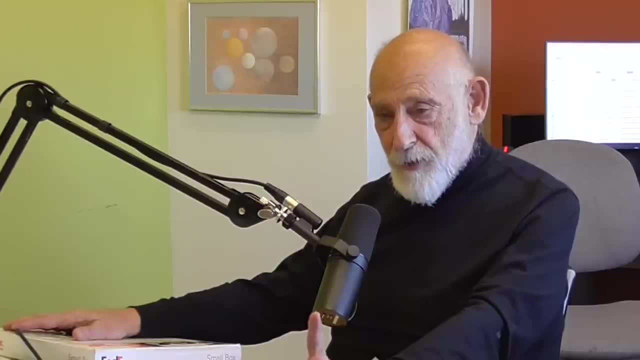 For example, you have neurons which detach- Yeah, You have neurons which detect vertical lines. You have different neurons which detect lines at 45 degrees. You have different neurons. I never imagined that there were whole circuits which were devoted to vertical lines in my brain. 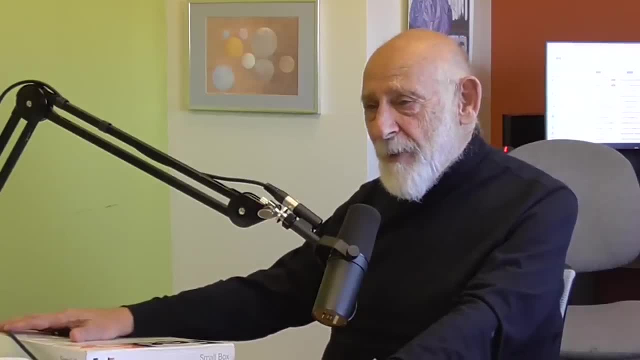 Yeah, It doesn't seem to be the way my brain works. My brain seems to work. if I put my finger up vertically, or if I put it horizontally, or if I put it this way or that way, it seems to me it's the same circuits that are. It's not the way it works, The way the brain is. 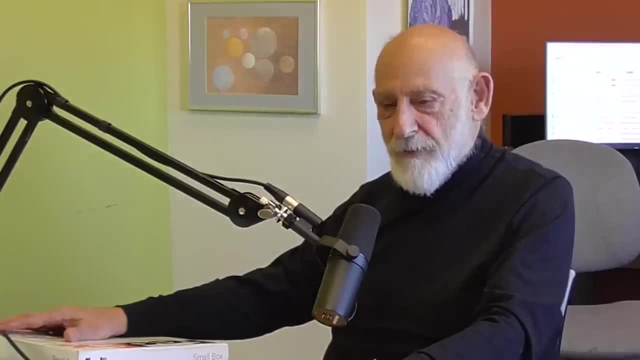 compartmentalized, seems to be very, very. It seems to be very, very different than what I would have imagined if I were just doing psychological introspection about how things work. My conclusion is that we won't get it right that way. How will we get it right? I think maybe computer scientists will. 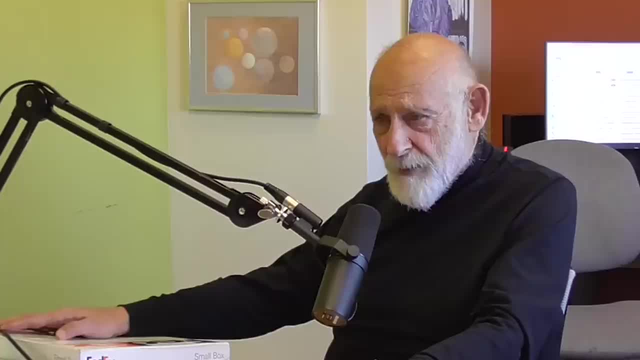 get it right eventually. I don't think they're anywhere near it, I don't even think they're thinking about it, But by computer, Eventually we will build machines, perhaps, which are complicated enough, partly engineered, partly evolved, maybe evolved by machine learning. 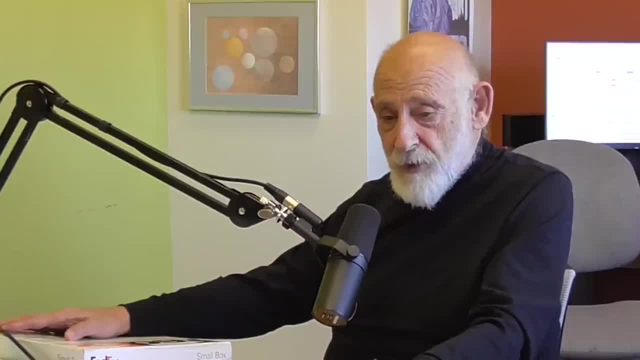 and so forth. Machine learning is very interesting. By machine learning, we will evolve systems and we may start to discover mechanisms that have implications for how we think and for what this consciousness thing is all about, And we'll be able to do experiments on them. 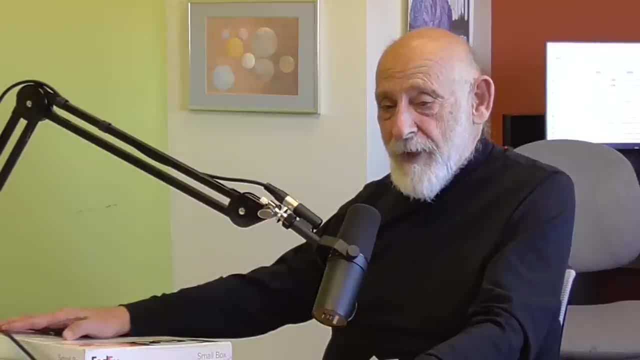 and perhaps answer questions that we can't possibly answer by introspection. So that's a really interesting point. In many cases, if you look at even a string theory, when you first think about a system it seems really complicated, like the human. 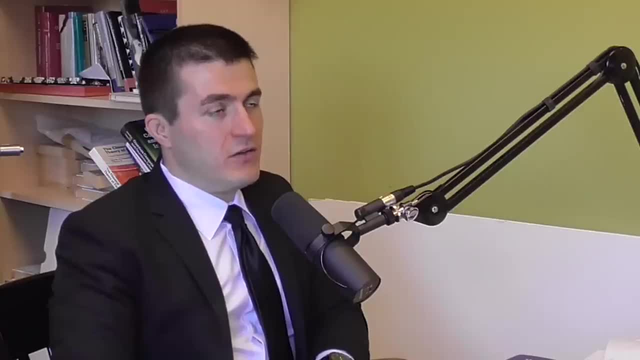 brain And through some basic reasoning and trying to discover fundamental low-level behavior of the system, you find out that it's actually much simpler. Do you One? have you Is that generally the process? And two, do you have that also hope for biological? 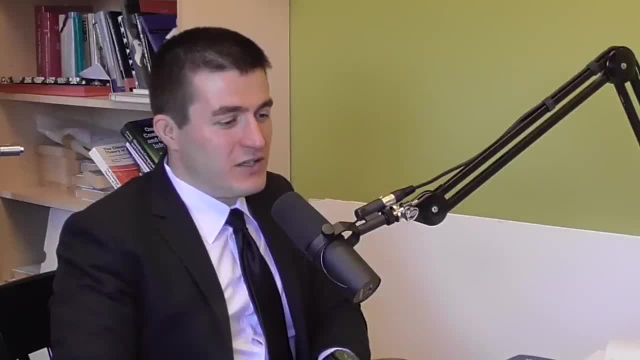 systems as well for all the kinds of stuff we're studying at the human level. Of course, physics always begins by trying to find the simplest version of something and analyze it. Yeah, I mean, there are lots of examples where physics has taken very complicated. 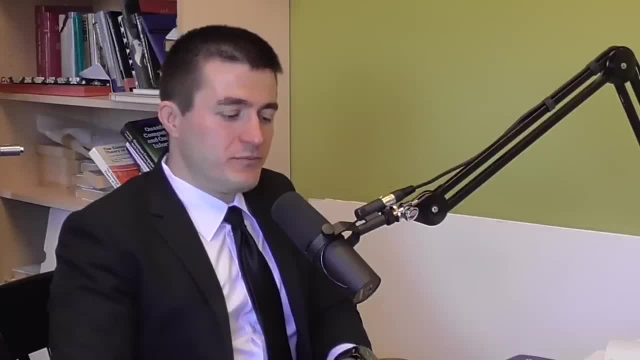 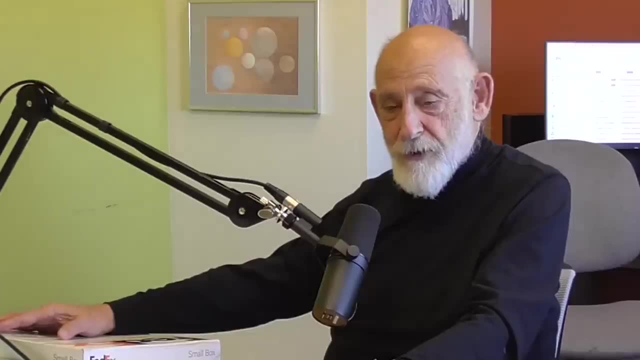 systems, analyzed them and found simplicity in them. for sure. I said superconductors before. It's an obvious one. A superconductor seems like a monstrous thing. It's a very complicated thing with all sorts of crazy electrical properties- magnetic. 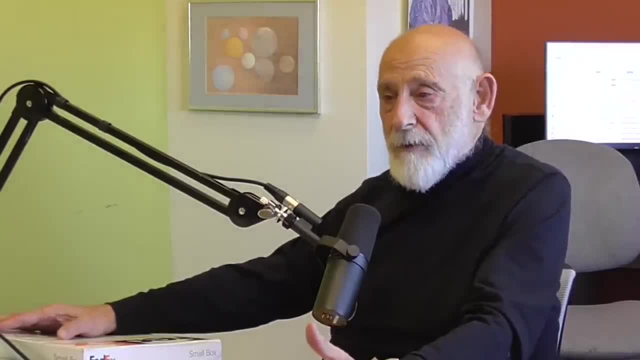 properties and so forth. And when it finally is boiled down to its simplest elements, it's a very simple quantum mechanical phenomenon called spontaneous symmetry breaking, which in other contexts we learned about and we're very familiar with. So yeah, I mean yes. 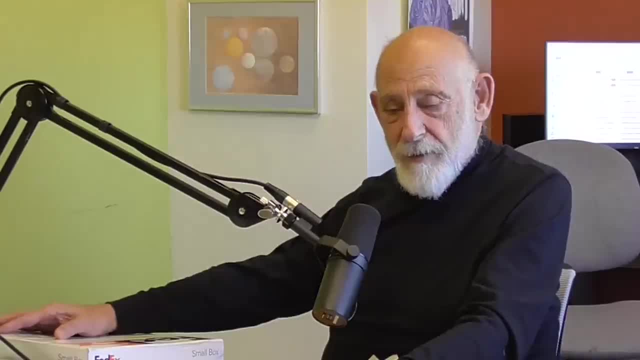 we do take complicated things, make them simple- Yeah, But what we don't want to do is take things which are intrinsically complicated and fool ourselves into thinking that we can make them simple. We don't want to make- I don't know who said this- but we don't want to make them simpler than they really are. 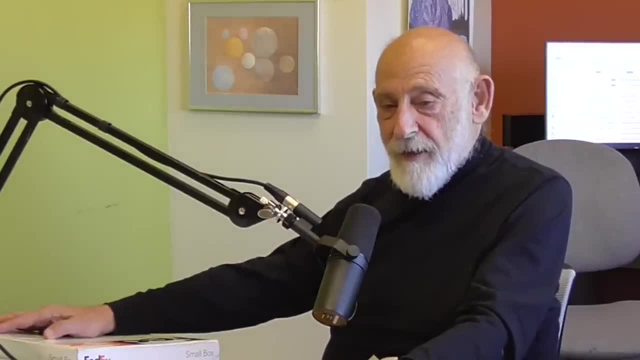 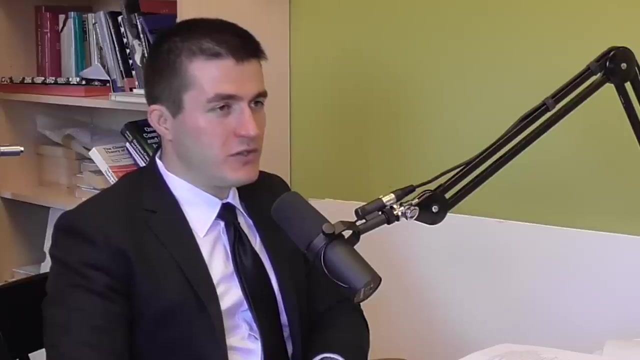 Right, Okay, Is the brain a thing which ultimately functions by some simple rules, or is it just complicated? In terms of artificial intelligence, nobody really knows what are the limits of our current approaches. You mentioned machine learning. How do we create human level intelligence? 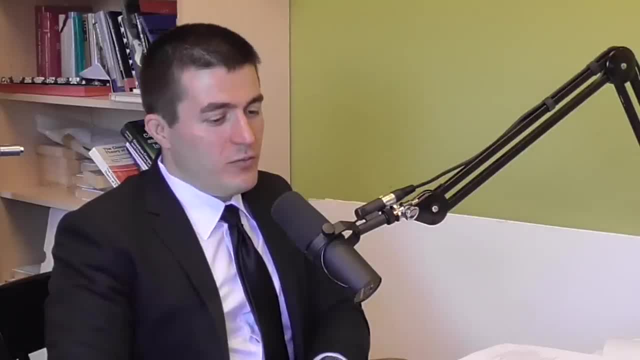 It seems that there's a lot of very smart physicists who perhaps oversimplify the nature of intelligence and think of it as information processing, And therefore there doesn't seem to be any theoretical reason why we can't artificially create human level or superhuman level intelligence. In fact, the reasoning goes: if you create human level intelligence, 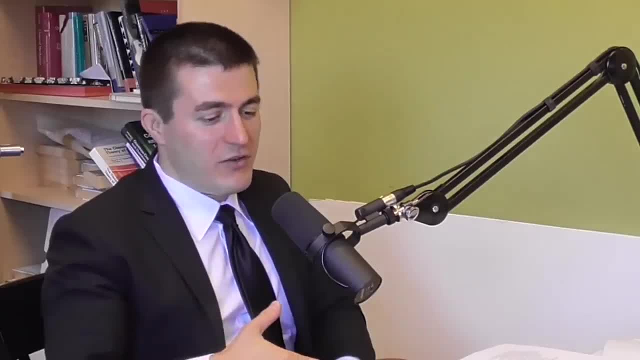 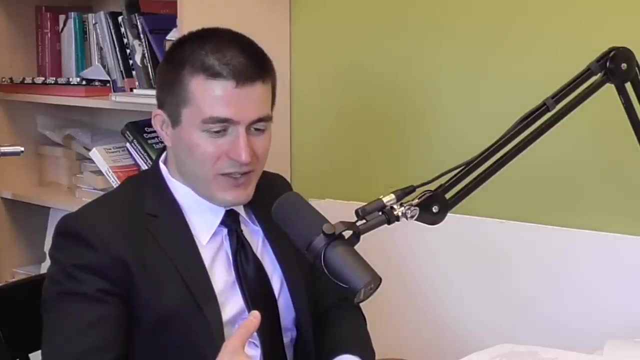 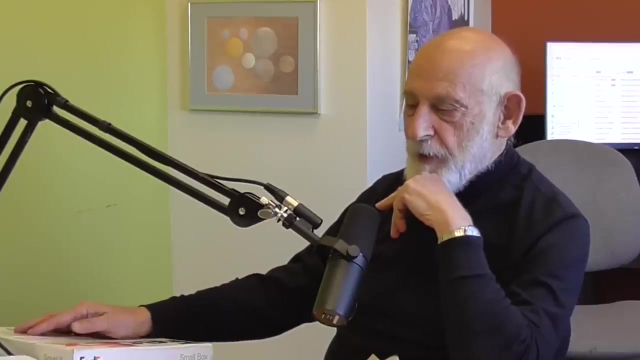 the same approach you just used to create human level intelligence should allow you to create superhuman level intelligence very easily, exponentially. So what do you think that way of thinking that comes from physicists is all about? I wish I knew, but there's a particular reason why I wish I knew. I have a second job. I 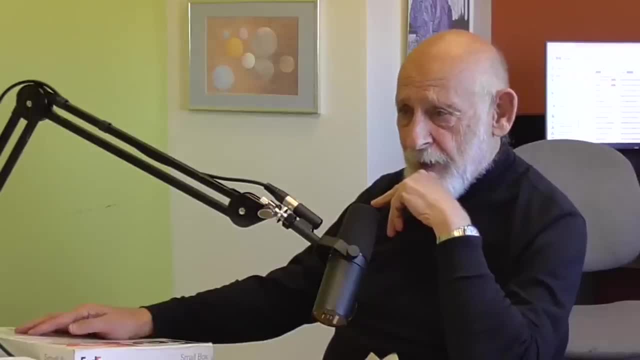 consult for Google, Not for Google for Google X. I am the senior academic advisor to a group of machine learning physicists. Okay, Now that sounds crazy, because I know nothing about the subject. I know very little about the subject. On the other hand, I'm good at giving advice, so I give them advice. 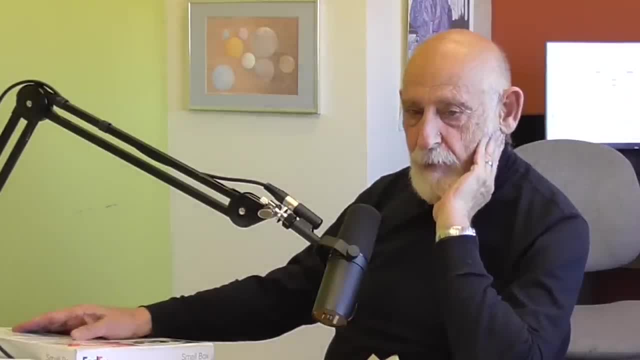 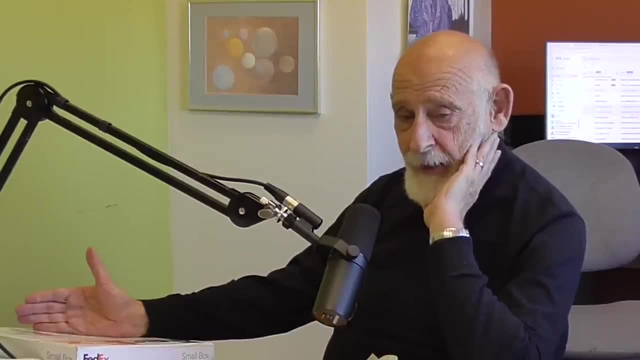 on things. Anyway, I see these young physicists who are approaching the machine learning problem. There is a real machine learning problem. Mainly, why does it work as well as it does? Nobody really seems to understand why it is capable of doing the kind of generalizations. 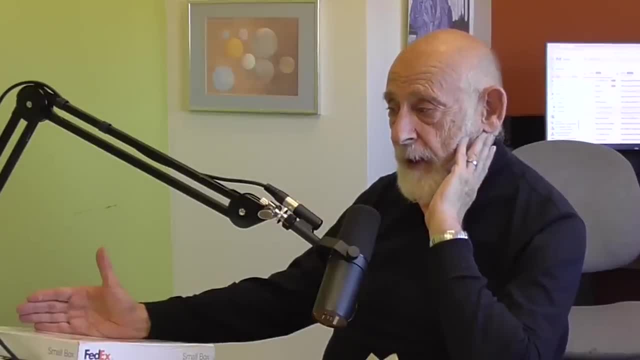 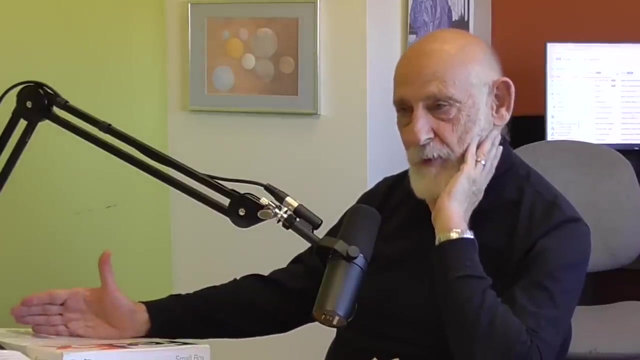 that it does, and so forth. There are three groups of people who have thought about this. There are the engineers. The engineers are incredibly smart, but they tend not to think as hard about why the thing is working as much as they do how to use it. obviously, They provided a lot. 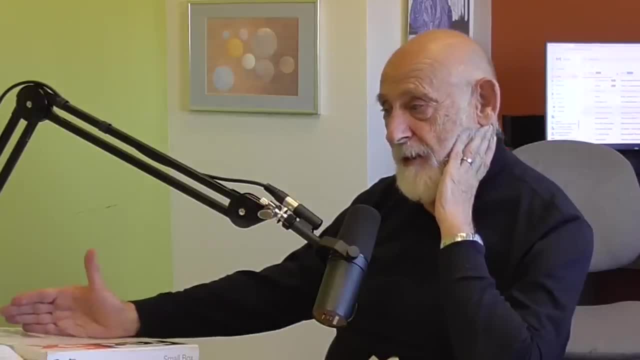 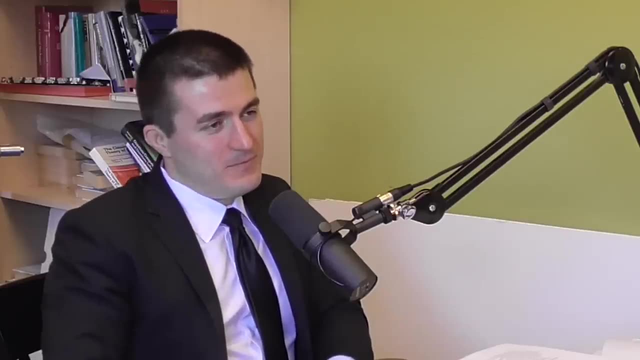 of data, and it is they who demonstrated that machine learning can work much better than you have any right to expect. The machine learning systems are systems. The systems are not too different than the kind of systems that physicists study. There's not all that. 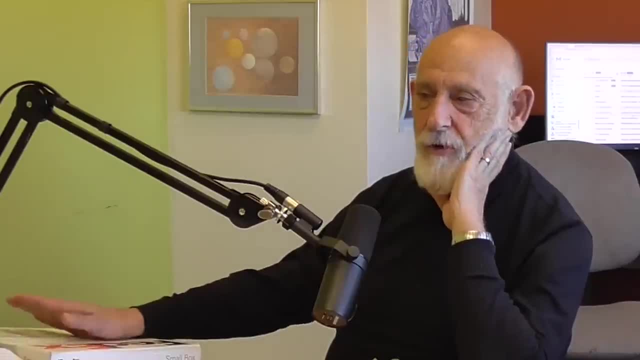 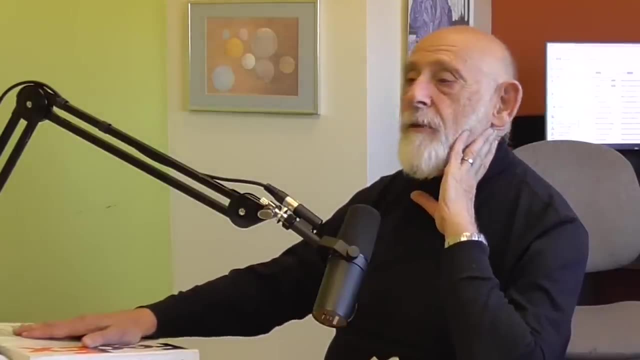 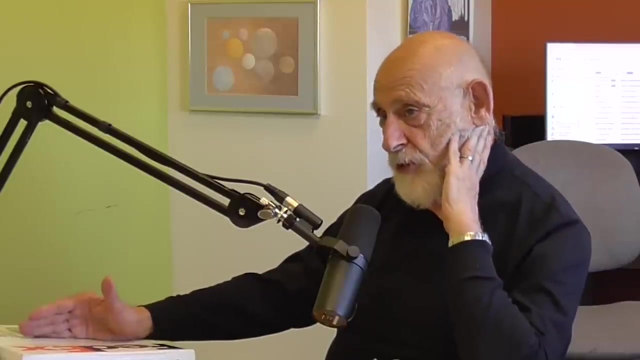 much difference in the structure of the mathematics- Physically, yes, but in the structure of the mathematics- between a tensor network designed to describe a quantum system on the one hand, and the kind of networks that are used in machine learning, More and more, I think. 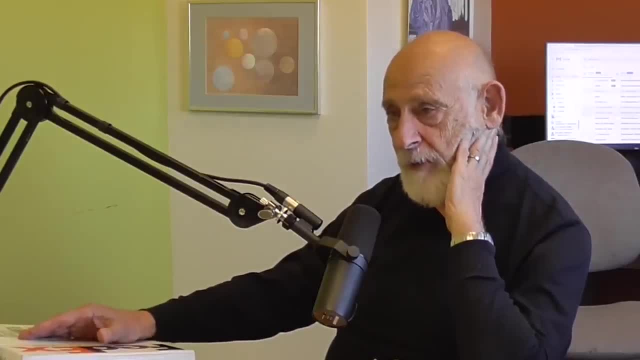 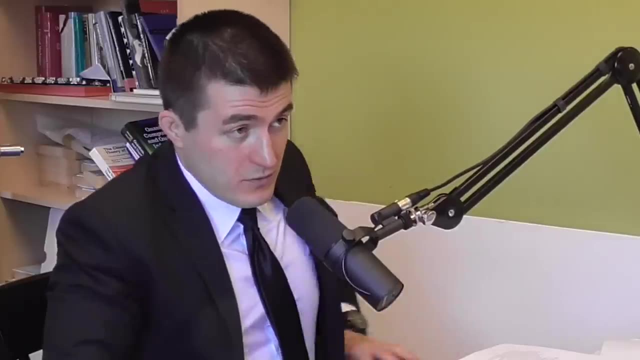 young physicists are being drawn…. …drawn to this field of machine learning. some very, very good ones. I work with a number of very good ones, not on machine learning, but on having lunch, On having lunch, Right Yeah. 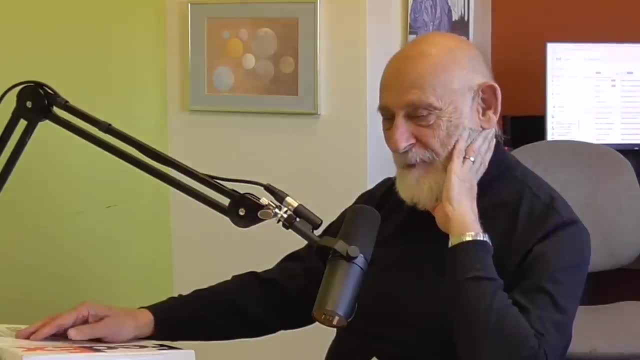 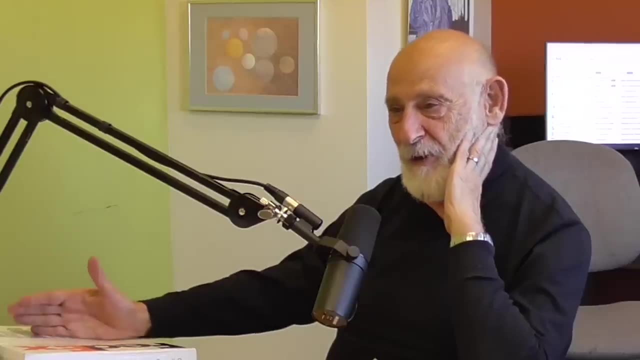 And I can tell you they are super smart. They don't seem to be so arrogant about their physics backgrounds that they think they can do things that nobody else can do. But the physics way of thinking, I think, will add great value to…. 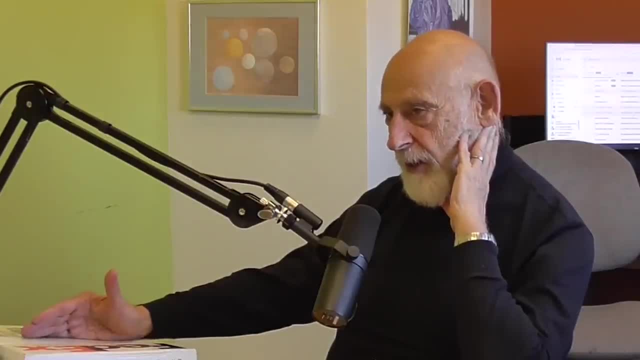 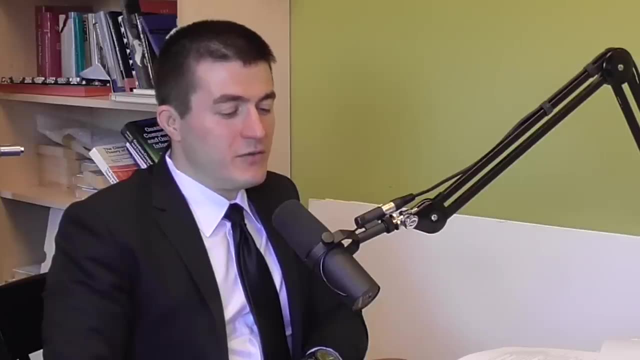 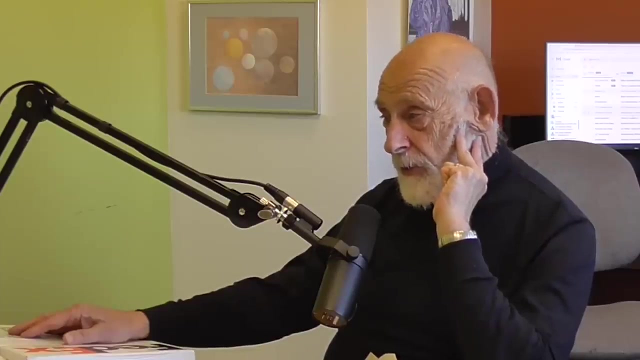 will bring value to the machine learning? I believe it will, And I think it already has. At what time scale do you think predicting the future becomes useless? In your long experience and being surprised at new discoveries- Sometimes a day, sometimes 20 years- There are things which I thought we were very far. 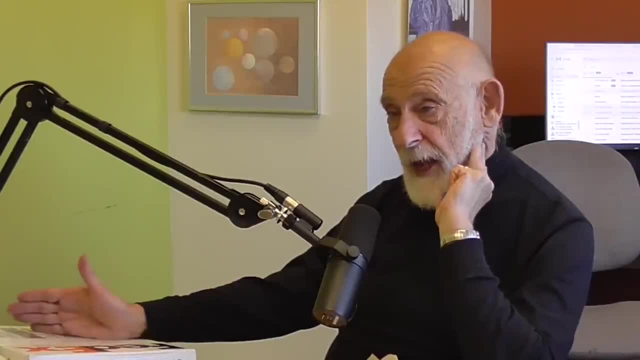 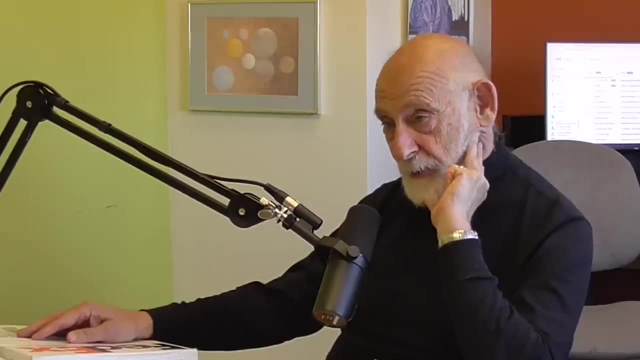 from understanding which… Practically in a snap of the fingers or a blink of the eye, suddenly became understood, Completely surprising to me. There are other things which I looked at and I said we're not going to understand these things for 500 years, in particular quantum gravity, The 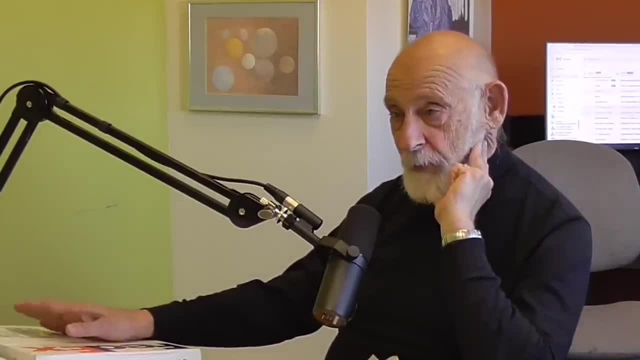 scale for that was 20 years, 25 years, And we understand a lot, and we don't understand it completely now by any means, but we… I thought it was 500 years to make any progress. It turned out to be very, very far from that. It turned out to be more like 20 or 25 years. 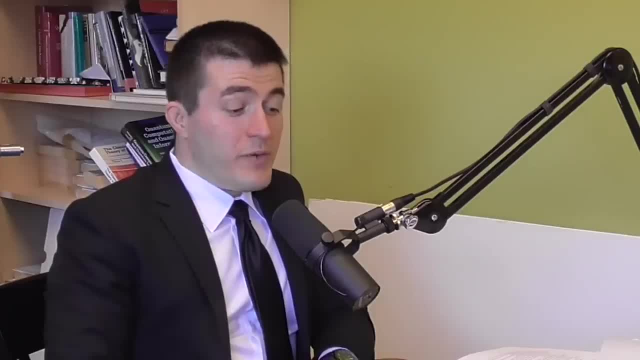 from the time when I thought it was 500 years. So, if we may, can we jump around quantum gravity? some basic ideas in physics. What is the dream of string theory? mathematically, What is the hope? Where does it come from? What problem? 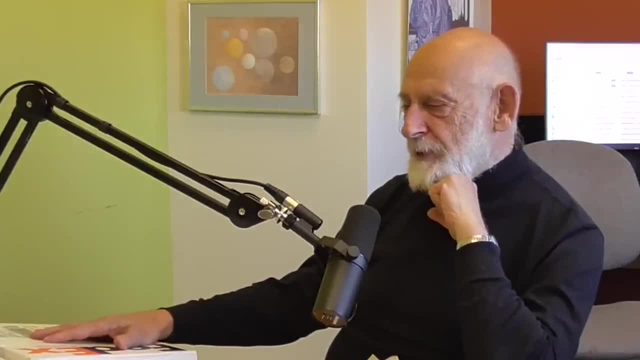 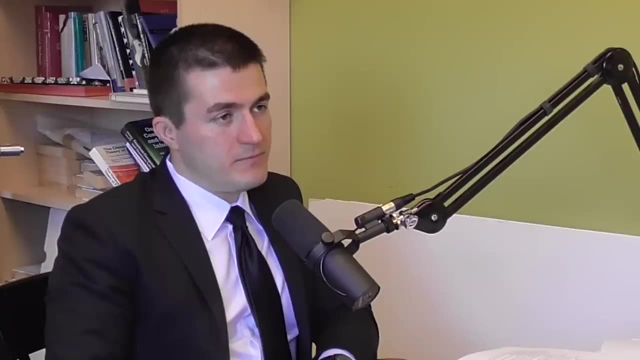 is it trying to solve? I don't think the dream of string theory is any different than the dream of fundamental theoretical physics, altogether Understandably, Understanding a unified theory of everything. Yeah, I don't like thinking of string theory as a subject unto itself with people. 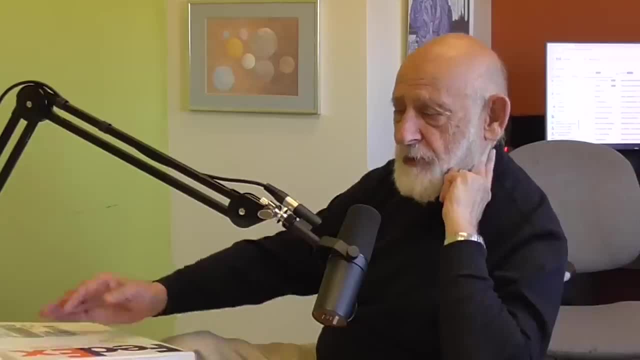 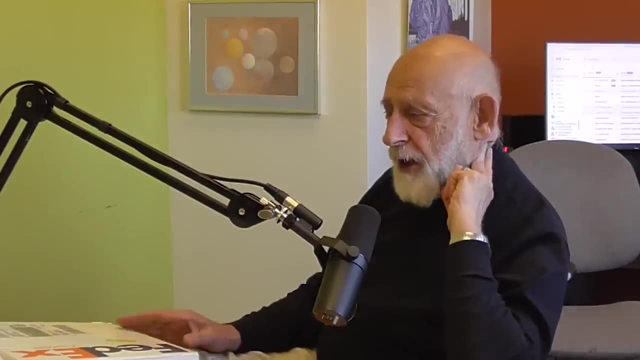 called string theorists, who are the practitioners of this thing called string theory. I much prefer to think of them as theoretical physicists trying to answer deep, fundamental questions about nature, in particular gravity, in particular gravity and its connection with quantum mechanics, and who, at the present time…. 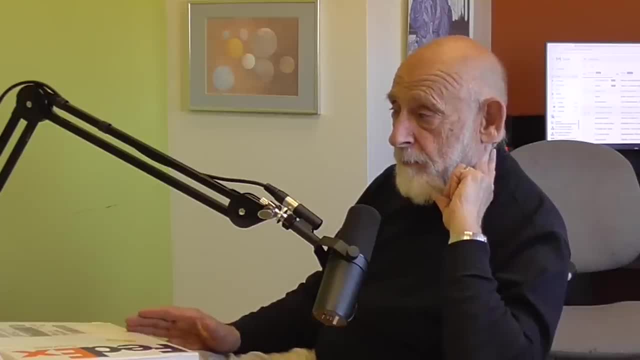 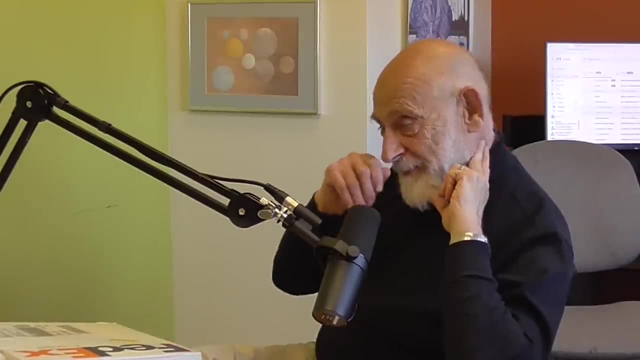 Yeah …find string theory a useful tool, rather than saying there's this subject called string theorists. I don't like being referred to as a string theorist, Yes, But as a tool is it useful to think about our nature in multiple dimensions? the 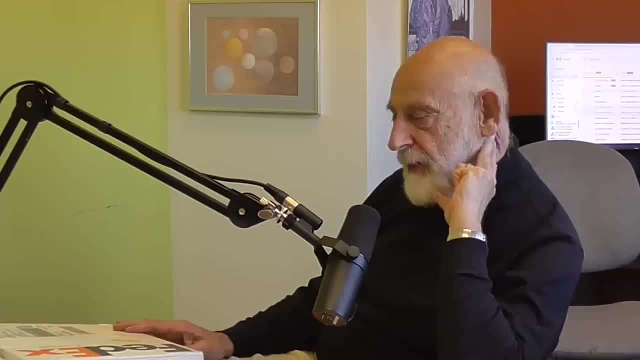 strings vibrating. I believe it is useful. I'll tell you what the main use of it has been up till now. Well, it has had a number of main uses. Originally, string theory was invented and I know that I was there. I was right at the spot where it was being invented. I was at 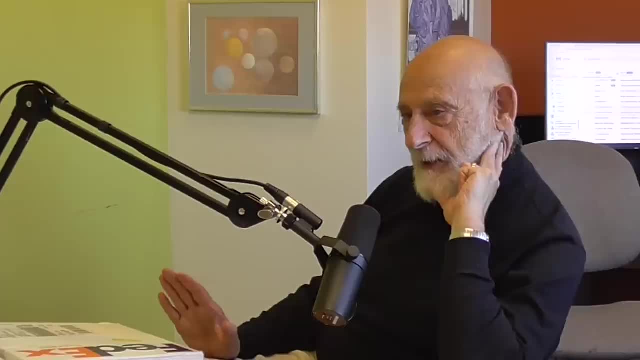 the place where it was being invented. I was at the place where it was being invented. I was at the place where it was being invented literally, And it was being invented to understand hadrons. Hadrons are subnuclear particles- protons, neutrons, mesons- And at that time, 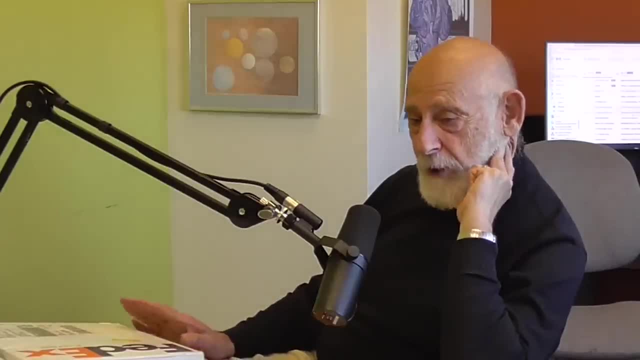 the late 60s, early 70s, it was clear from experiment that these particles called hadrons had… could vibrate, could rotate, could do all the things that a little closed string can do. And it was and is a valid and correct theory of these hadrons. It's been experimentally. tested and that is a done deal. It had a second life as a theory of gravity. the same basic mathematics, except on a very, very much smaller distance scale. The objects of gravitation are 19 orders of magnitude smaller than a particle. 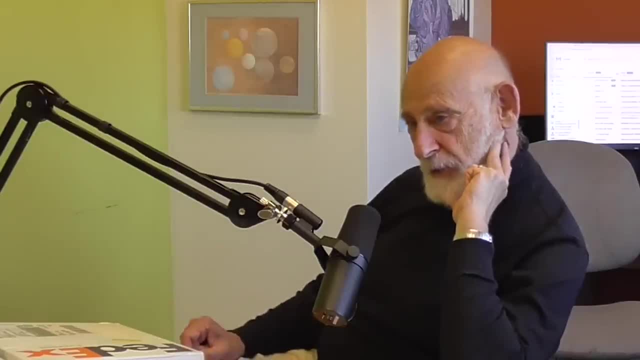 Wow, It's a proton, But the same mathematics turned up. The same mathematics turned up. What has been its value? Its value is that it's mathematically rigorous in many ways and enabled us to find mathematical structures which have both quantum mechanics and gravity. 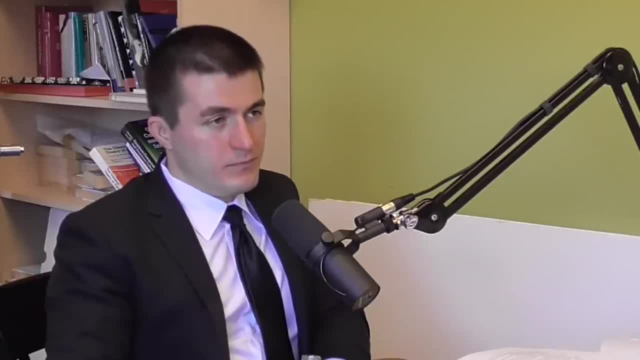 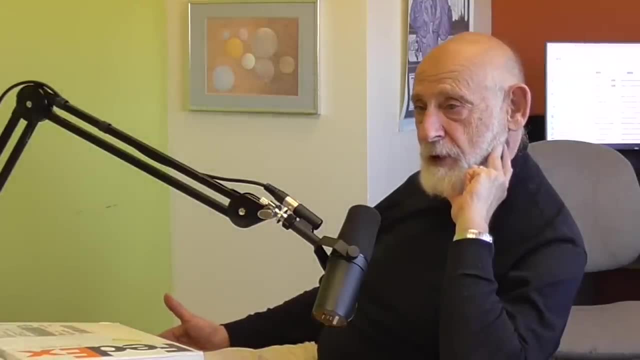 with rigor. We can test out ideas. We can test out ideas. We can't test them in the laboratory. They're 19 orders of magnitude. They're too small- the things that we're interested in. But we can test them out mathematically. 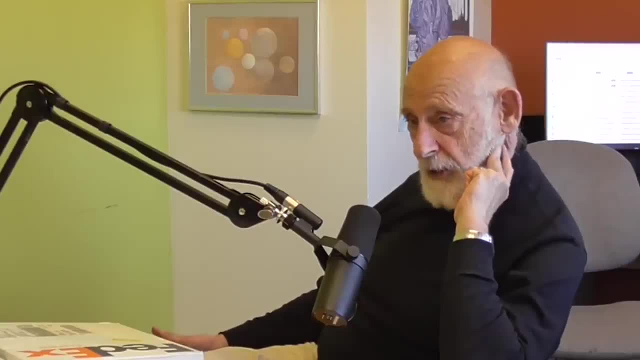 and analyze their internal consistency. By now, 40 years ago, 35 years ago or so forth, people very, very much questioned the consistency between gravity and quantum mechanics. Stephen Hawking was very famous for it, Rightly so. Now nobody questions that consistency anymore. 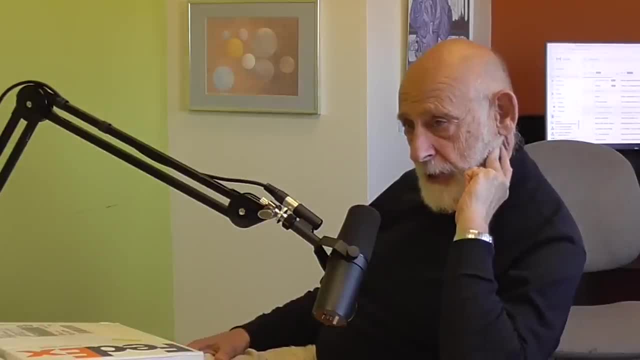 Right Now nobody questions that consistency anymore, Right? They don't, because we have mathematically precise string theories which contain both gravity and quantum mechanics in a consistent way. So it's provided that certainty that quantum mechanics and gravity can coexist. That's not a small thing, It's a very big. 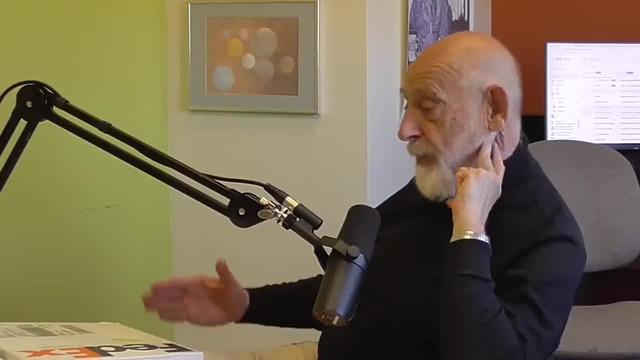 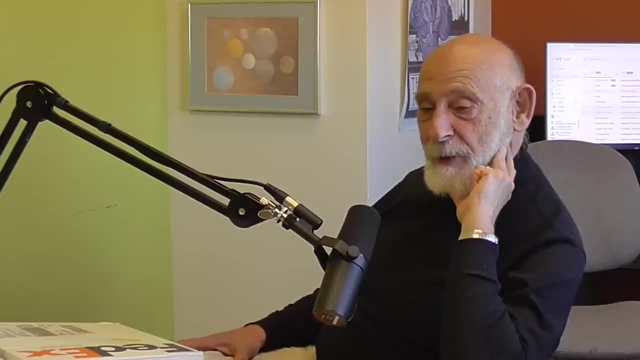 thing. It's a huge thing. Einstein would be proud Einstein. he might be appalled, I don't know. He didn't like quantum mechanics very much, Yeah, But he would certainly be struck by it, Yeah, And I think that may be, at this time, its biggest contribution to physics in illustrating 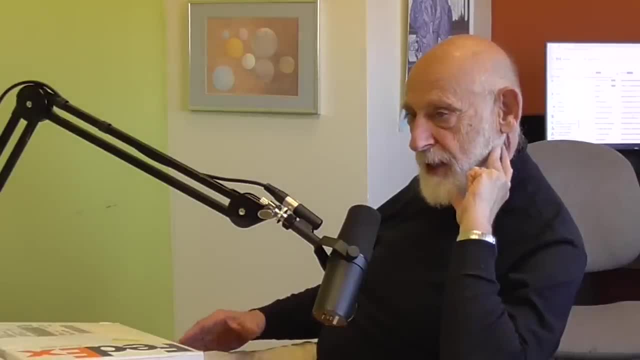 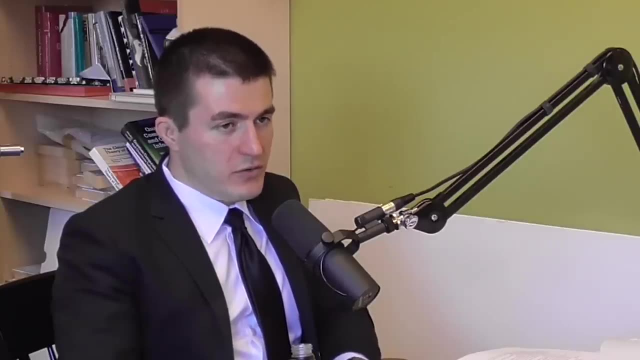 almost definitively that quantum mechanics and gravity are very closely related and not inconsistent with each other. Is there a possibility of something deeper, more profound, that still is consistent with string theory, but is deeper, that is to be found? Well, you could ask the same thing about quantum mechanics. Is there something-? 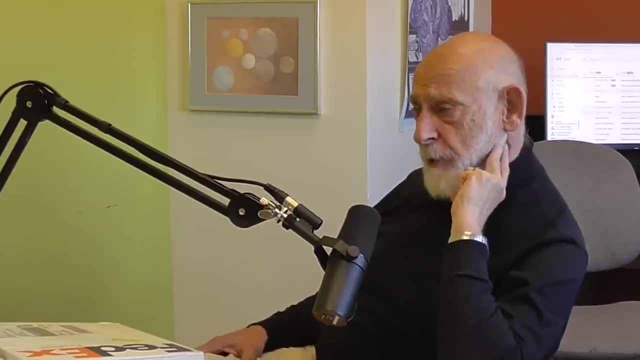 Exactly, Yeah, Yeah, I think string theory is just an example of a quantum mechanical system that contains both gravitation and quantum mechanics. So is there something underlying quantum mechanics? Perhaps something deterministic? Perhaps something deterministic? My friend Gerard Etouft, whose name you may know, he's 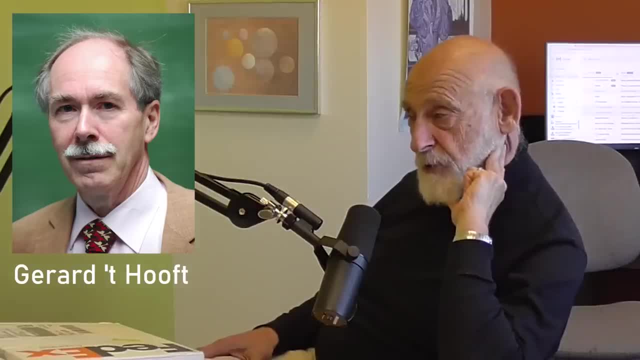 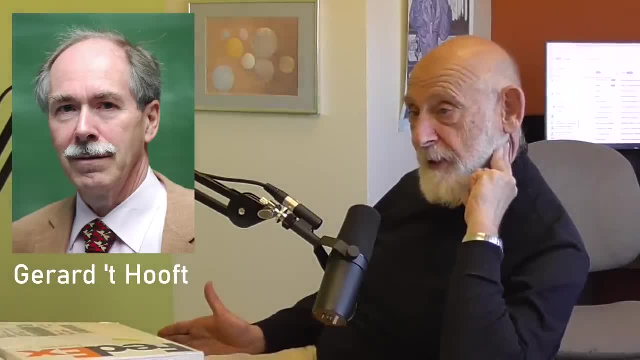 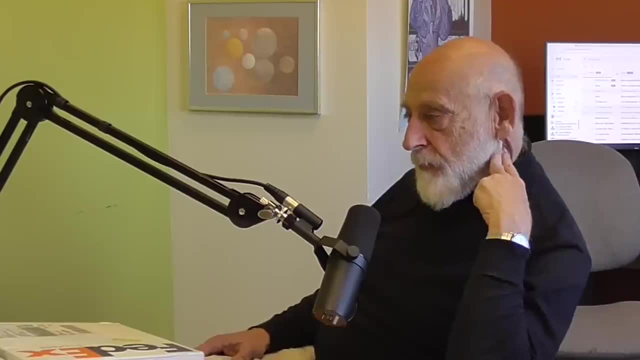 Yeah, He's a little younger than me, but he's nevertheless one of my heroes. He's a little younger than me, but he's nevertheless one of my heroes. Etouft believes that there is some sub-structure to the world which is classical in character. 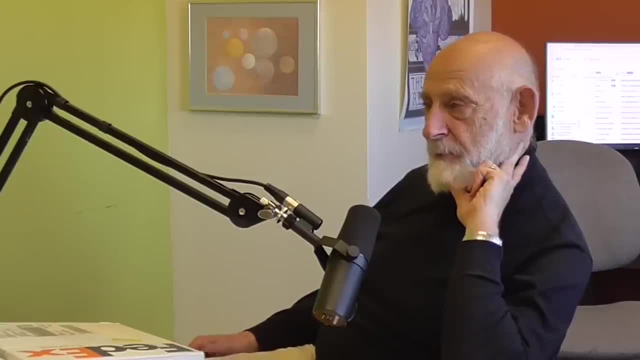 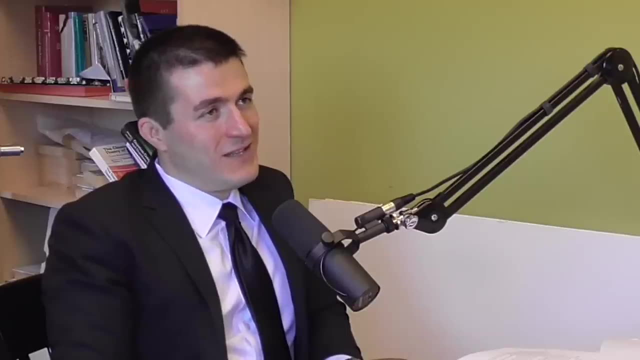 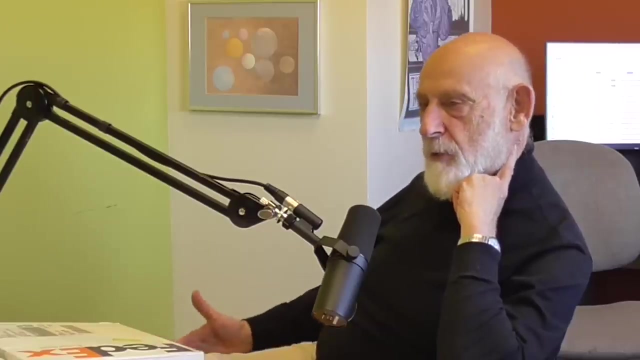 deterministic in character, which somehow, by some mechanism that he has a hard time spelling out, emerges. emerges as quantum mechanics? I don't. The wave function is somehow emergent, The wave function. not just the wave function, but the whole mech and the whole thing. 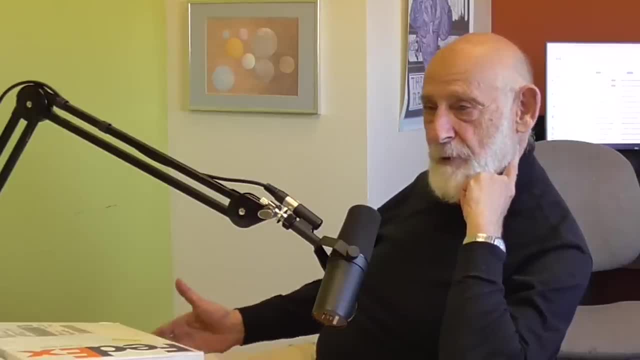 that goes with quantum mechanics. uncertainty, entanglement, all these things are emergent. So you think quantum mechanics is the bottom of the well Is the. Here, I think, is where you have to be humble, Here's where humility comes. 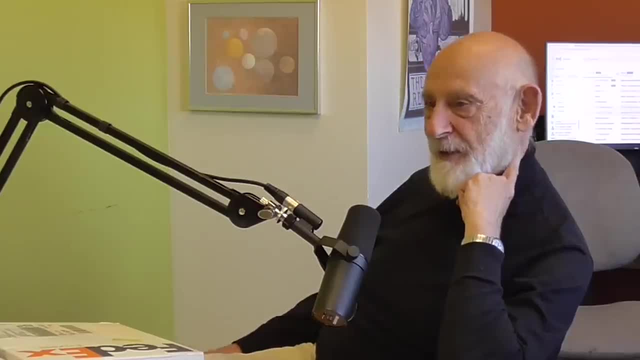 I don't think anybody should say anything is the bottom of the well at this time. I think we can reasonably say. I can reasonably say: when I look into the well, I can't see past quantum mechanics. I don't see any reason for there to be anything. 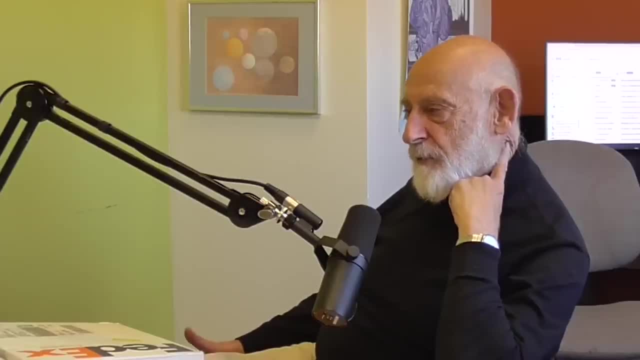 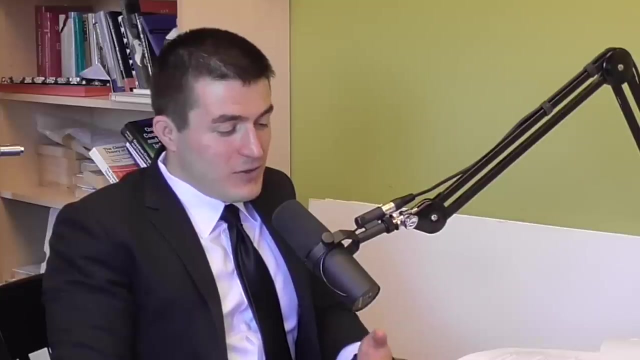 beyond quantum mechanics. I think Etouft has asked very interesting and deep questions. I don't like his answers. Well, again, let me ask if we look at the deep, at the deepest nature of reality, whether is deterministic or when observed as probabilistic. 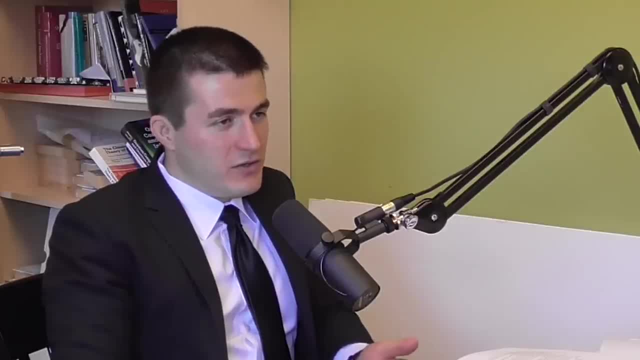 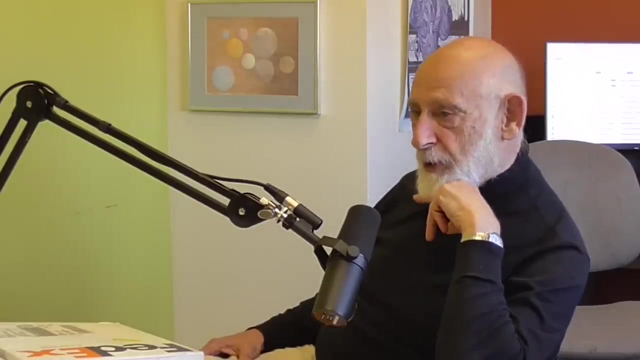 what does that mean for our human level of ideas of free will? Is there any connection whatsoever from this perception, perhaps illusion, of free will that we have and the fundamental nature of reality? The only thing I can say is: I am puzzled by that as much as you are. 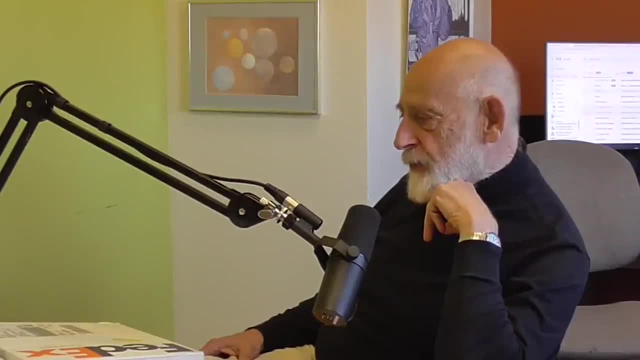 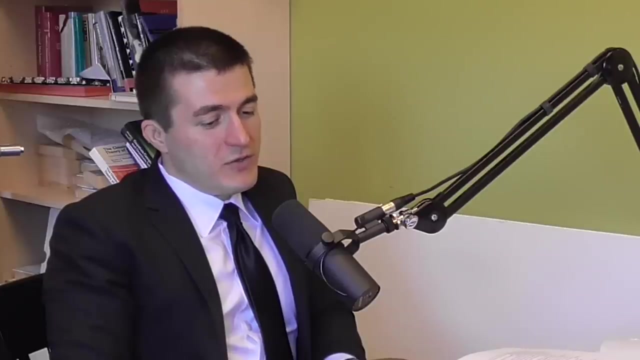 The illusion of it, The illusion of consciousness, the illusion of free will, the illusion of self. Does that connect to? How can a physical system do that? And I am as puzzled as anybody. There's echoes of it in the observer effect. 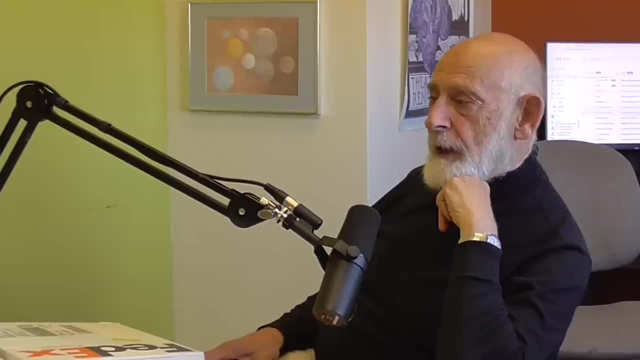 Yeah, So do you understand what it means to be an observer? I understand it at a technical level. An observer is a system with enough degrees of freedom that it can record information and which can become entangled with the thing that it's measuring. 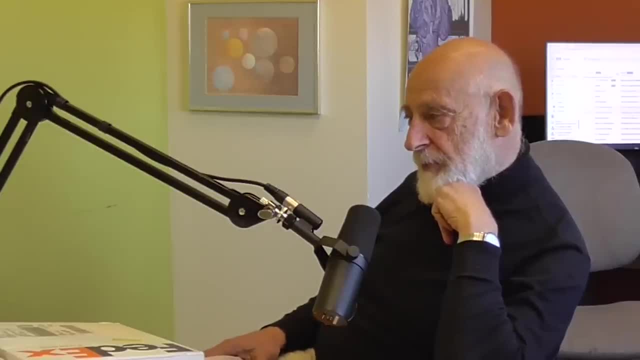 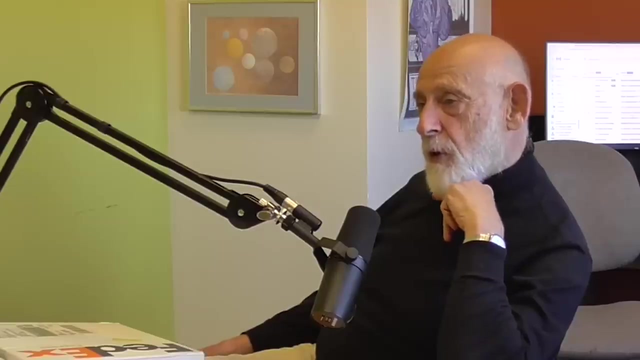 Entanglement is the key. When a system, which we call an apparatus or an observer same thing, interacts with the system that it's observing, it doesn't just look at it, It becomes physically entangled with it, And it's that entanglement which we call an observation or a measurement. 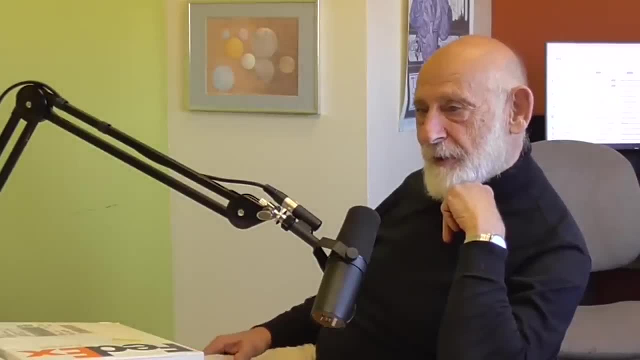 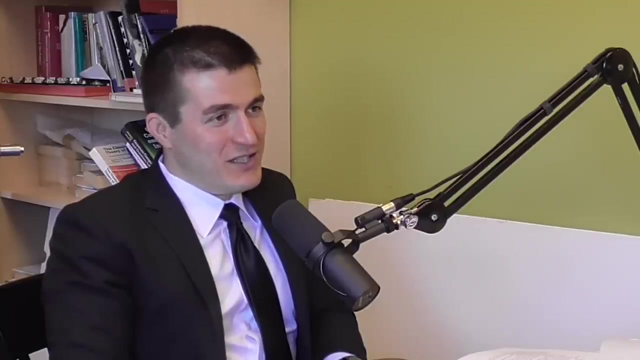 Now, does that satisfy me personally as an observer? No, Yes and no. I find it very satisfying that we have a mathematical representation of what it means to observe a system. You are observing stuff right now. Yeah, The conscious level, Right. 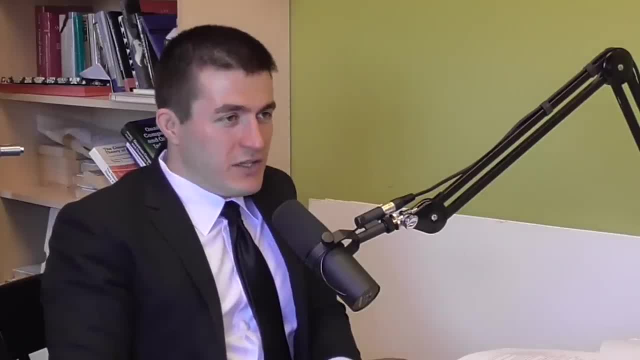 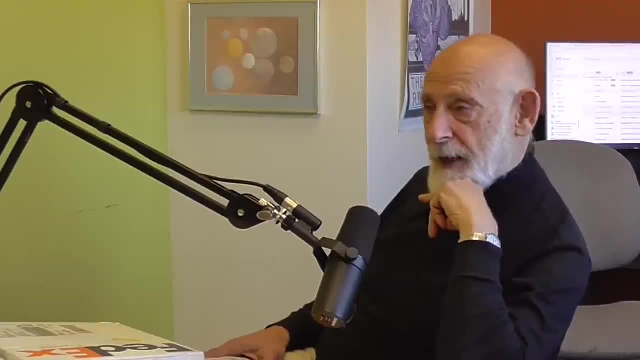 Do you think there's echoes of that kind of entanglement in our macro scale? Yes, absolutely For sure. We're entangled with Quantum, mechanically entangled with everything in this room. If we weren't, then we would just. 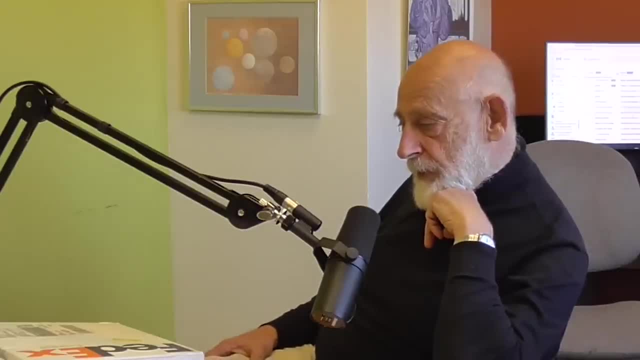 Well, we wouldn't be observing it. But on the other hand, you can ask: am I really comfortable with it? And I'm uncomfortable with it, in the same way that I can never get comfortable with five dimensions. My brain isn't wired for it. 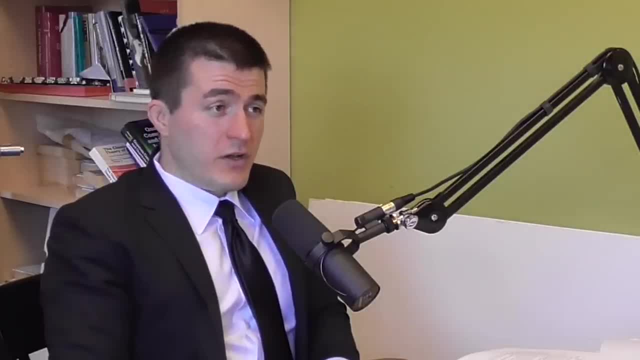 Are you comfortable with four dimensions A little bit more, because I can always imagine the fourth dimension is time. So the arrow of time. are you comfortable with that arrow? Do you think time is an emergent phenomenon Or is it fundamental to nature? 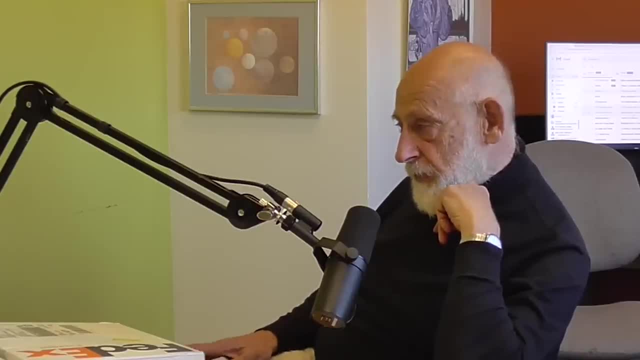 That is a big question. in physics right now, All the physics that we do, or at least that the people that I am comfortable with talking to, my friends, my friends- we all ask the same question that you just asked: Space. we have a pretty good idea: is emergent. 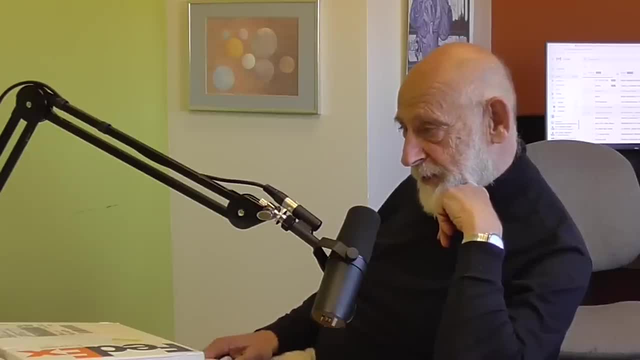 And it emerges out of entanglement and other things. Time always seems, It seems to be built into our equations as just what Newton pretty much would have thought. Newton, modified a little bit by Einstein, would have called time. And mostly in our equations it is not emergent. 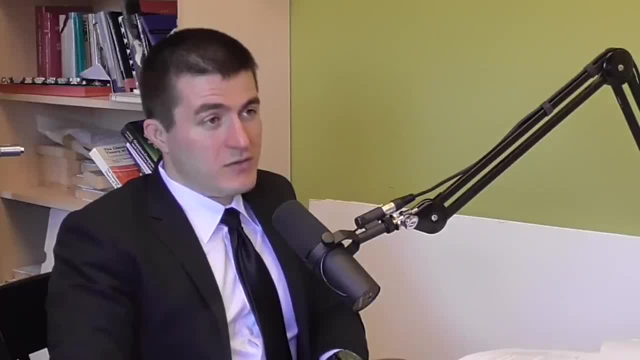 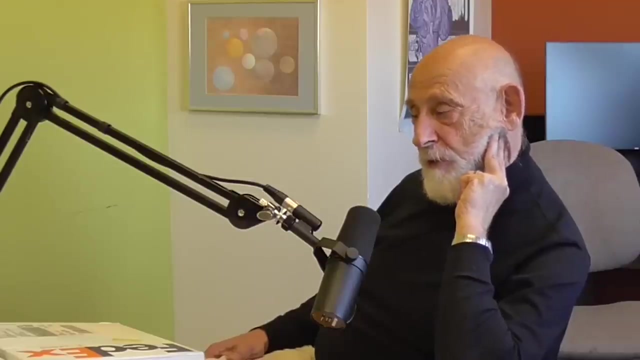 Time in physics is completely symmetric: forward and backward, Right it's symmetric, So you don't really need to think about the arrow of time. for most physical phenomena, Most microscopic phenomena, no, It's only when the phenomena involves systems which are big enough for thermodynamics to become important. 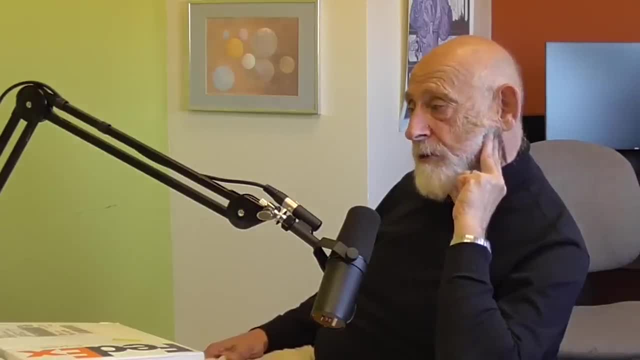 For entropy to become important. For a small system, entropy is not a good concept And entropy is something which emerges out of large numbers. It's a probabilistic idea, it's a statistical idea and it's a thermodynamic idea. The thermodynamics requires lots and lots and lots of little substructures. okay, 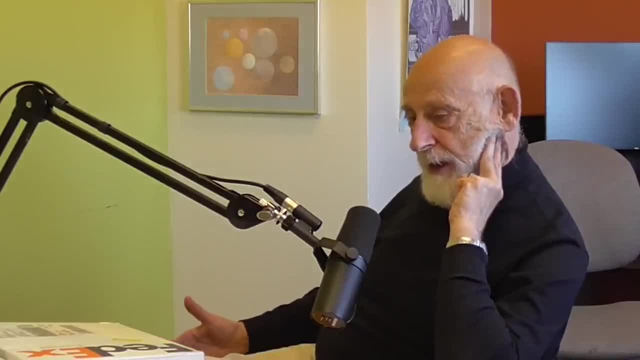 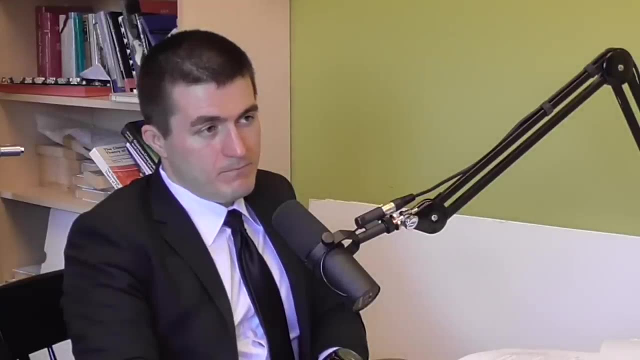 So it's not until you emerge at the thermodynamic level that there's an arrow of time. Do we understand it? Yeah, I think we understand it better than most people think they understand it. Most people say they think we understand it. Yeah, I think we understand it. 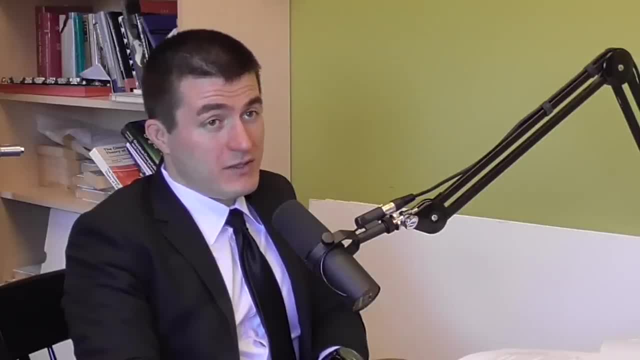 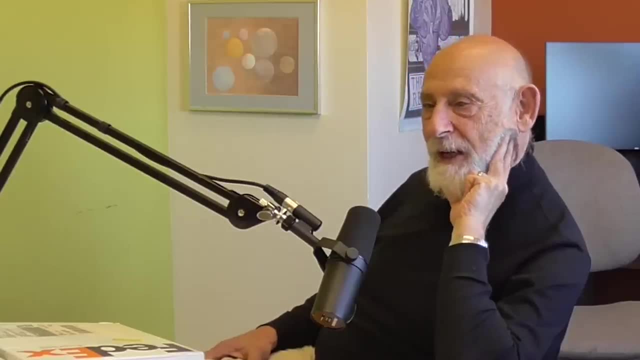 It's just a statistical idea. You mean like second law, thermodynamics, entropy and so on. Yeah, pick a pack of cards and you fling it in the air and you look what happens to it. It gets random. We understand it. 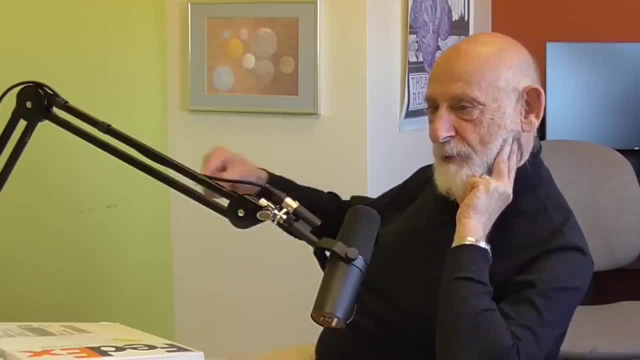 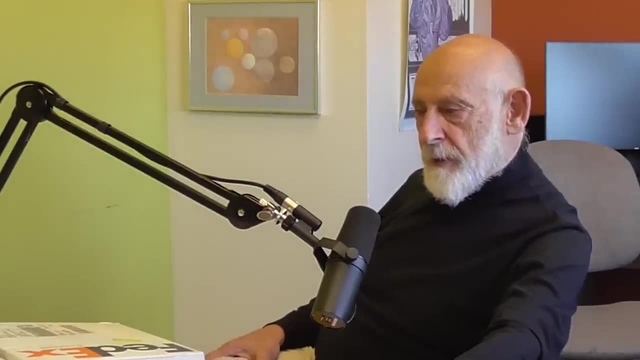 It doesn't go from random to simple. It goes from simple to random, But do you think it ever breaks down? What I think you can do is, in a laboratory setting, you can take a system which is somewhere intermediate between being small and being large and make it go backward. 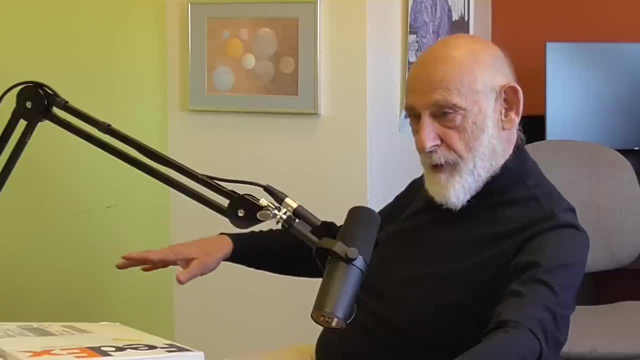 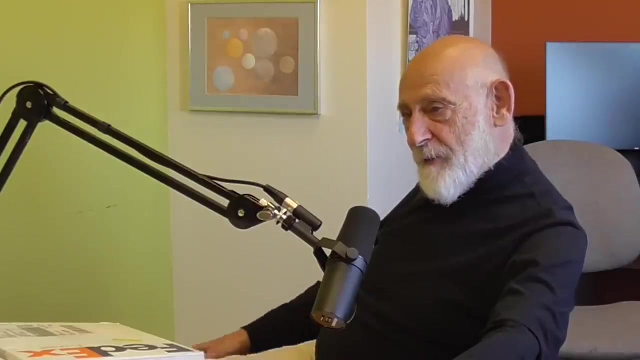 A thing which looks like It only wants to go forward because of statistical, mechanical reasons, because of the second law, you can very, very carefully manipulate it to make it run backward. I don't think you can take an egg- Humpty Dumpty- who fell on the floor and reverse that. 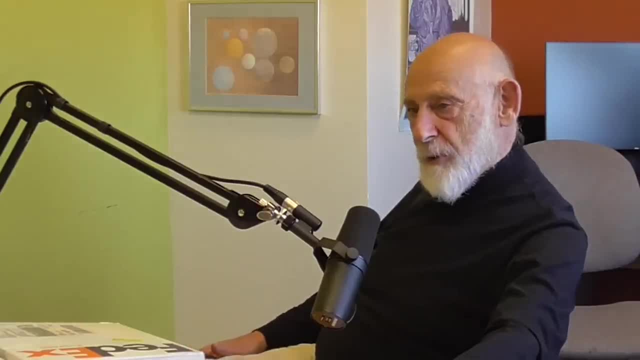 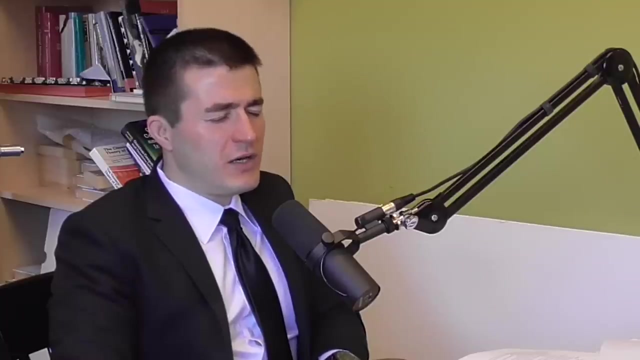 But you can, in a very controlled situation. you can take systems which appear to be evolving statistically toward randomness, stop them, reverse them And make them go back. What's the intuition behind that? How do we do that? How do we reverse it? 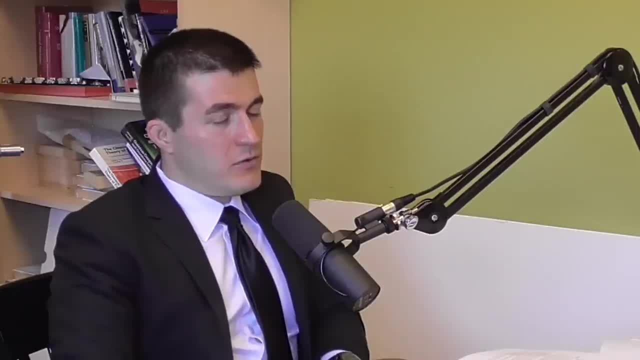 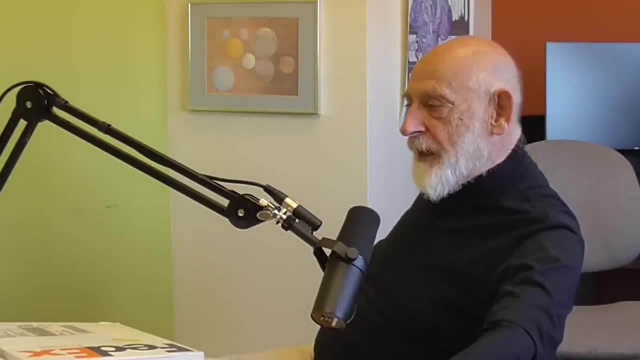 You're saying a closed system? Yeah, pretty much closed system. yes, Did you just say that time travel is possible? No, I didn't say time travel is possible. I said you can make a system go backward In time. You can make it go back. 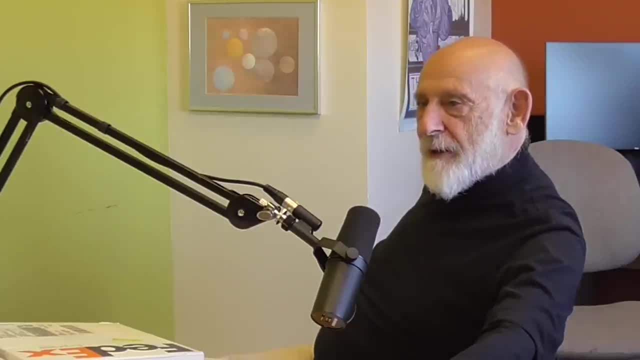 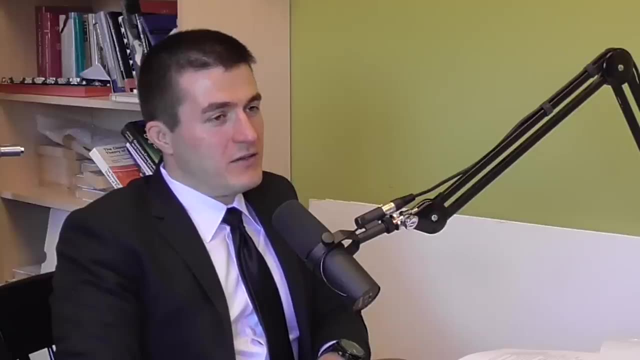 You can make it reverse its steps. You can make it reverse its trajectory. Yeah, How do we do it? What's the intuition there? Is it just a fluke, A thing that we can do at a small scale in the lab that doesn't have? 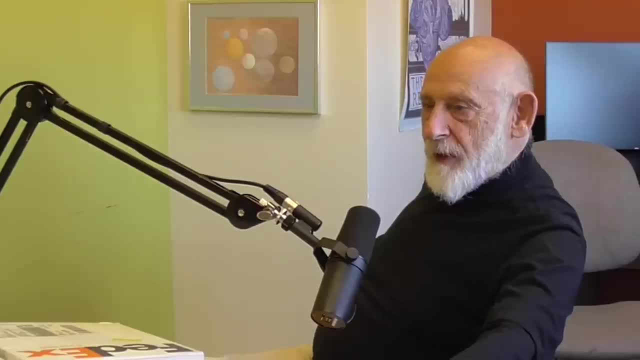 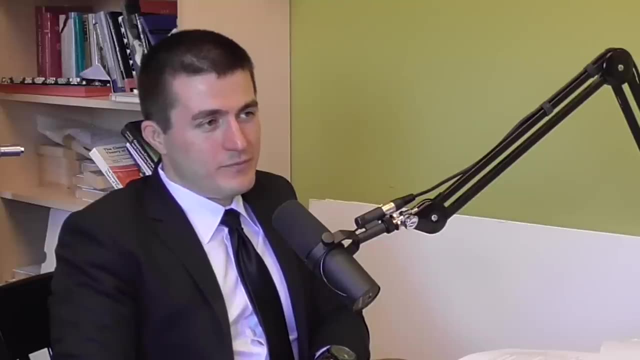 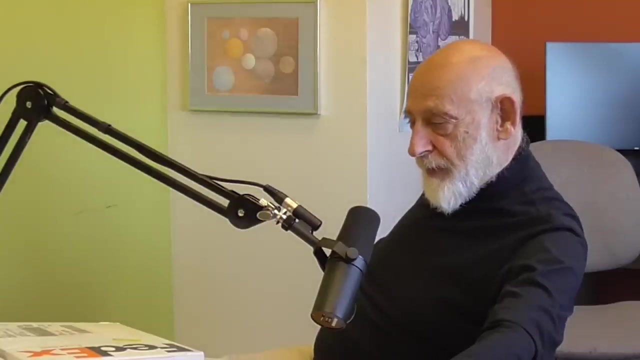 Well, what I'm saying is: you can do it on a little bit better than a small scale. You can certainly do it with a simple small system. Small systems don't have any sense of the arrow of time Atoms. Atoms are no sense of an arrow of time. 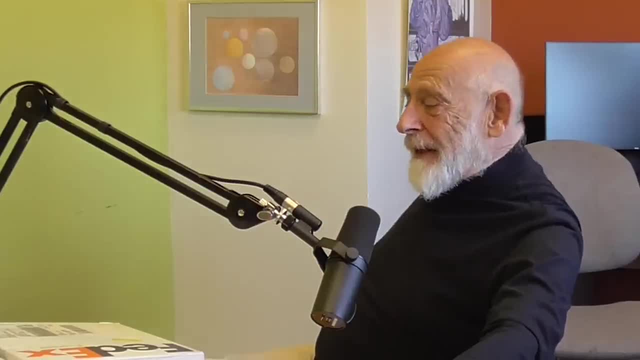 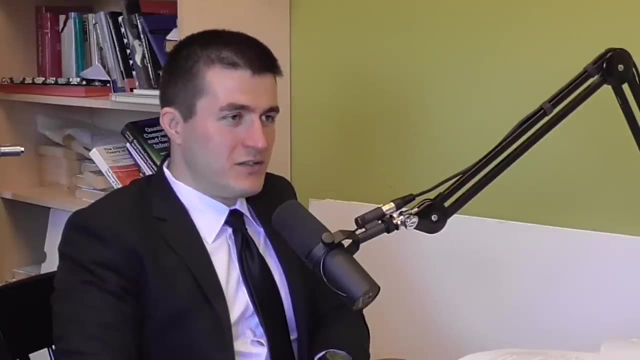 They're completely reversible. It's only when you have. The second law of thermodynamics is the law of large numbers. So you can break the law, because it's not deterministic law. You can break it, but it's hard, It requires great care. 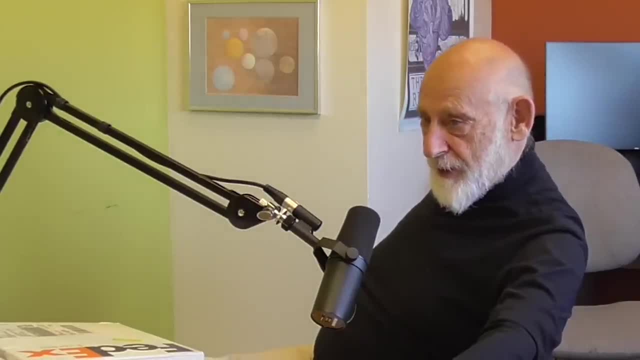 The bigger the system is, the more care, the harder it is. You have to overcome what's called chaos, And that's hard And it requires more and more precision. For 10 particles. you might be able to do it with some effort. 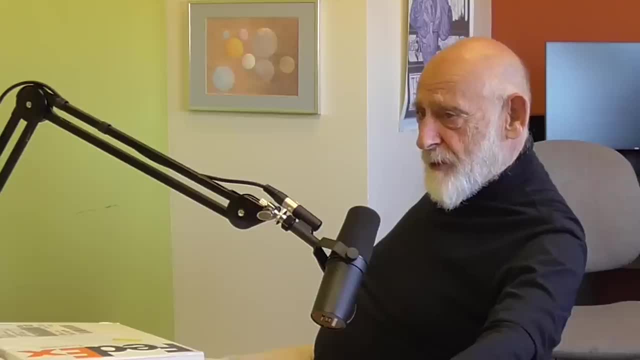 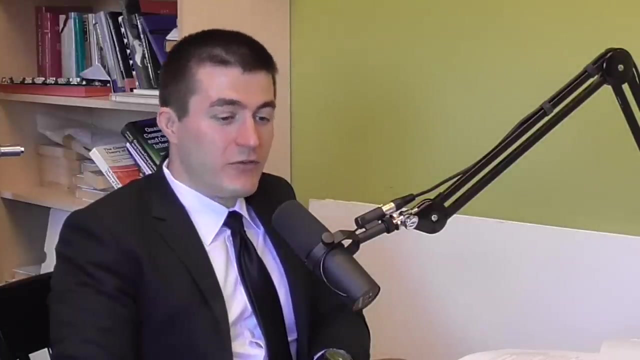 For 100 particles. it's really hard For 1,000 or 1,000 particles, forget it. But not for any fundamental reason, just because it's technologically too hard to make the system go backward. So no time travel for engineering reasons. 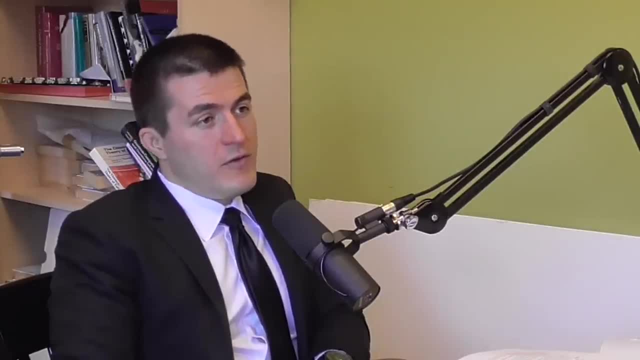 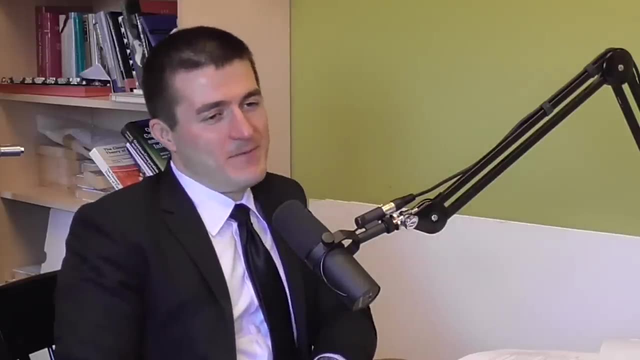 No, no, no, no. What is time travel? Time travel to the future, That's easy. You just close your eyes, go to sleep and you wake up in the future. Yeah, yeah, A good nap gets you there, yeah. 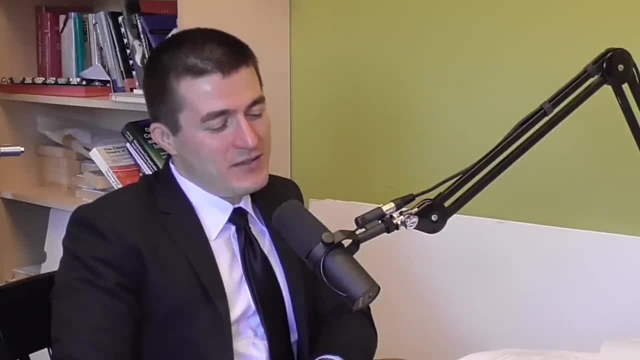 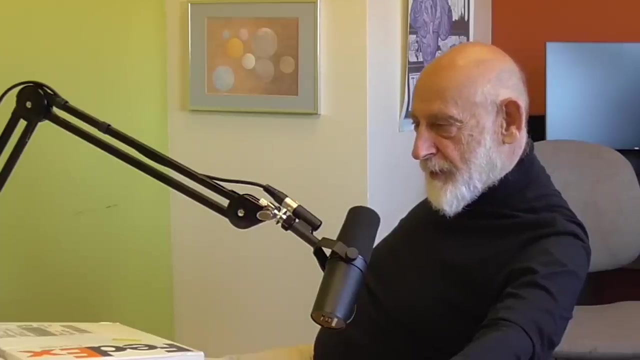 Yeah, A good nap gets you there right. What happens in reversing the second law of thermodynamics, going backward in time for anything that's human scale, is a very difficult engineering effort. I wouldn't call that time travel because it gets too mixed up with what science fiction calls time travel. 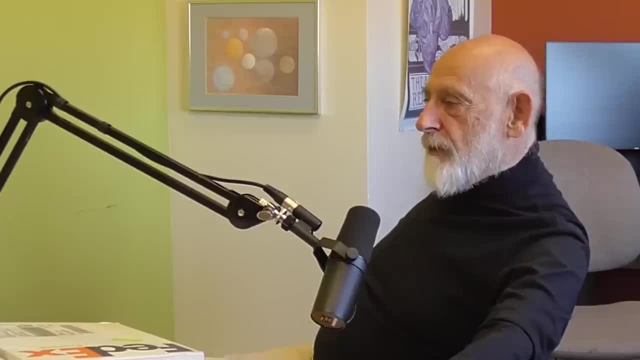 Right. This is just the ability to reverse a system. You take the system and you reverse the direction of motion. You reverse the direction of every molecule in it. You can do it with one molecule If you find a particle moving in a certain direction. 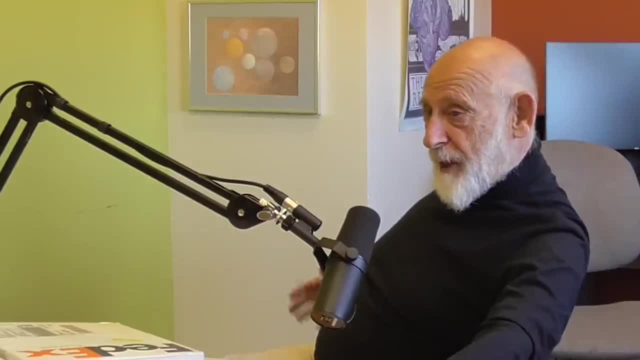 let's not say a particle, a baseball. you stop it dead and then you simply reverse its motion. In principle, that's not too hard And it'll go back along its trajectory in the backward direction, Just running the program backwards. 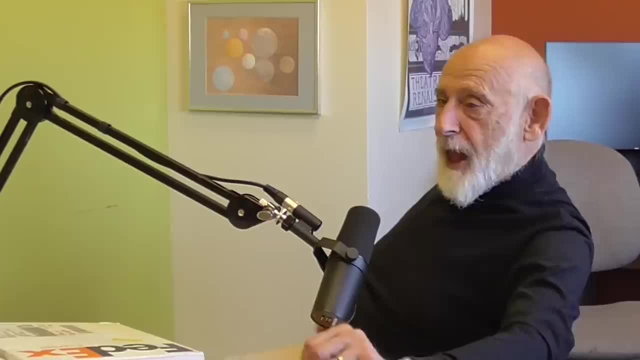 Running the program backward. Yeah, Okay, If you have two baseballs colliding, well, you can do it, but you have to be very, very careful to get it to the other side. You have to get it just right If you have 10 baseballs. 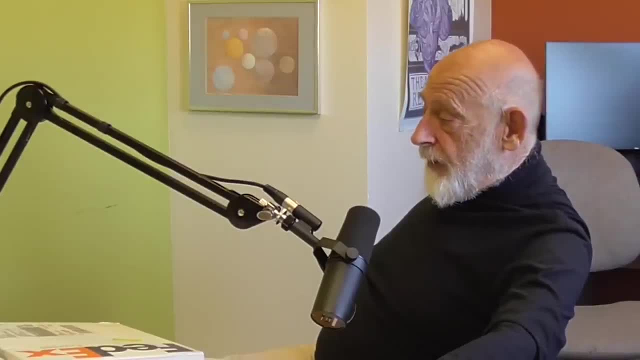 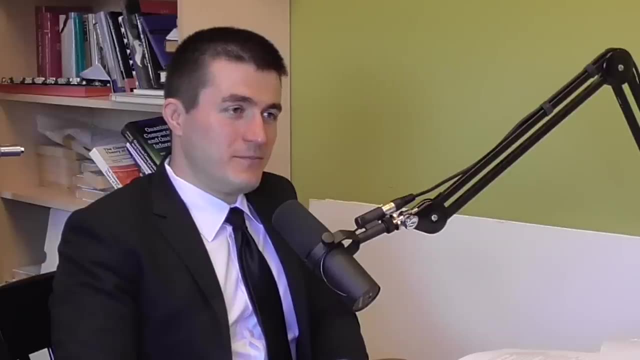 really, really, or better yet, 10 billiard balls on an idealized frictionless billiard table. Okay, So you start the balls all in a triangle, right, Yep, And you whack them- Yep, Depending on the game you're playing. 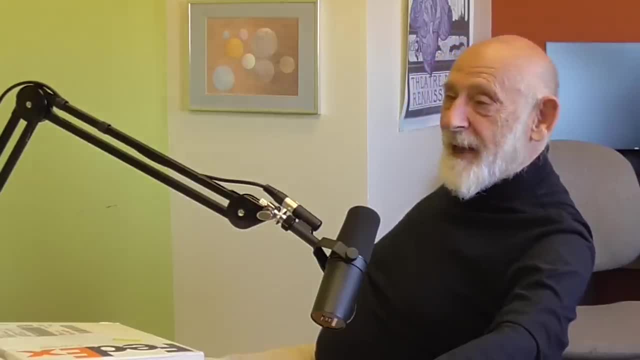 you either whack them or you're really careful, but you whack them And they go flying off in all possible directions. Yeah, Okay, Try to reverse that. Try to reverse that. Imagine trying to take every billiard ball, stopping it dead at some point. 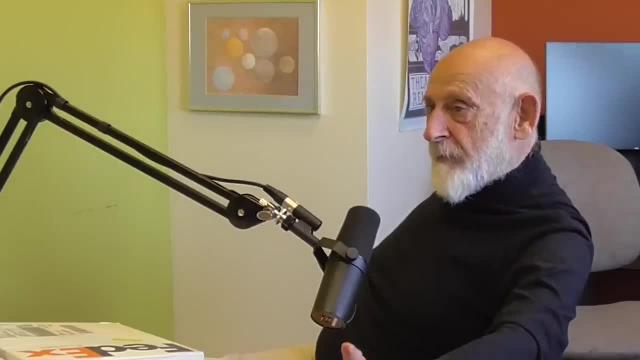 and reversing its motion so that it was going in the opposite direction. If you did that with tremendous care, it would reassemble itself back into the triangle. Okay, That is a fact, And you can probably do it with two billiard balls. 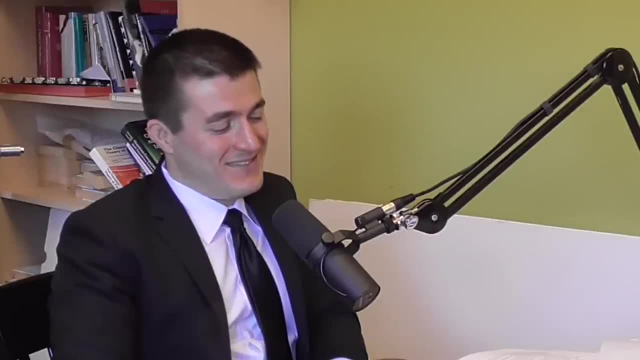 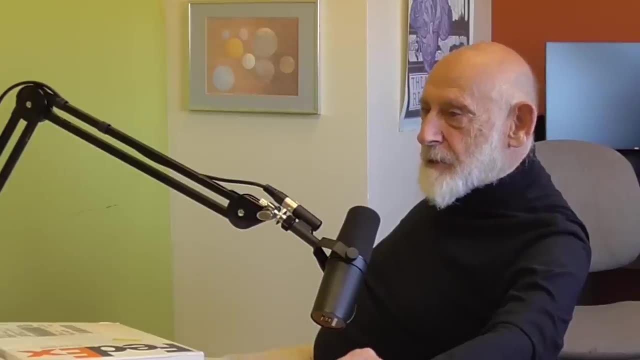 maybe with three billiard balls if you're really lucky. But what happens is, as the system gets more and more complicated, you have to be more and more precise, not to make the tiniest error, because the tiniest errors will get magnified. 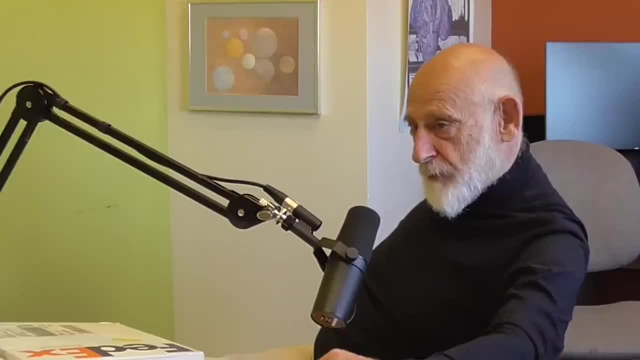 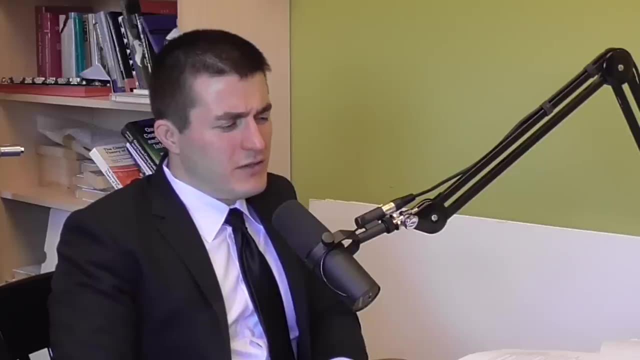 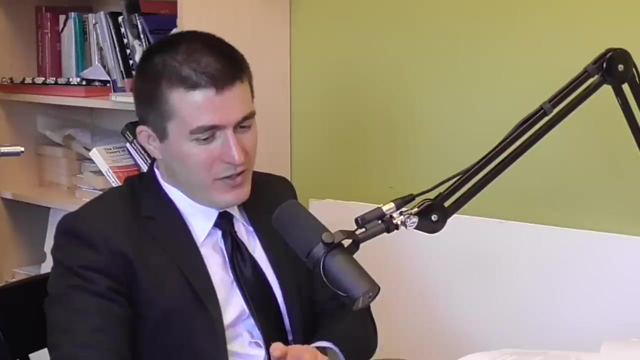 and you'll simply not be able to do the reversal. So, yeah, but I wouldn't call that time travel. Yeah, that's something else, But if you think of it, it just made me think. if we think the unrolling of state that's happening as a program. 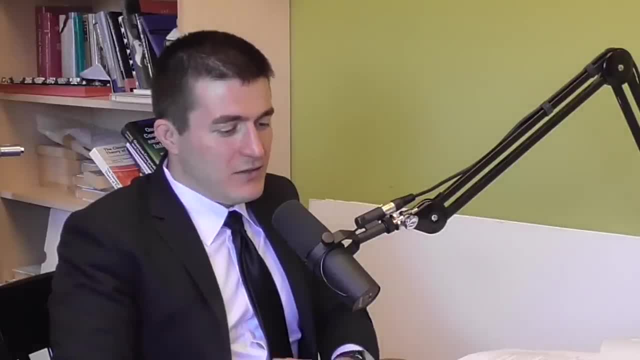 if we look at the world. so the idea of looking at the world as a simulation, as a computer. But it's not a computer, It's just a single program. A question arises that might be useful: How hard is it to have a computer that runs the universe? 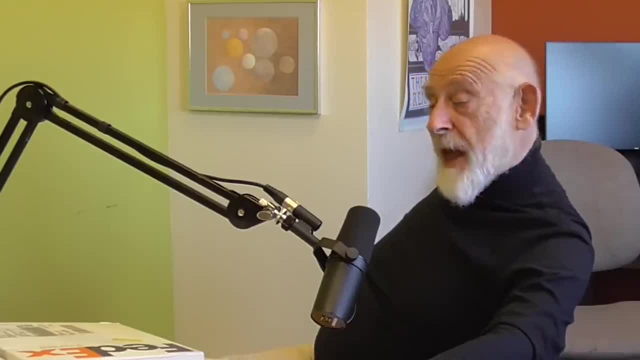 Okay, so there are mathematical universes that we know about. One of them is called anti-de Sitter space, where we, we, and it's quantum mechanics. Well, I think we could simulate it in a computer, in a quantum computer. 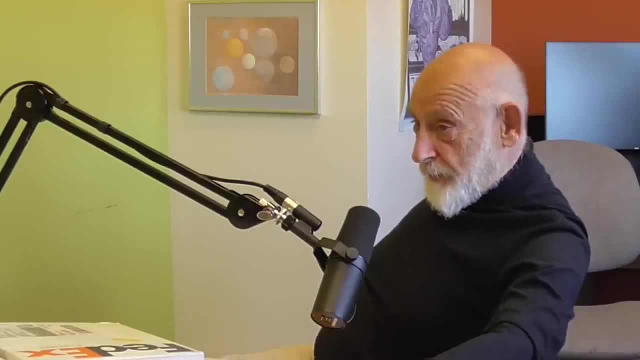 Classical computer. all you can do is solve its equations. You can't make it work like the real system. If we could build a quantum computer, a big enough one, a robust enough one, we could probably simulate a universe, a small version of an anti-de Sitter universe. 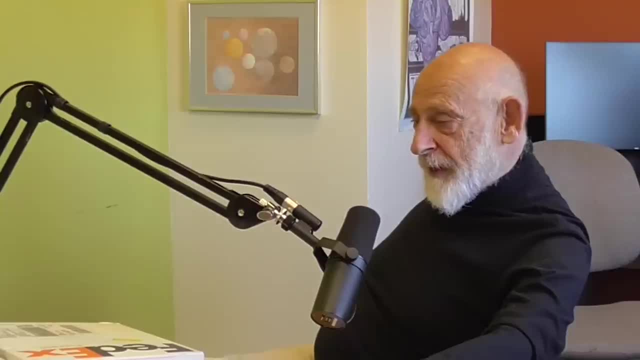 Anti-de Sitter is a kind of cosmology. Okay, so I think we know how to do that. The trouble is, the universe that we live in is not the anti-de Sitter geometry, It's the de Sitter geometry, And we don't really understand its quantum mechanics at all. So at the present time, I would say we wouldn't have the vaguest idea how to simulate a universe similar to our own. No, we could ask: could we build in the laboratory a small version, a quantum mechanical version, the collection of quantum computers entangled? 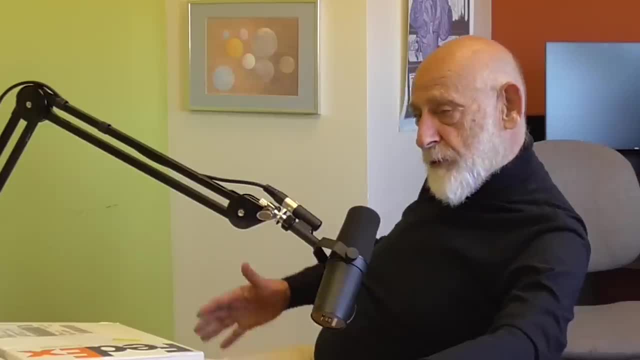 and coupled together, which would reproduce the phenomena that go on in the universe, even on a small scale. Yes, if it were anti-de Sitter space. No, if it's de Sitter space. Can you slightly describe de Sitter space? 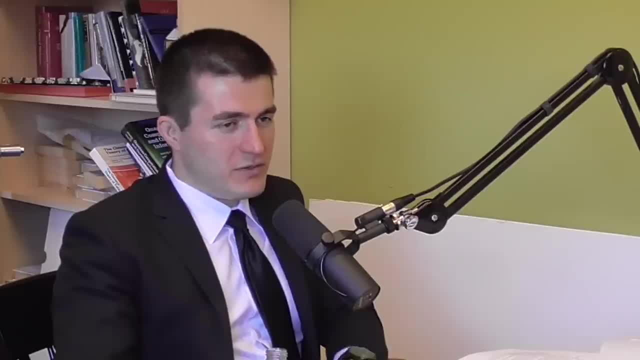 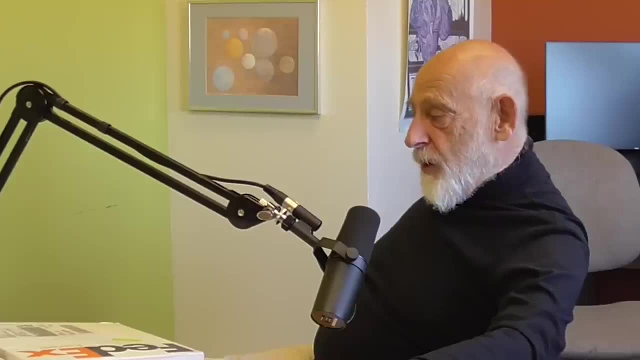 and anti-de Sitter space. Yeah, What are the geometric properties of- They differ. They differ by the sign of a single constant called the cosmological constant. One of them is negatively curved, The other is positively curved, The anti-de Sitter space. 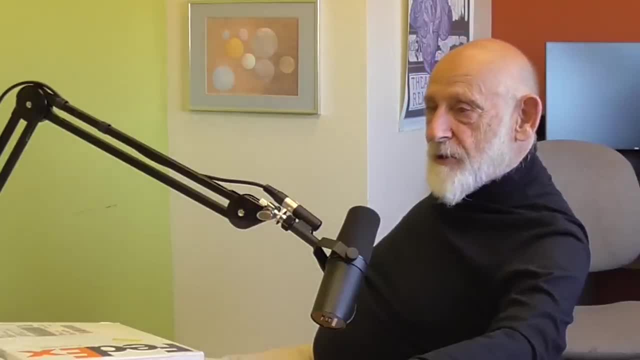 which is the negatively curved one. you can think of as an isolated system in a box with reflecting walls. You could think of it as a quantum mechanical system, isolated in an isolated environment. Mm-hmm, The Sitter space is the one we really live in. 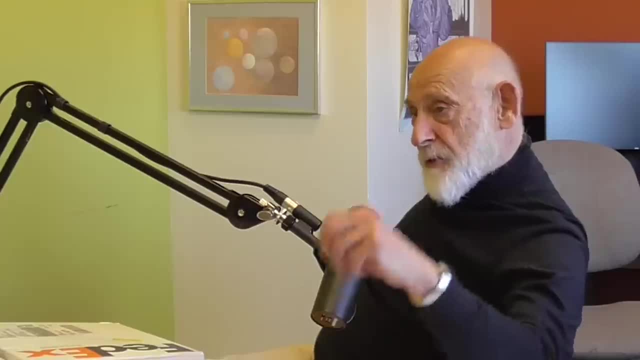 and that's the one that's exponentially expanding. Exponential expansion, dark energy, whatever we wanna call it. And we don't understand that mathematically Do we understand- Not everybody would agree with me, but I don't understand. I mean they would agree with me. 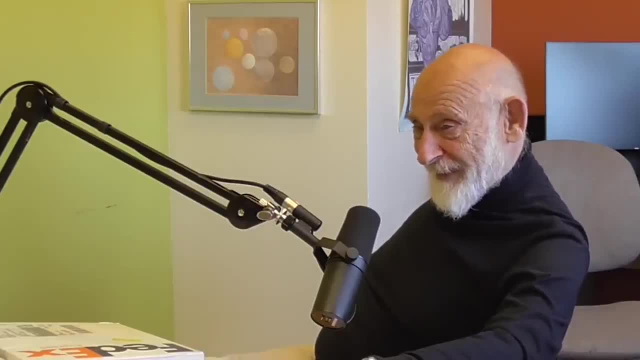 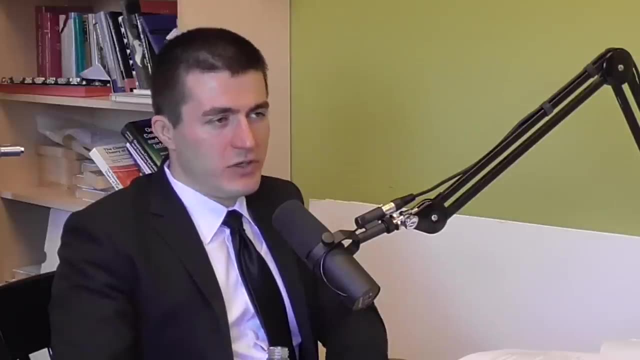 they definitely would agree with me that I don't understand it. What about? is there an understanding of the birth, the origin- No. The Bing Bang? No, no. So does one come with the other Theories? there are theories. 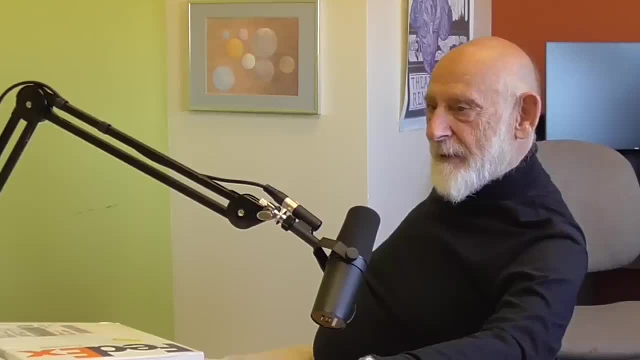 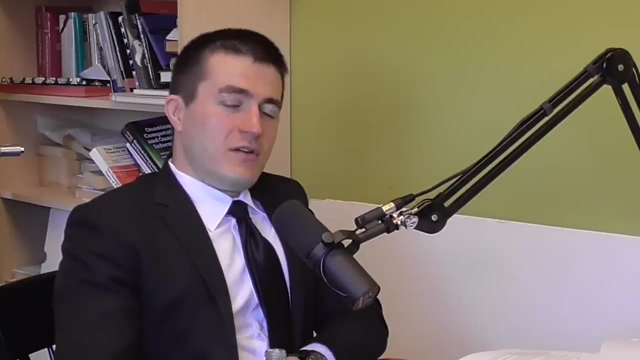 My favorite is the one called eternal inflation. The infinity can be on both sides, on one of the sides and none of the sides. So what's eternal infinity? Okay, Infinity on both sides. Oh boy, Yeah, yeah, Why is that your favorite? Because it's the most just, mind-blowing? No, Because we want a beginning. No, Why do we want a beginning? In practice, there was a beginning. of course, In practice there was a beginning, But could it have been a random fluctuation? 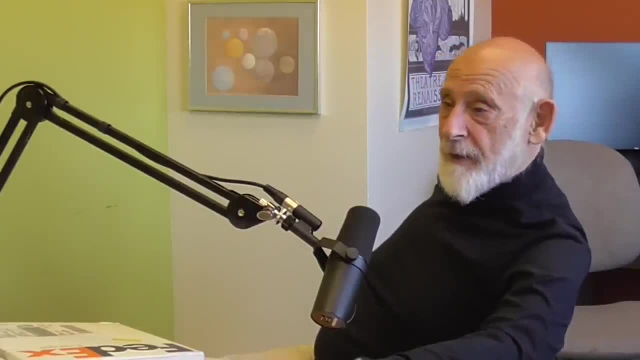 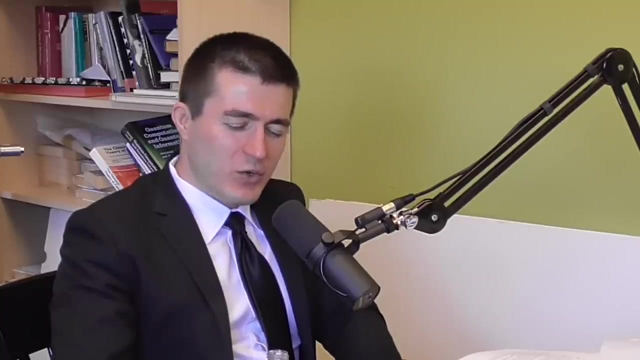 in an otherwise infinite time, Maybe. In any case, the eternal inflation theory, I think, if correctly understood, would be infinite in both directions. How do you think about infinity, Oh God? So okay, of course, you can think about it mathematically. 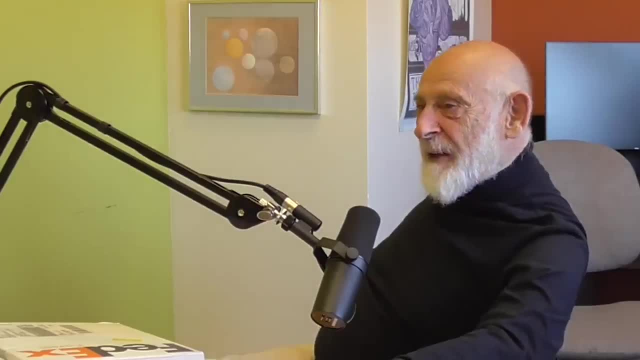 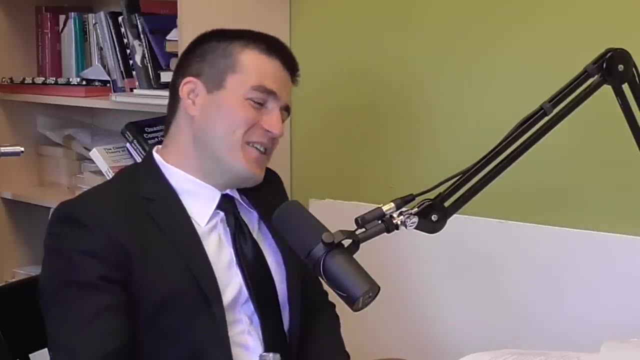 I just finished this discussion with my friend, Sergey Brin. Yes, How do you think about infinity? I say, well, Sergey Brin is infinitely rich. How do you test that hypothesis? Okay, That's such a good line, Right? 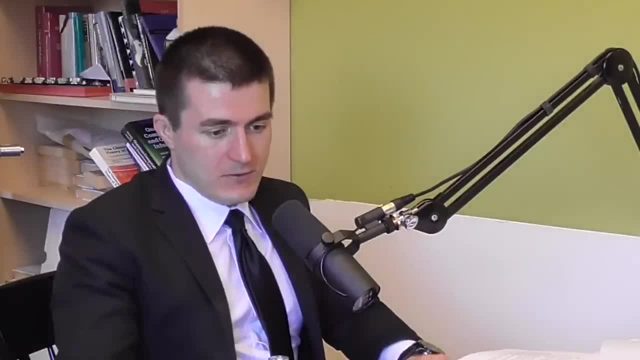 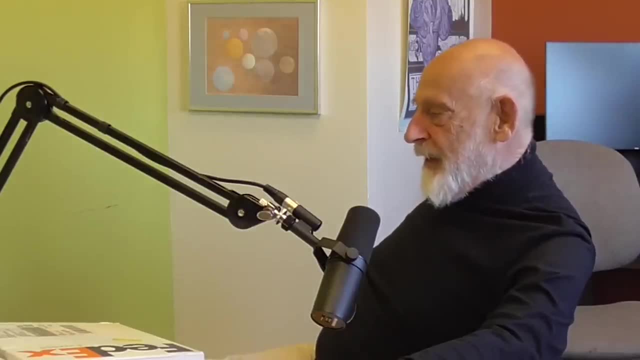 Yeah, so there's really no way to visualize some of these things. Yeah, No, this is a very good question. Does physics have any? does infinity have any place in physics? Right, Right, And all I can say is: very good question. 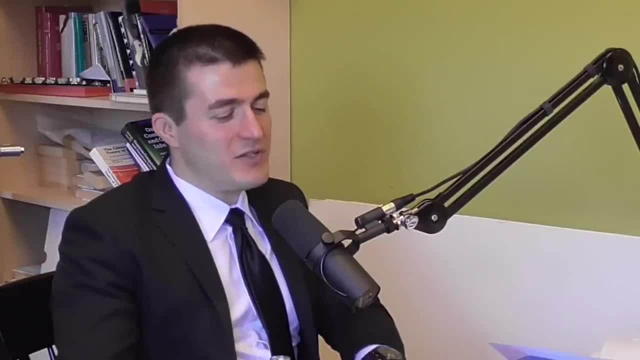 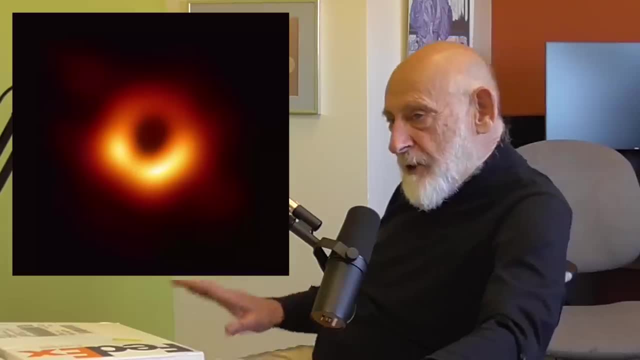 So what do you think of the recent first image of a black hole visualized from the Event Horizon Telescope? It's an incredible triumph of science In itself. the fact that there are black holes which collide is not a surprise, Right, And they seem to work. 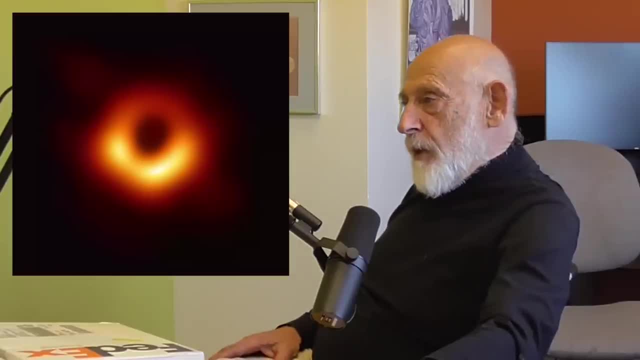 they seem to work exactly the way they're supposed to work. Will we learn a great deal from it? I don't know, I can't, I, I, I, we might, But the kind of things we'll learn won't really be about black holes. 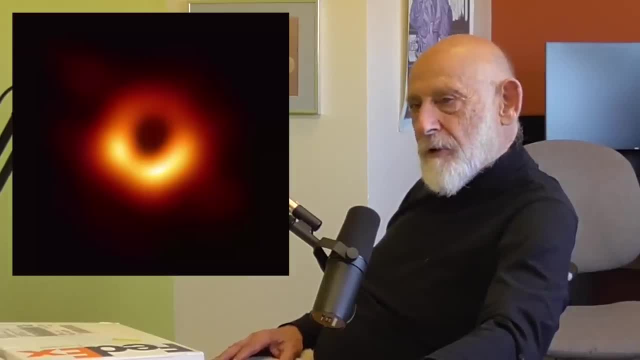 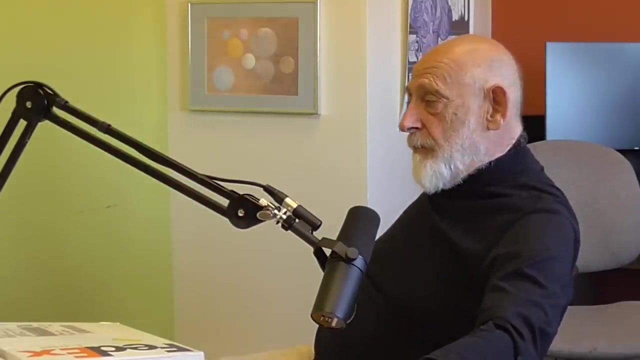 Why there are black holes in nature of that particular mass scale and why they're so common may tell us something about the structure evolution of structure in the universe, But I don't think it's going to tell us anything new about black holes. But it's a triumph in the sense that you go back a hundred years. 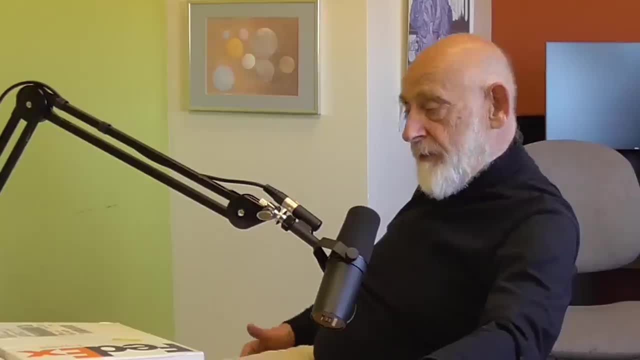 and it was a continuous development. general relativity, the discovery of black holes, LIGO, the incredible technology that went into LIGO. It is something that I never would have believed was going to happen, you know, 30,, 40 years ago. 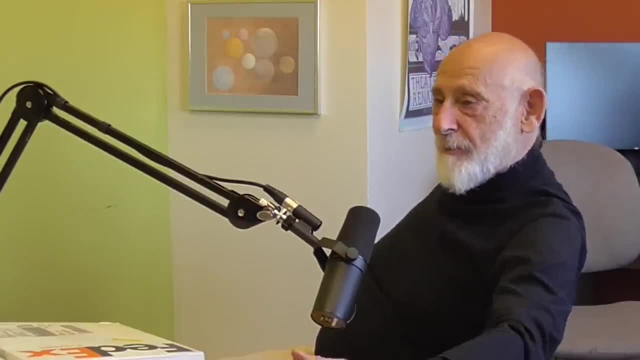 And I think it's a magnificent structure. It's a magnificent thing, This evolution of general relativity, LIGO, high precision, ability to measure things on a scale of 10 to the minus 21.. So, yeah, So you're just in awe. 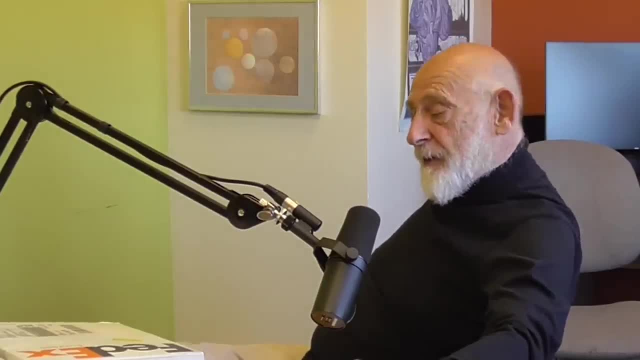 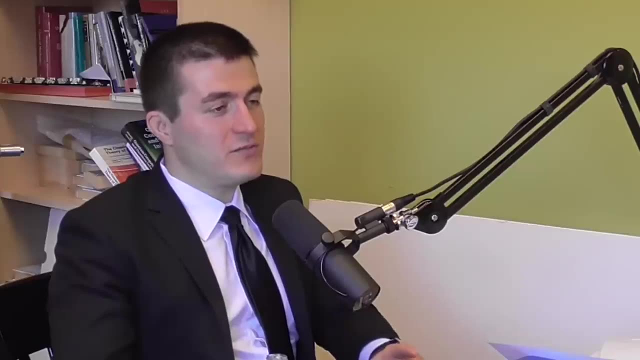 Astonishing, Just in awe. This path took us to this picture. Is it different? You know you've thought a lot about black holes, Is it? how did you visualize them in in your mind, And is the picture different than you realized it? 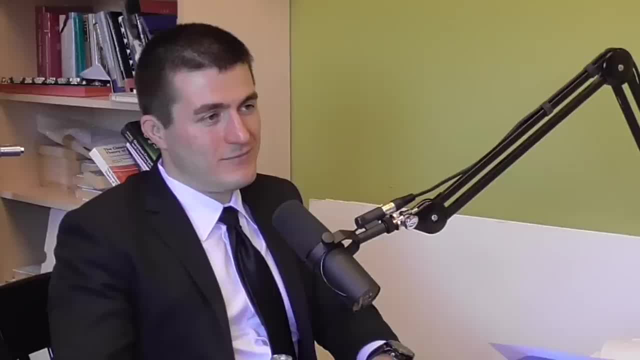 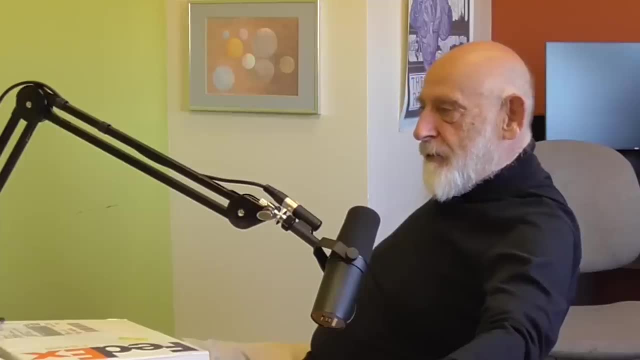 No, no, It simply confirmed. you know, it's a magnificent triumph to have confirmed, Confirmed, A direct observation. Yeah, That Einstein's theory of gravity at the level of black hole collisions actually works is awesome, It is really awesome. 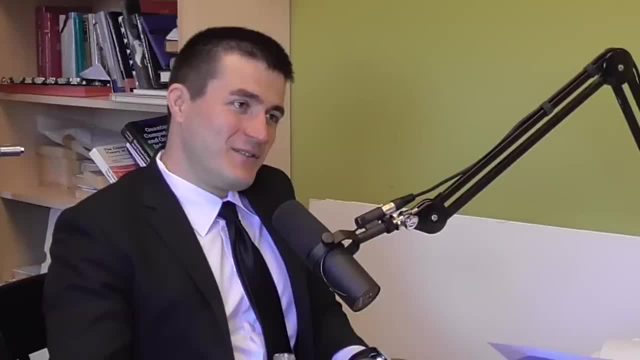 You know, I know some of the people who were involved in that. They're just ordinary people, Yeah, Yeah, And But the idea that they could carry this out, I, I, just, I'm shocked. Yeah, Just these little homo sapiens. 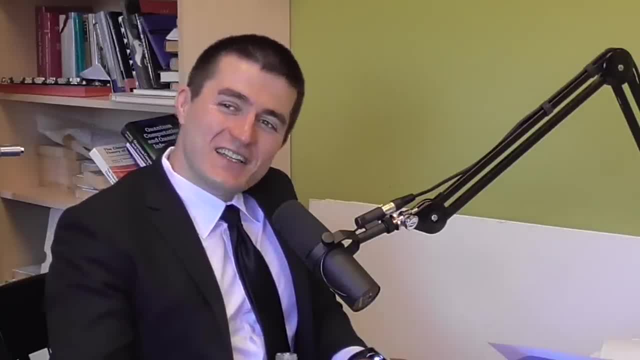 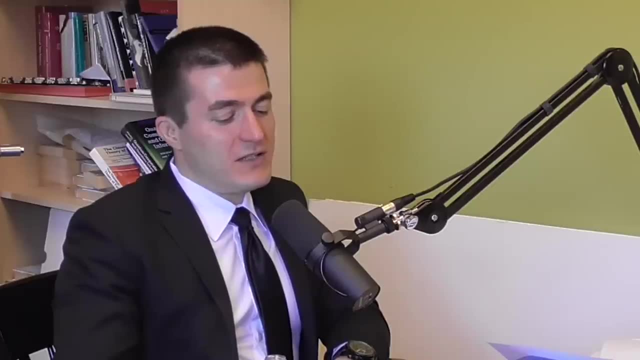 Yeah, Just these little uh monkeys got together and uh took a picture of uh slightly advanced limers, I think. What kind of questions can science not currently answer but you hope might be able to soon? Well, you, you've already addressed them. 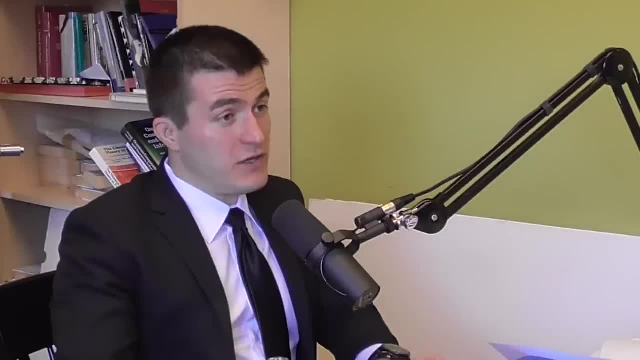 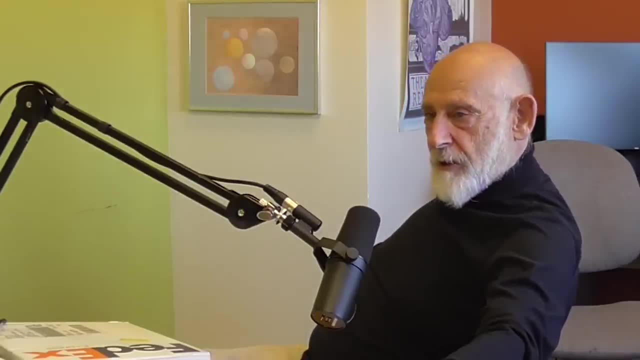 What is consciousness, For example? you think that's within the reach of science. I think it's somewhat within the reach of science, But I think now I think it's in the hands of the computer scientists and the neuroscientists, Not a physicist. 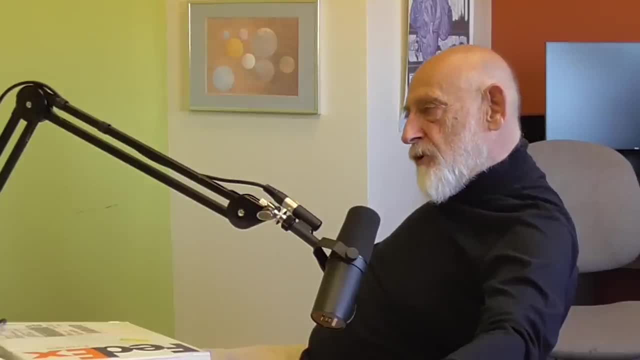 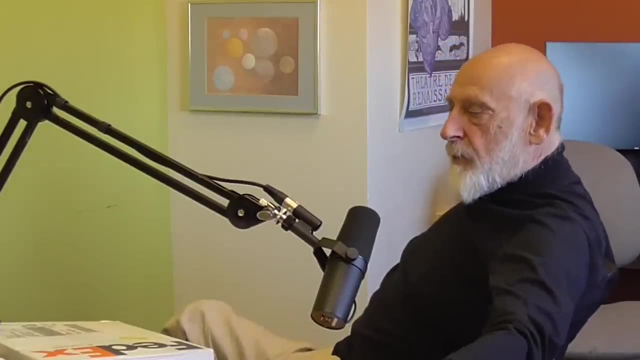 Perhaps Would that help, Perhaps at some point. but I think physicists will try to simplify it down to something that they can use their methods and maybe they're not appropriate. Maybe we, we, maybe we simply need to do more machine learning on bigger scales. 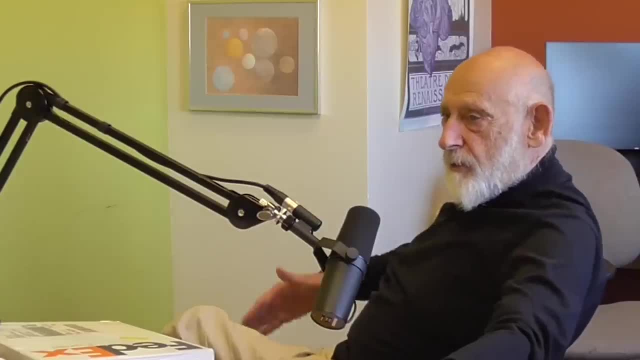 evolve machines. machines not only that learn, but evolve their own architecture. Yeah, As a process of learning, evolve an architecture, not under our control, only partially under our control, but under the control of a machine learning. Uh, I'll tell you another thing that I find awesome. 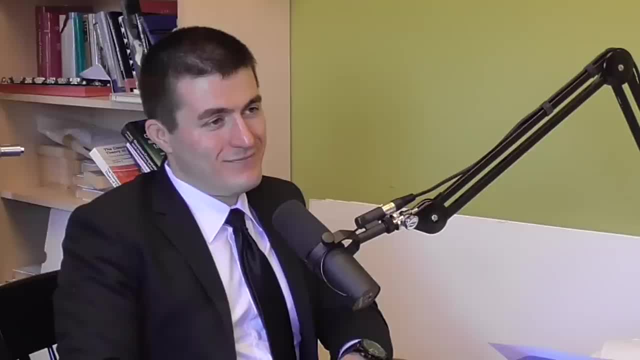 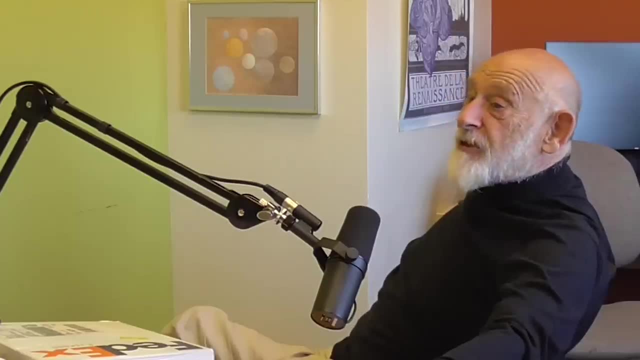 Uh, you know this Google thing that they taught, uh computers how to play chess. Yeah, Yeah, Okay, They taught computers how to play chess. not by teaching them how to play chess, but just having them play against each other. 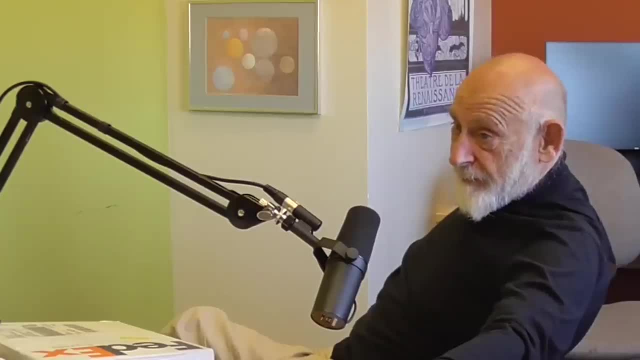 Against each other, Self play Against each other. This is a form of evolution. These machines evolved. They evolved an intelligence. They evolved an intelligence without anybody telling them how to do it. They were not engineered, They just played against each other and got better and better and better. 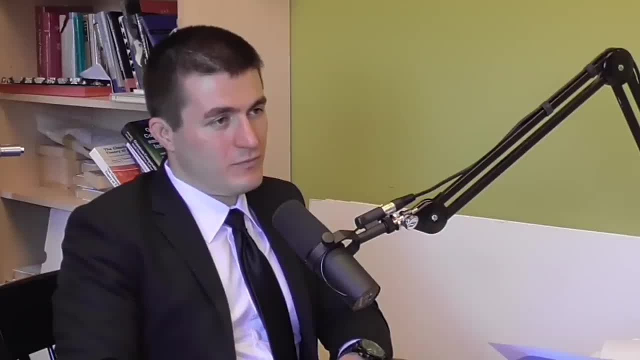 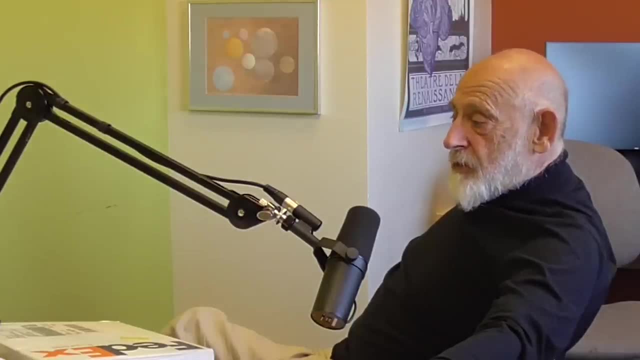 That makes me think that machines can evolve intelligence. What exact kind of intelligence, I don't know. but in understanding that, better and better, maybe we'll get better clues As to what goes on in our own intelligence. Well, life and intelligence is. 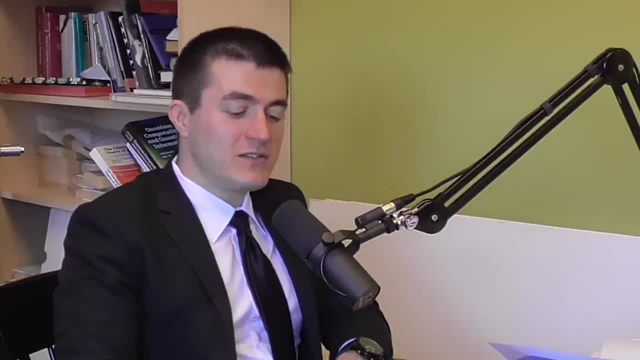 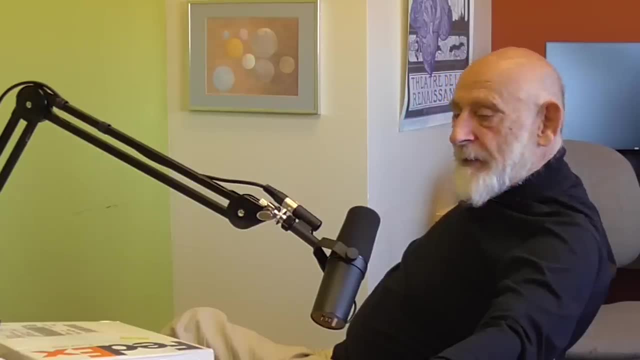 Yeah. Last question: What kind of questions can science not currently answer and may never be able to answer? Yeah, Is there an intelligence out there? that's underlies the whole thing. You can call them with a G word if you want. Uh, I can say uh, uh, are we a computer simulation with a purpose?